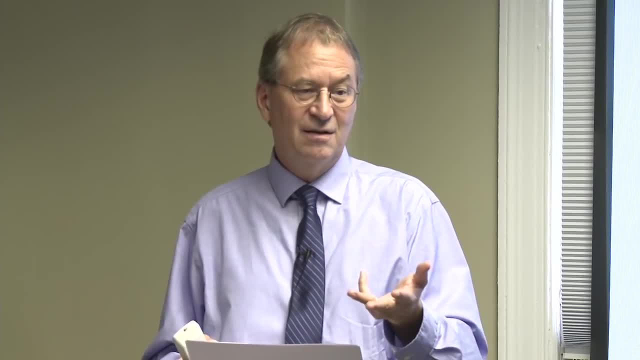 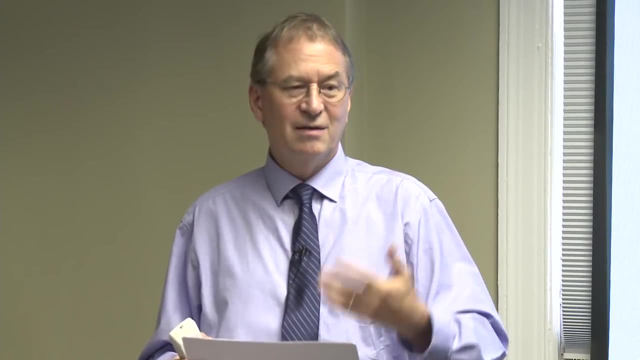 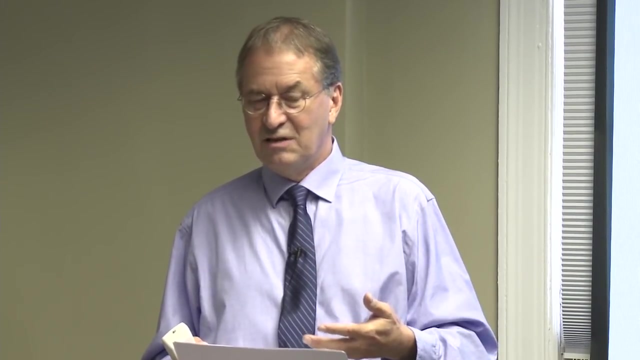 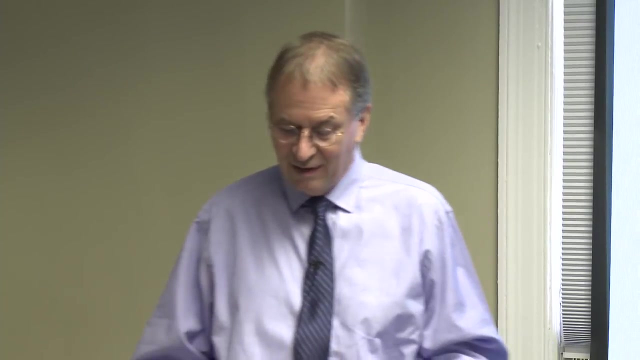 nuclear weapons. That includes India, Pakistan and Israel. Technically they're non-nuclear weapon states because they didn't test a nuclear weapon. It also includes signatories to the NPT that have sought nuclear weapons. We bring disarmament into that discussion. Some of the lectures will cover that, In fact, one part of today. 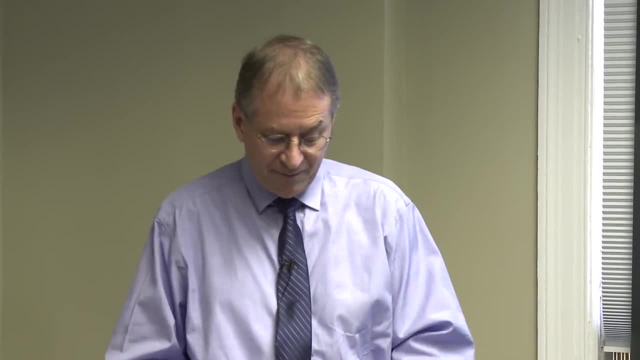 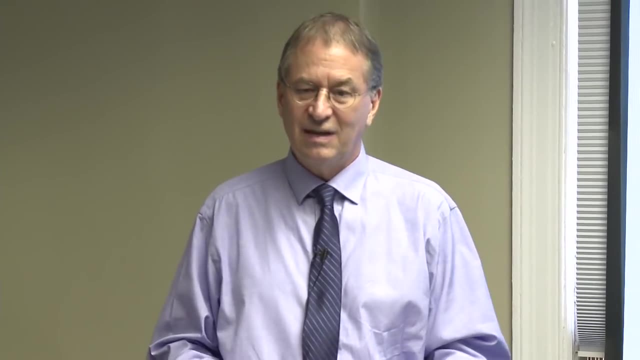 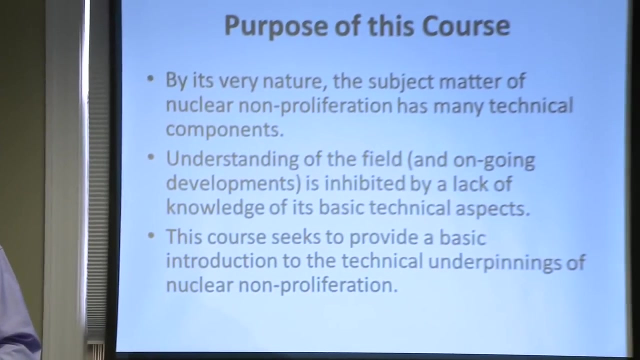 I'll look at the South African case I mentioned. it's a technical field. It's very hard to understand it without understanding the technical side of this. We're going to try to provide some basics on that. Later courses we'll get into. 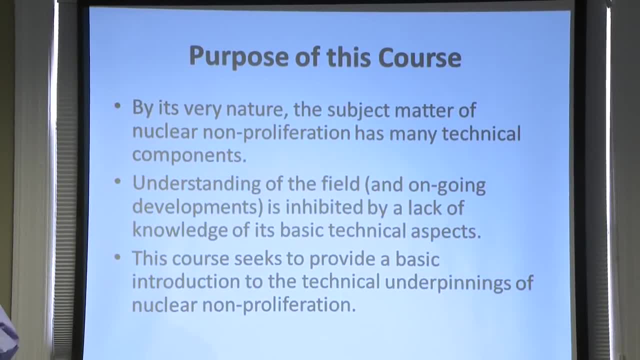 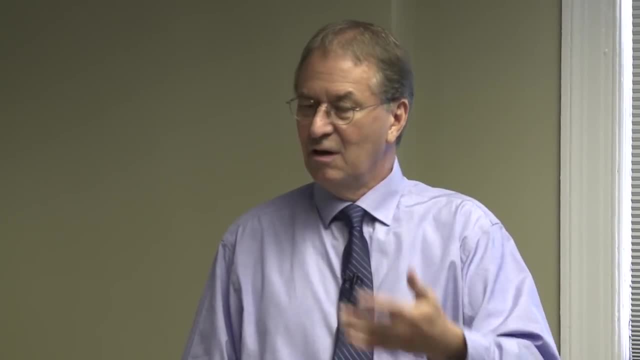 other topics, I think one we've decided to do in the winter is we'll do a survey of the Iran nuclear program from a technical point of view to really understand all you need to know about the Iran nuclear program relevant to any agreement that's reached. 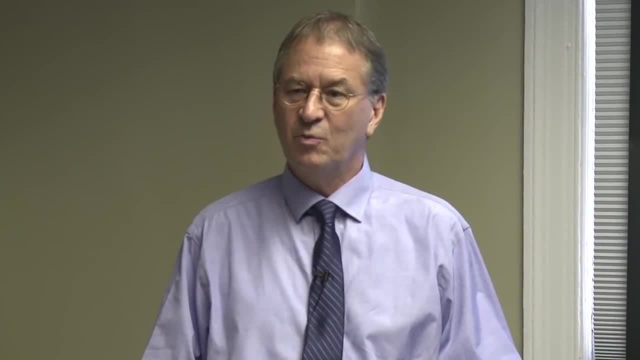 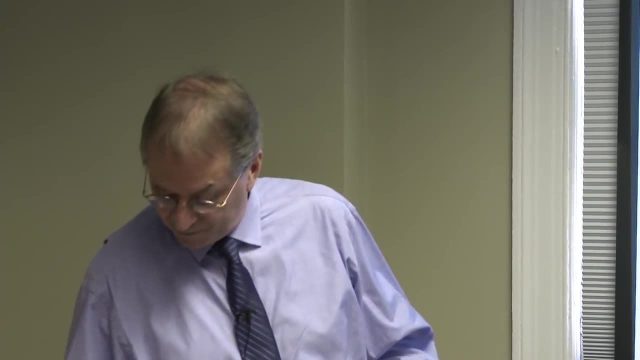 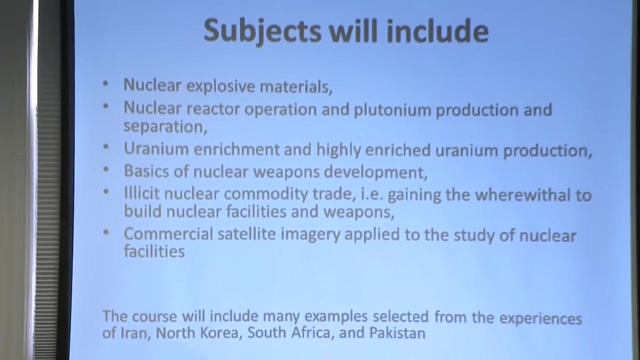 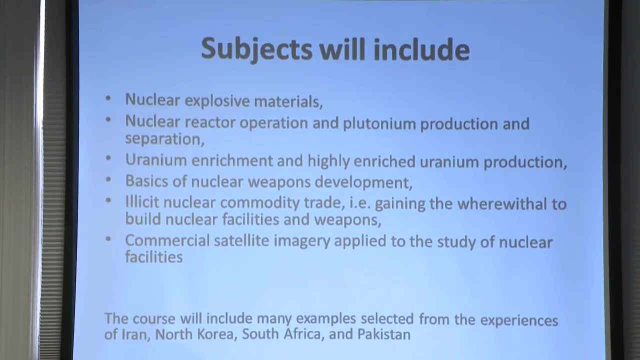 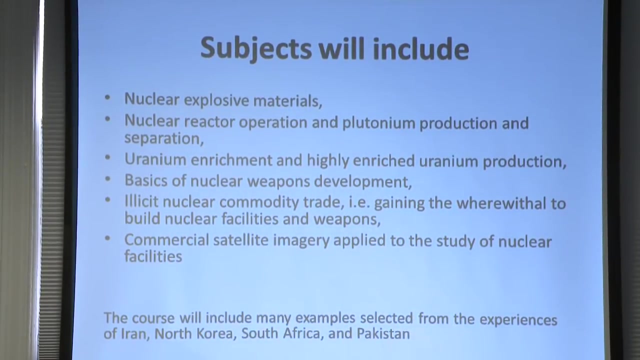 or not reached all the discussions of the diplomacy. What's what In this course? we have ten weeks. We're going to cover quite a bit from nuclear explosive materials. We'll get into how reactors operate and plutonium is produced and separated. We'll do a lot on uranium enrichment. We'll touch upon the basics of nuclear weapons. 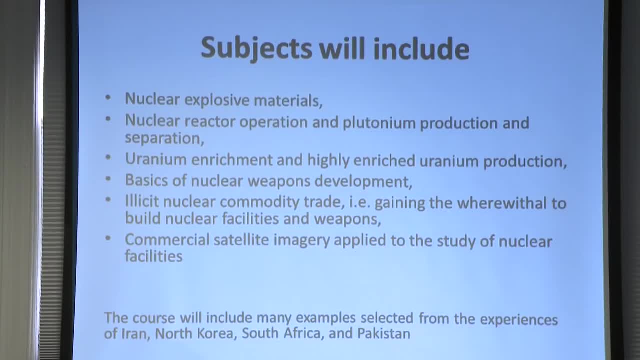 development. Much will just depend on how much time we have. It's one of the more sensitive topics, and one of the ways we deal with this is by avoiding the discussion. Today I'll give a lecture that will touch upon several aspects of nuclear weapons development. If there's 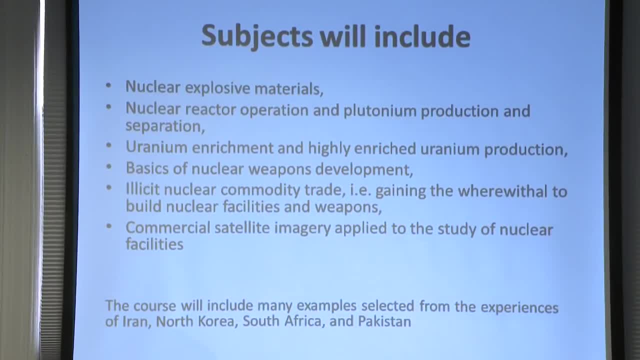 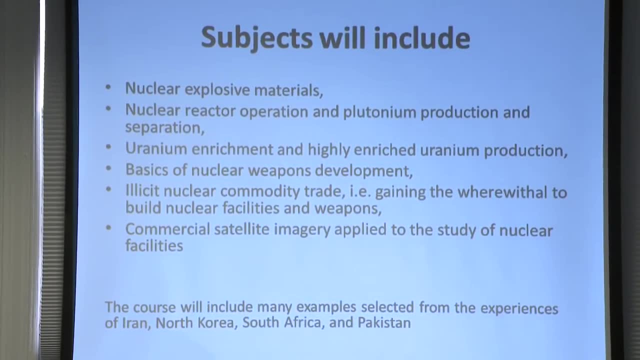 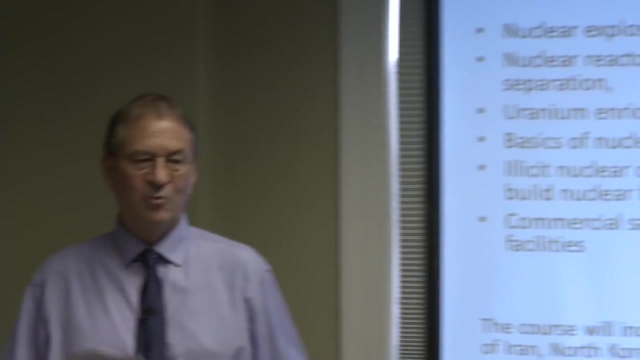 another lecture, it will just depend on time. We'll also cover some specialized area: elicit, nuclear commodity procurements, how countries get the wherewithal to build nuclear weapons. These countries that we study don't have great industrial bases so they have to go out and buy a considerable amount to put together. 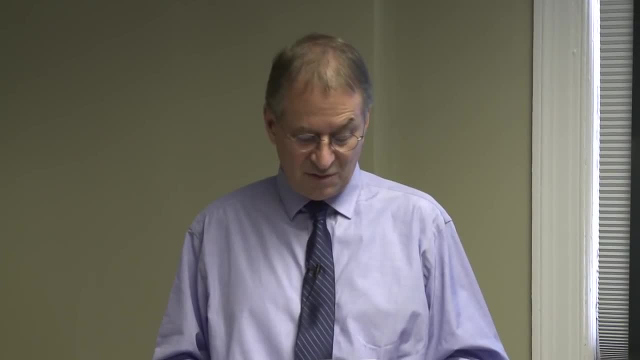 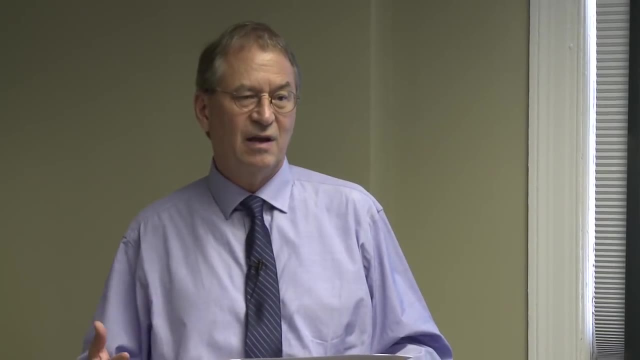 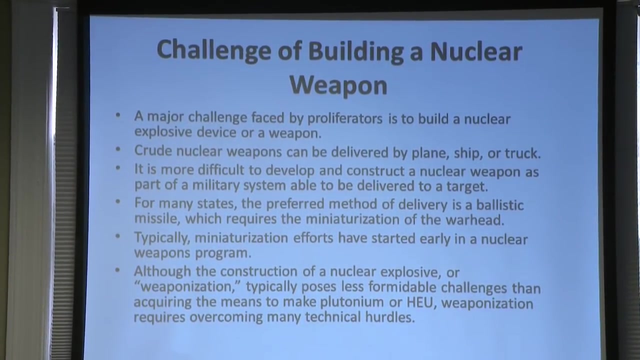 the facilities to make nuclear explosive materials. Then we'll also spend time trying to use commercial satellite imagery as applied to nonproliferation. It's often said that it's easy to build a nuclear weapon. I mean separate from getting the nuclear explosive material. but if you go to the Internet, you talk to people, they'll 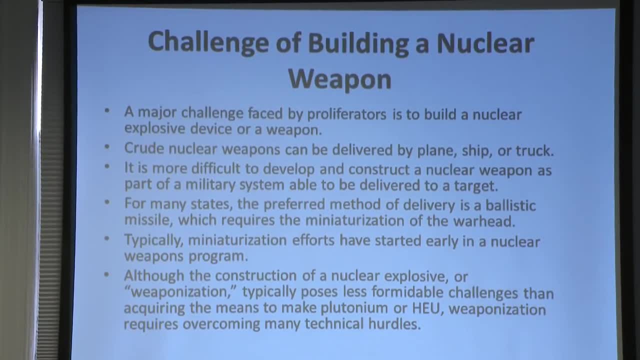 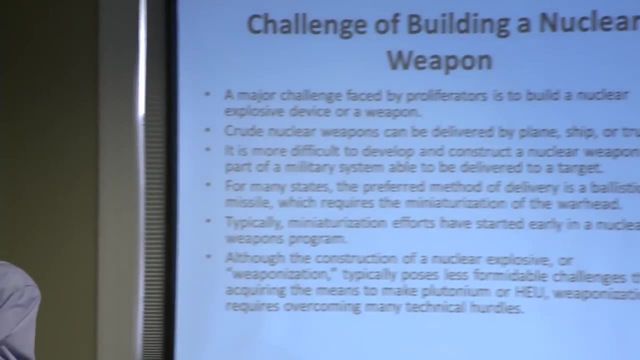 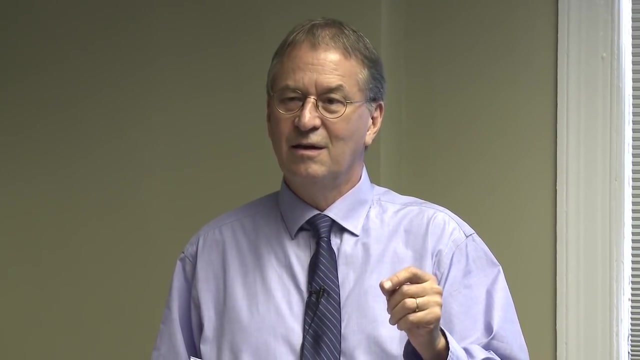 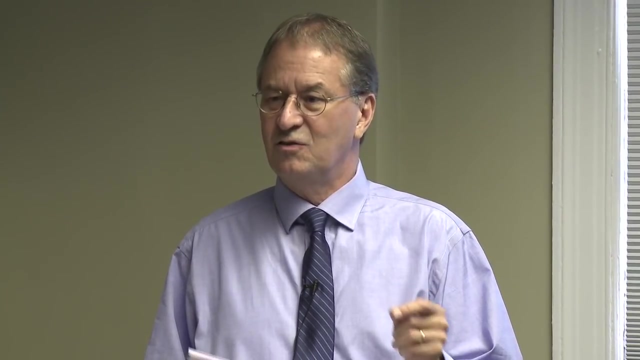 say it's an easy thing to do If you look at countries building them- India, Pakistan. be careful on Iran. but we will talk about the information about Iran's nuclear weapons program. At least we'll touch upon that. It's IA information and it's available. But they have problems. It's not as easy to. do. There's a lot of challenges. even to build a crude nuclear explosive. I'll admit it's not as hard as building a uranium enrichment plant to produce highly enriched uranium, or reactor and chemical processing plant to create separated plutonium, but it has its own challenges. 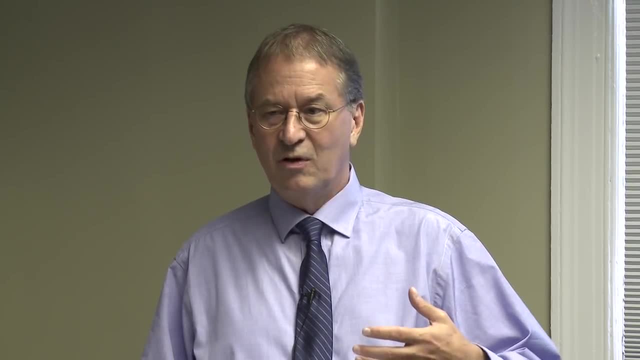 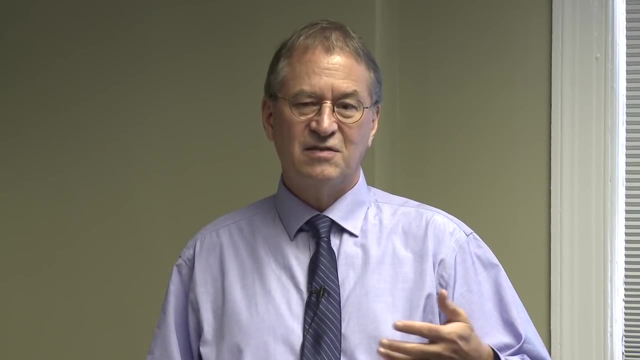 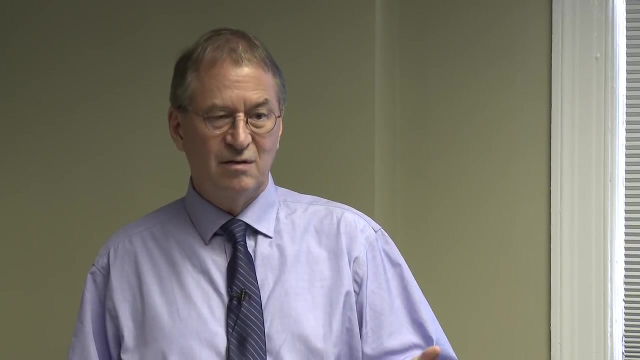 If you want to put that nuclear weapon on a delivery system, there's new challenges. It's a military system. It has to meet criteria of reliability, safety, security and military standards. That can be extremely challenging If you want to put it on a ballistic missile. 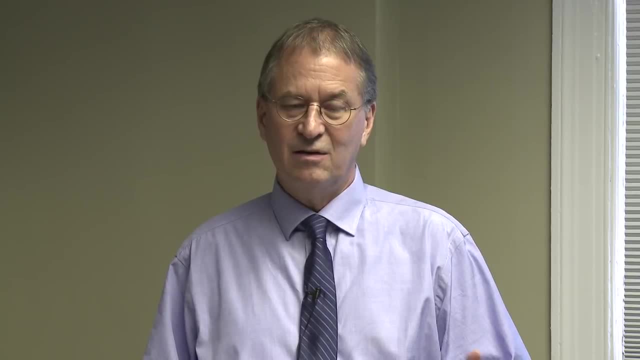 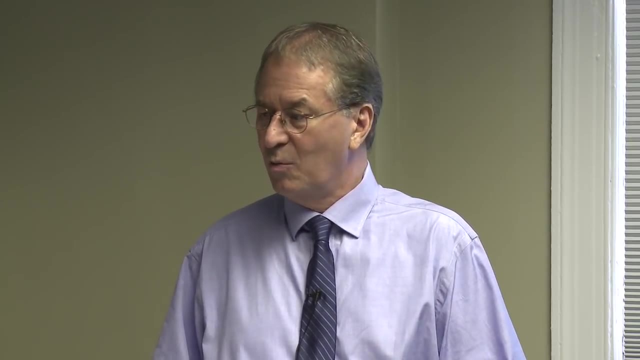 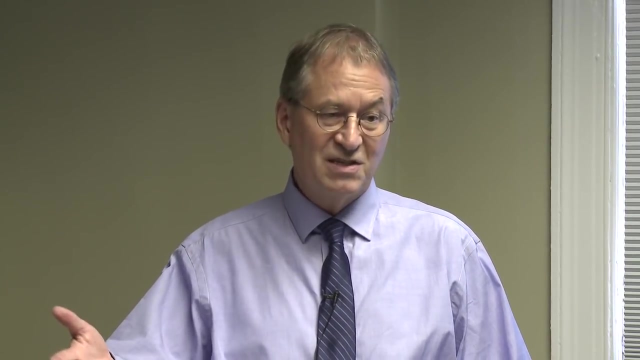 you have to worry about miniaturizing it. That creates additional problems that have to be overcome. Now, all the states that go about this will overcome these problems, but how long it takes it depends on their skills and also their outside help. In many cases, it's been the 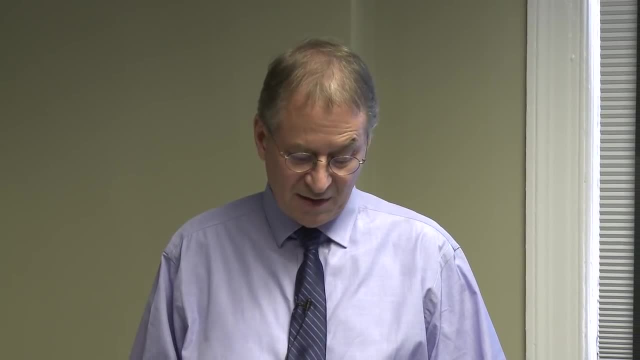 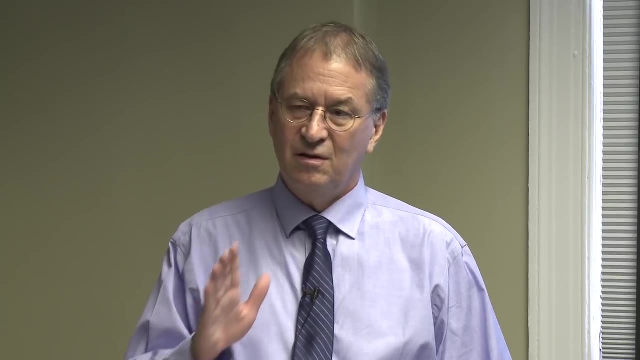 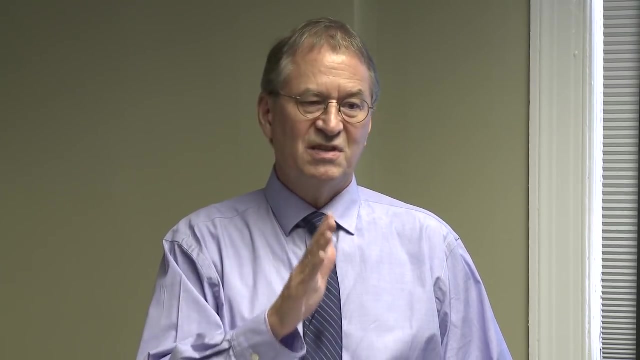 outside help. that has been critical to speeding up the process. Also, one thing I want to emphasize is you have to get the nuclear explosive material. You have to learn how to- we call it- weaponize it. Those things tend to happen in parallel. 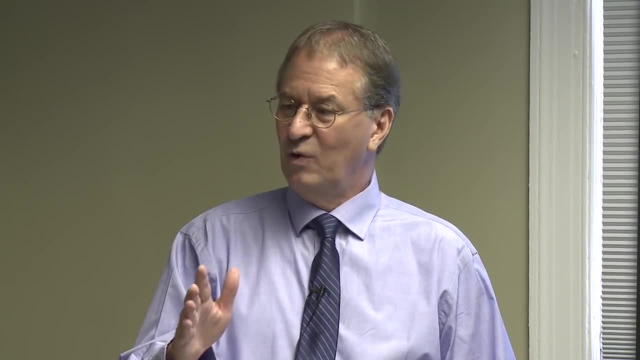 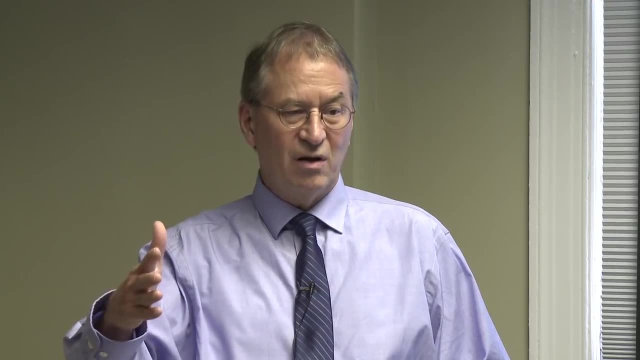 It's not as if the state- okay, now we're going to concentrate on this, We're going to wait to get plutonium. and then they get it and they think, oh, now we need to think about how to make a weapon. They typically run in parallel. Sometimes the state gets. 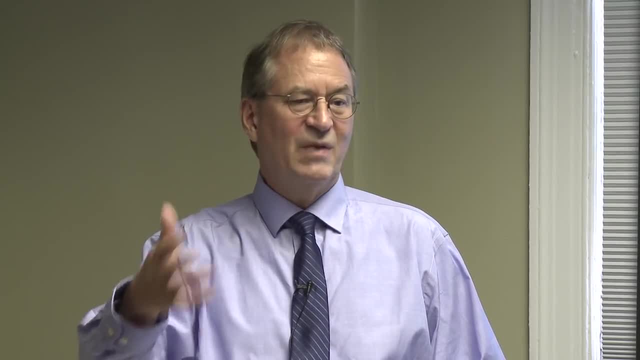 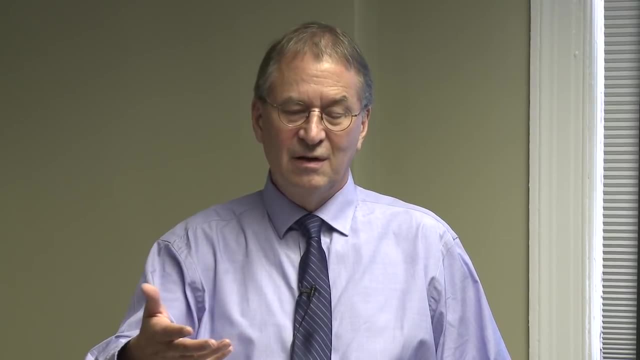 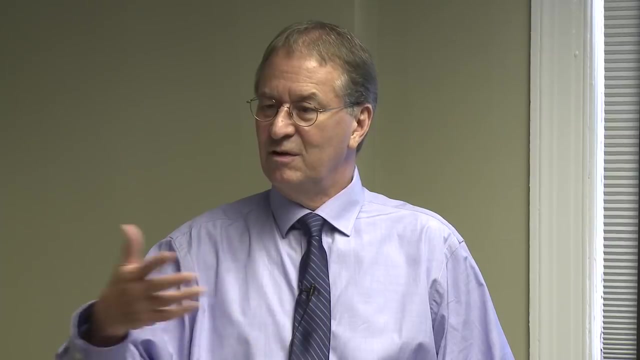 the fissile material and it doesn't take them that long to be able to weaponize it. Also, there's different ways of weaponizing it, If you think through the Iranian problem, in a sense, if they broke out either secretly, 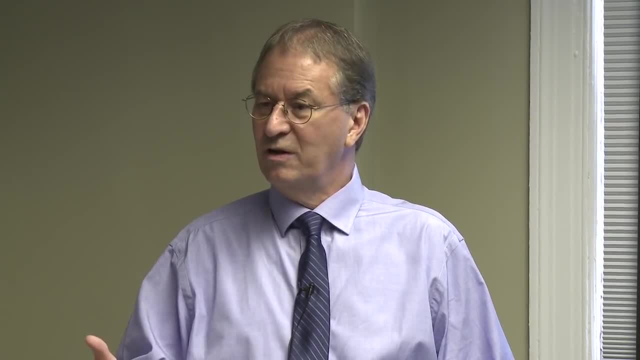 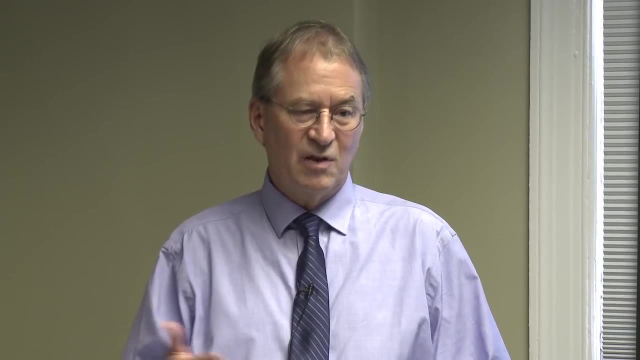 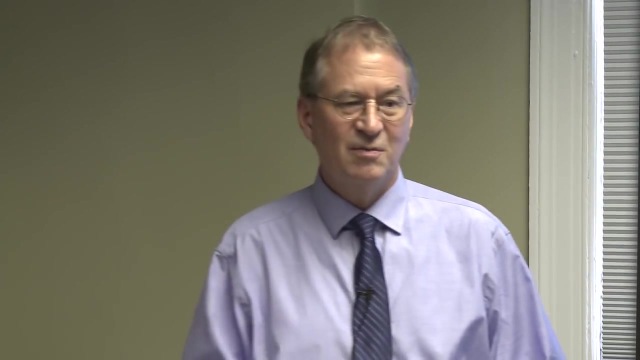 or overtly got highly enriched geranium in sufficient quantity for a bomb. what can they do with it? They could build a weapon that we don't even know about in some period of time. That weapon may never be intended for delivery, except maybe in some kind of odd emergency by ship. 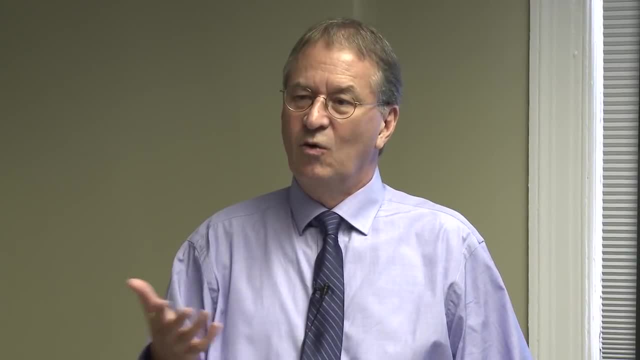 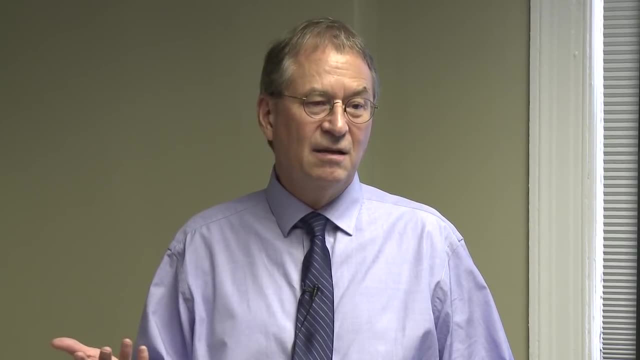 or truck. It could also end up being a way to say to the outside world: if you invade us, we'll use it. Well, how would they use it? In a sense, it would be like an Iranian IED would be a nuclear weapon. If anyone invaded them, then they would just have to emplace these nuclear weapons where the troops come through and then detonate them Even early after, only when they could make a crude weapon. they would actually create some kind of deterrence against a military. 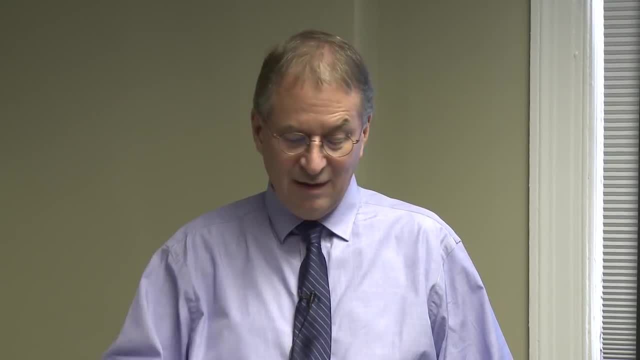 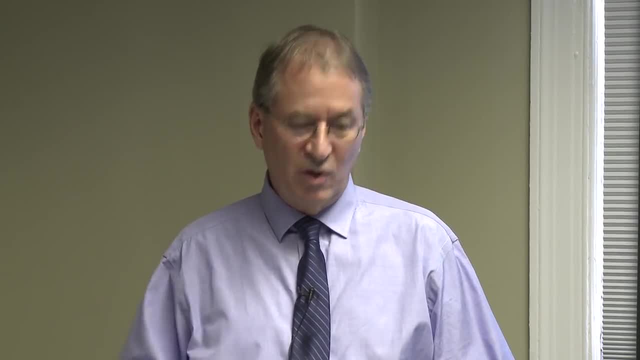 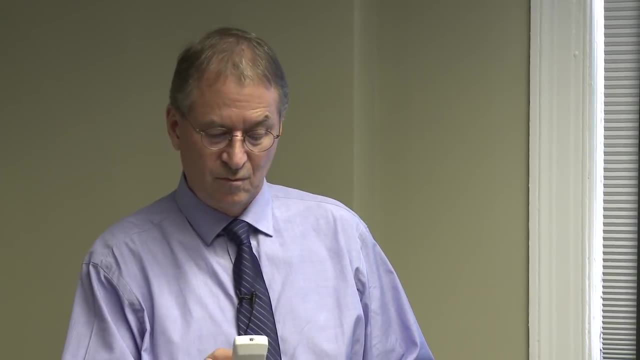 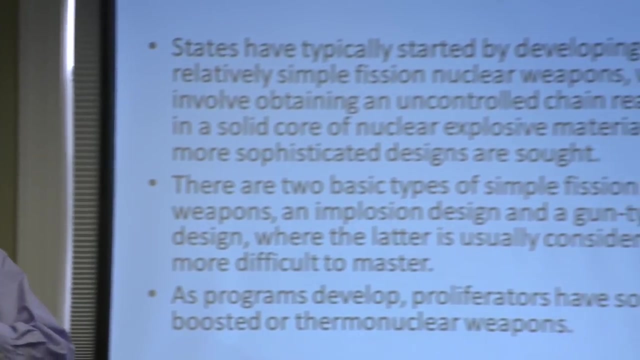 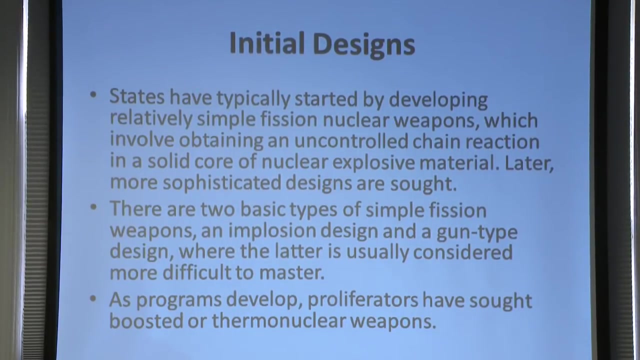 They would ultimately think of putting it on a ballistic missile, and that could very well be challenging. There's nothing surprising about the development of a nuclear weapon. If you're going to do it, you're going to start with a simple design, Unless someone hands you a design of an advanced 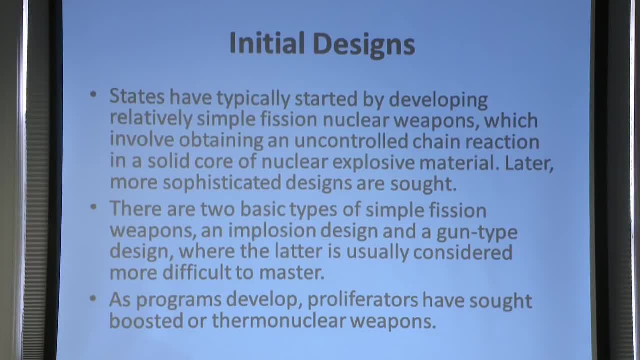 weapon and the help to master it. Getting to a separate weapon is not going to do you. Detailed design isn't going to be enough. typically in this area You're going to need additional, in a sense, human help. But typically the pattern has been to start simple and then work from there. 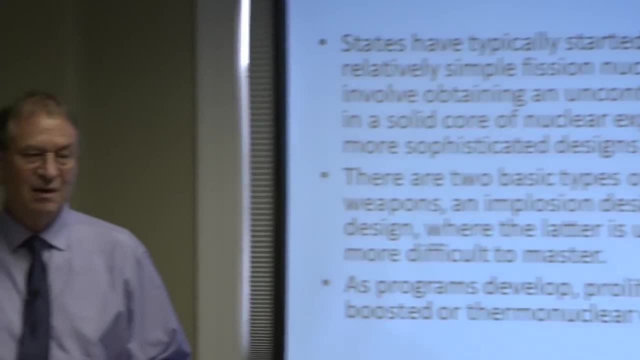 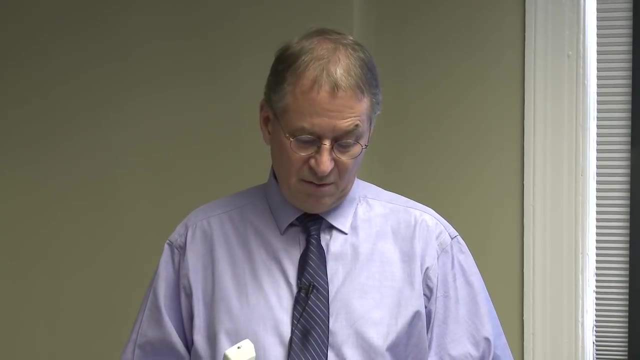 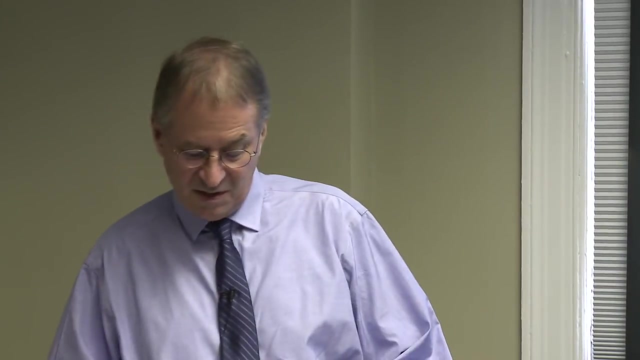 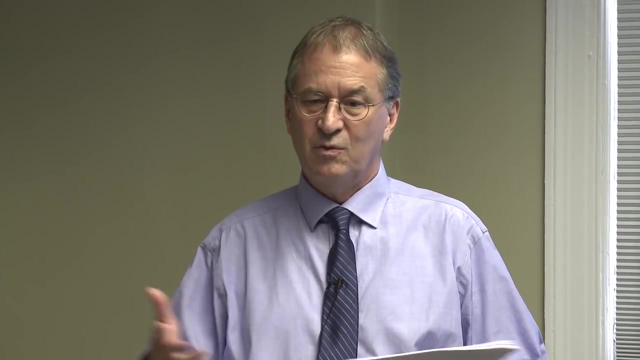 Most of what we study are crude fission weapons of two types: implosion type and gun type. The implosion type is where the former is usually considered more difficult to master. Then, as programs develop, they'll get into more advanced weapons. We won't talk about it today, but hopefully later boosted weapons. 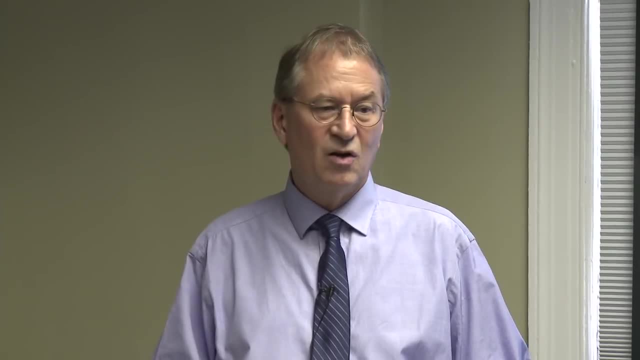 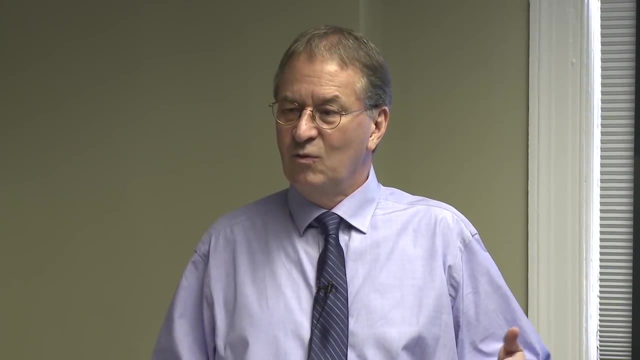 You all know what an H-bomb is. That would be a goal We worry. India is building H-bombs. now We have evidence that North Korea is working. We're looking to separate a thermonuclear material, tritium, from a certain process. 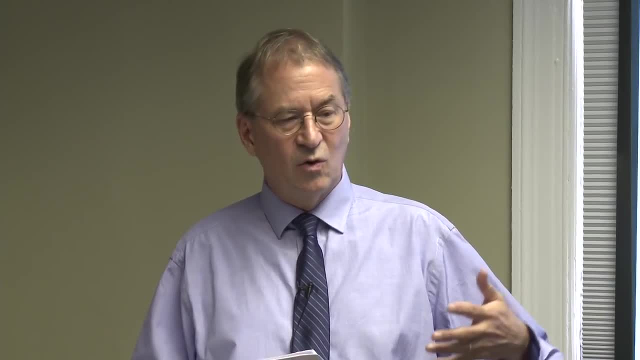 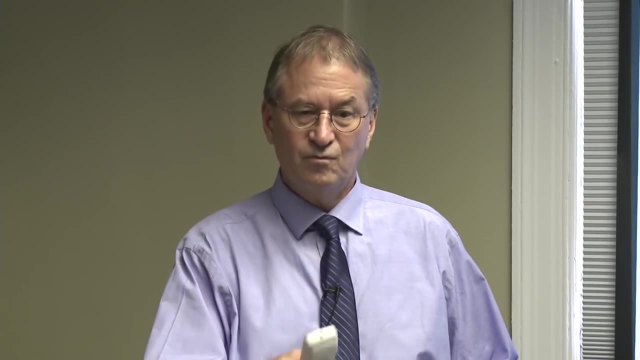 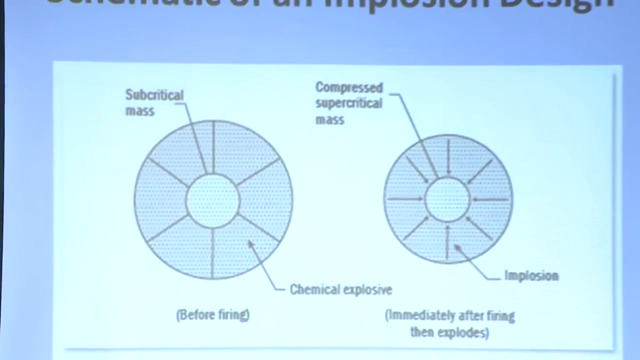 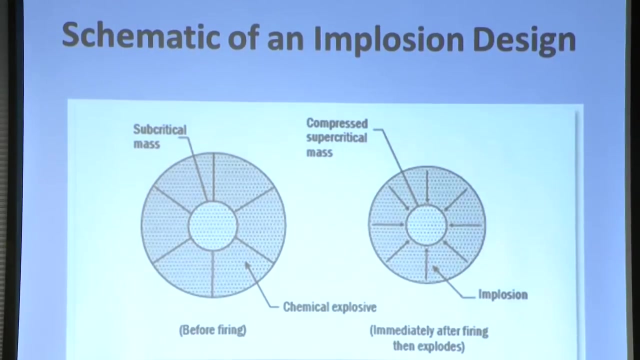 that we know it's working on. We're worried that North Korea is exploring more advanced nuclear weapons designs. Here's a very crude schematic of an implosion design. The idea of an implosion design is based on the fact that if you want to make a nuclear 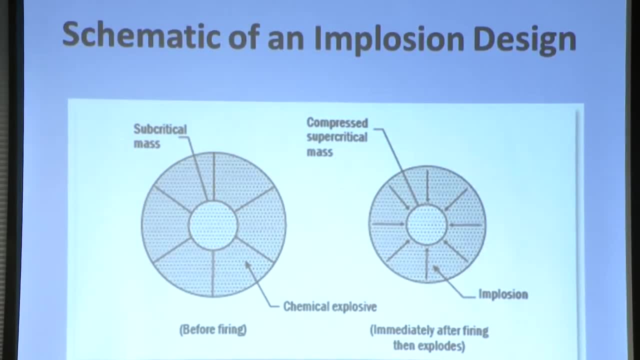 weapon, you're going to have to have something go what's called supercritical, which I'll talk about next week when I talk about nuclear explosive material Here. in a practical way, what you have to do is just find a way to take a piece of metal—could. 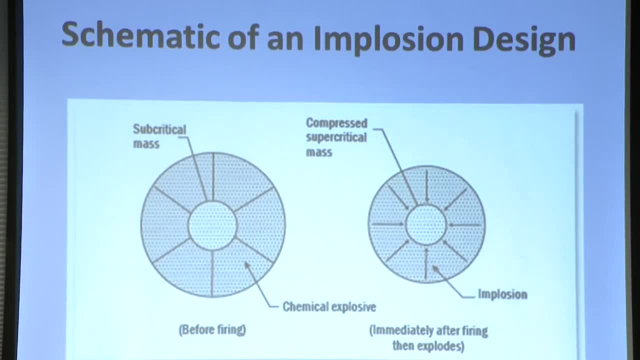 be just some X kilograms of plutonium or weapon-grade uranium—and squeeze it, It could actually change in diameter by a centimeter. Think about that. How do you take a piece of metal? How do you take a piece of metal? How do you take a piece of metal? 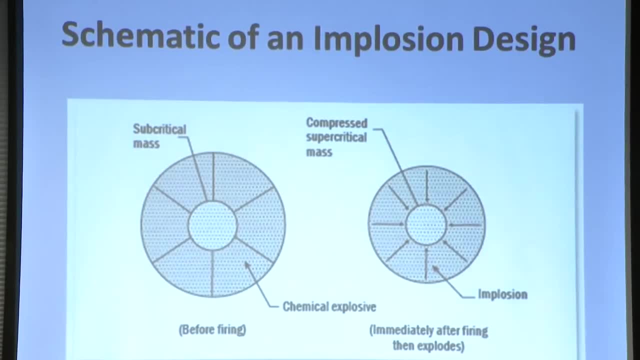 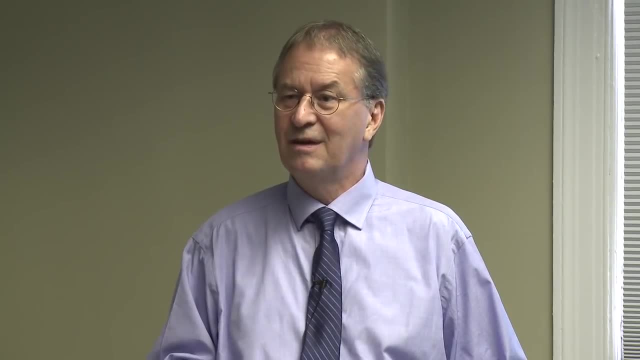 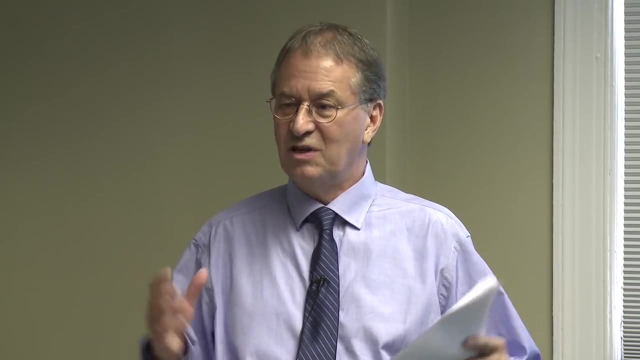 And then you don't get the compression. So it's really an art to figure out how to compress this thing uniformly so that you actually get this shrinkage in diameter which causes this increase in density, And that's what makes it super critical. 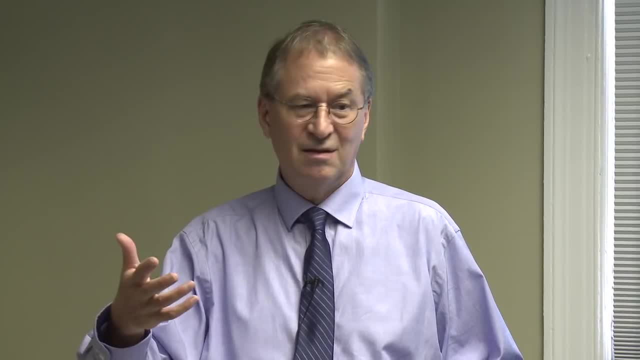 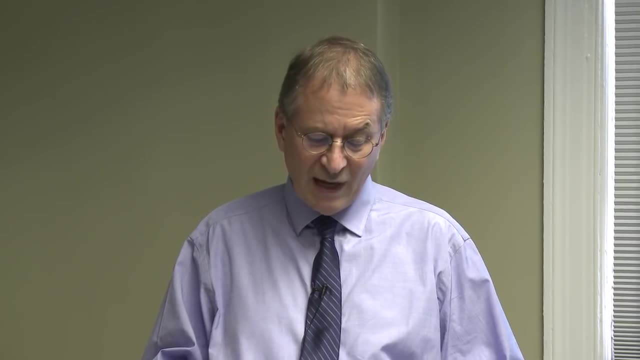 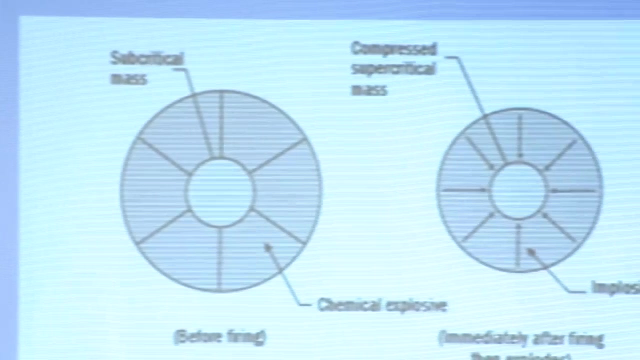 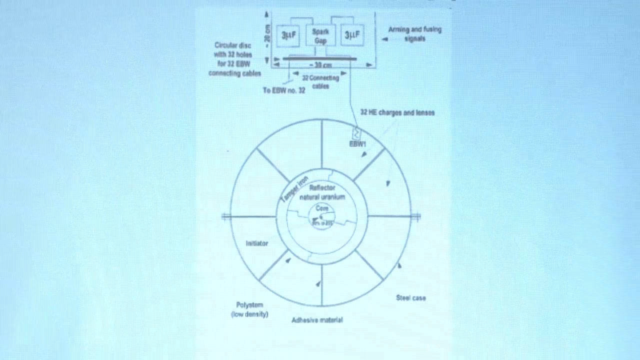 And so you're aiming, in an ideal world, to double the density through this shrinkage of the nuclear explosive material, And this diagram on the left shows it before, And then on the right it shows the mass smaller. Yeah, the next slide is from the Iraqi full, final and complete declaration from the 80s. 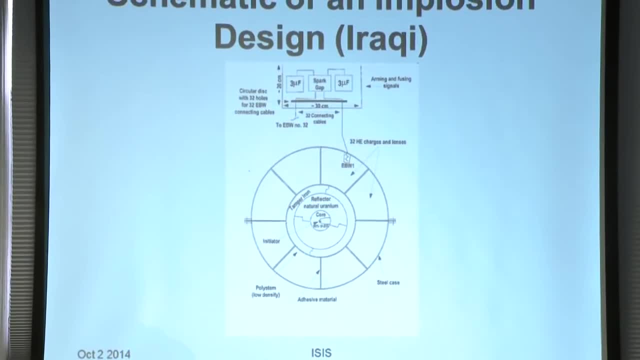 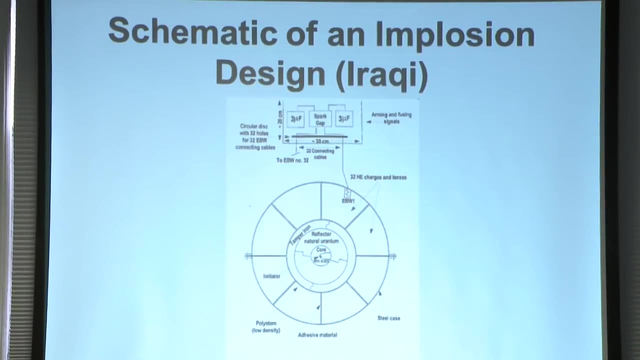 and just shows a little more detail of an implosion system. It's unclassified, but it just adds a little more detail where you need some fast-acting electronics And in this case they were using a spark gap. Well, I won't get into that at this lecture. 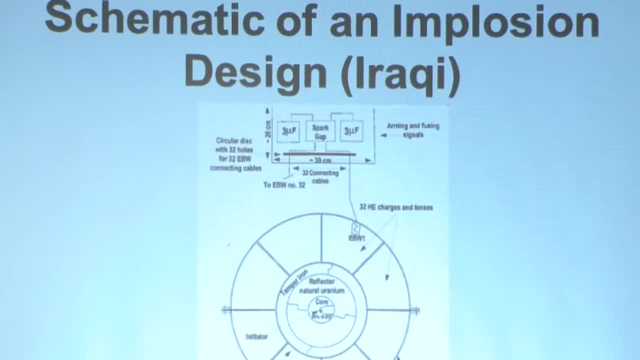 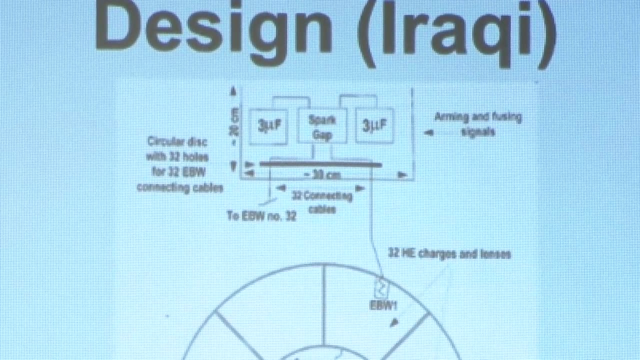 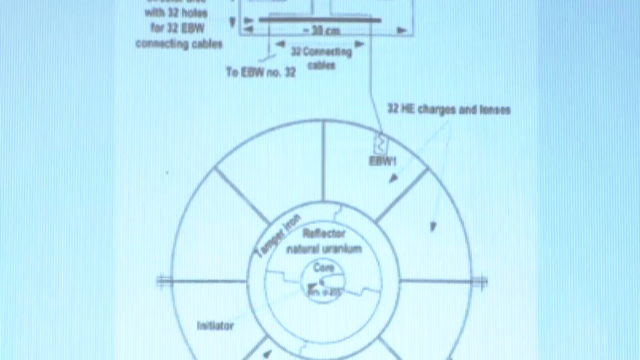 But in order to make this thing compress spherically, the high explosives have to be set off around this sphere of high explosive very precisely, And so you need a system to essentially send an electrical signal that then gets transmitted to points on the sphere essentially simultaneously. 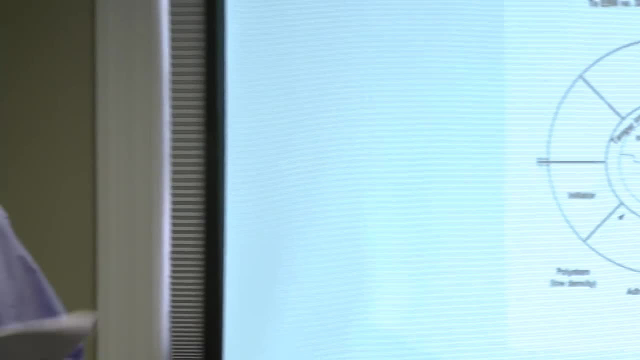 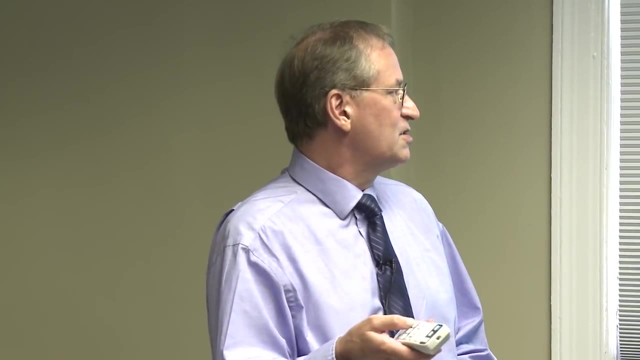 And then that creates- if the high explosives are done right, it creates a spherical shock wave. But I'll leave that to you to look at if you're interested. Here's just a picture. This is either Trinity or Nagasaki, I'm not sure. 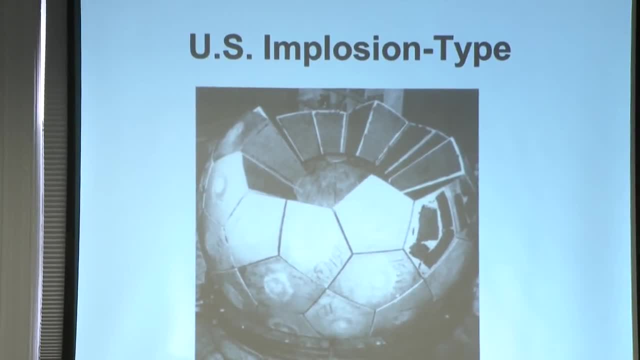 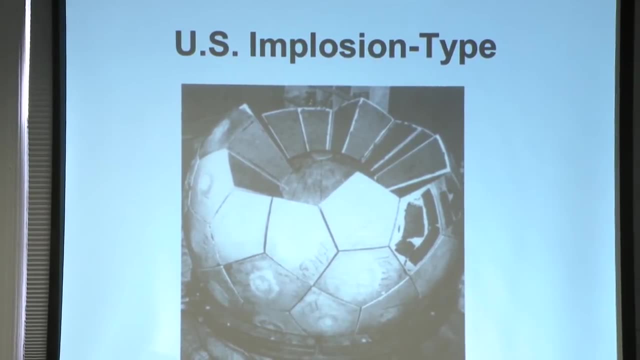 But it's an old US design, very large. You can see the shape charges. There's a core. It's not the plutonium. I mean. the core has several things in it and we'll talk about that another time. This is from an Iraqi declaration. 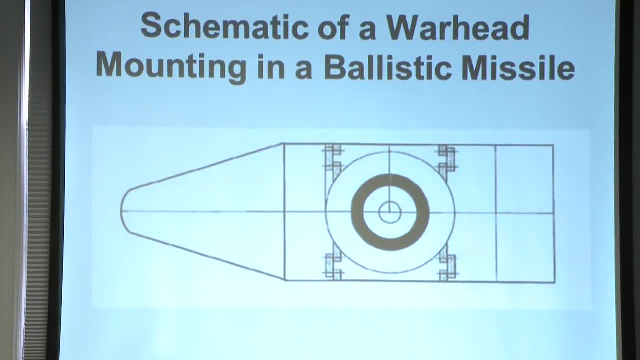 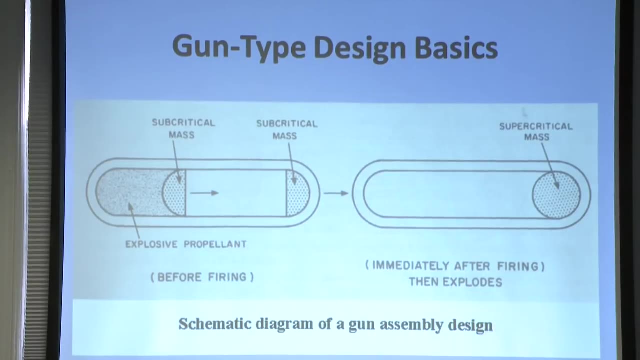 It's showing They're attempting to thinking through in a very primitive way how you would mount a warhead inside a ballistic missile reentry vehicle. The other type is a gun type And this one is conceptually a lot simpler. It literally, if you have enough mass of nuclear explosive material, if you can assemble it. 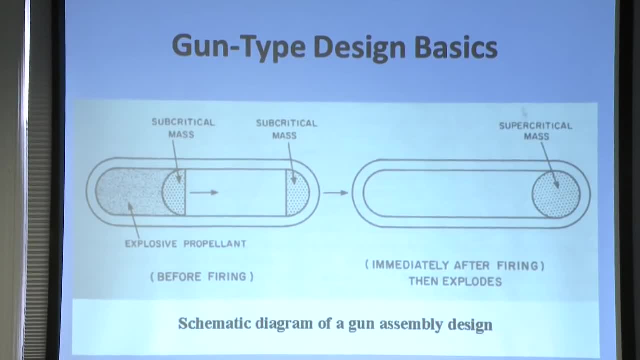 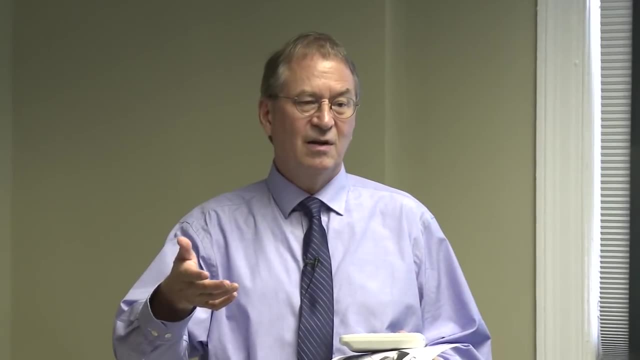 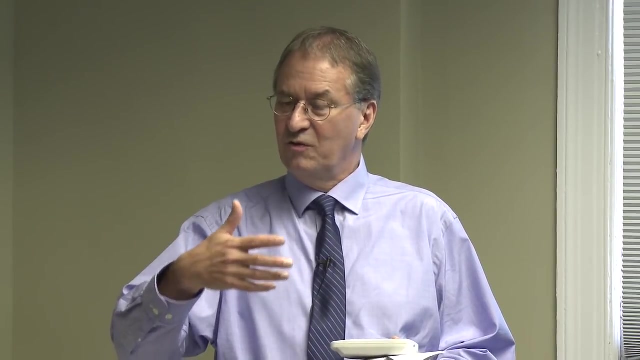 together it'll be super critical. And a rule of thumb is: if you have twice- I talked about doubling the density- well, if you have twice the amount of material, that's enough to make it go critical, which is have a self-sustaining chain reaction again. I'll cover this next week. 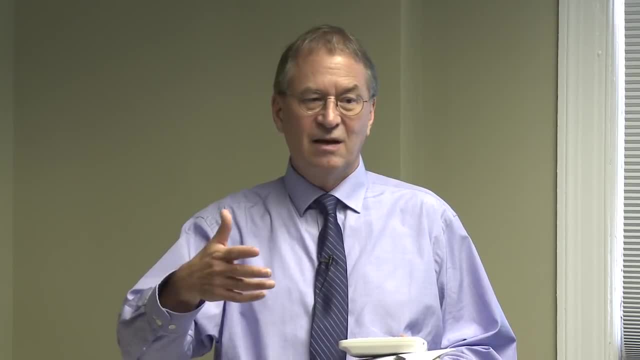 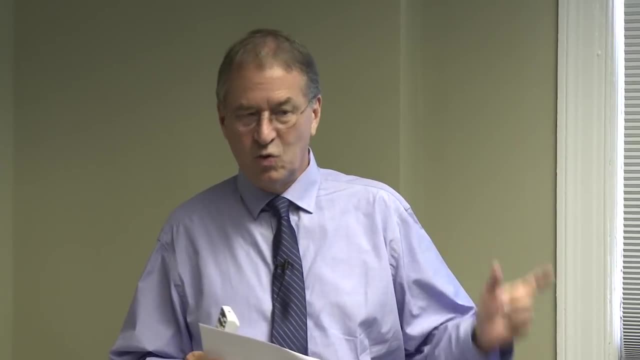 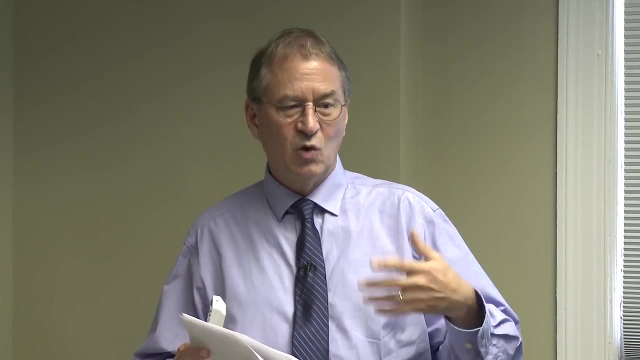 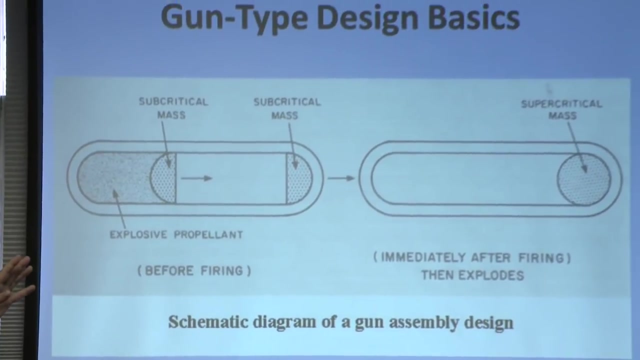 But if you double the amount of what causes criticality, then that'll be super critical, And so there's some problems that require you to do this quickly, and so the idea was: get a naval gun, Cut it down, Put most of the- in this case, they put half of the highly enriched geranium at one end. 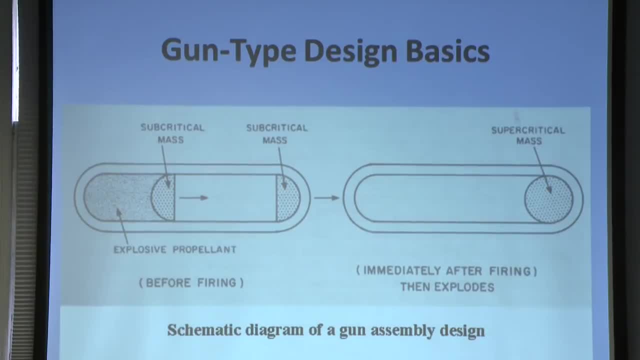 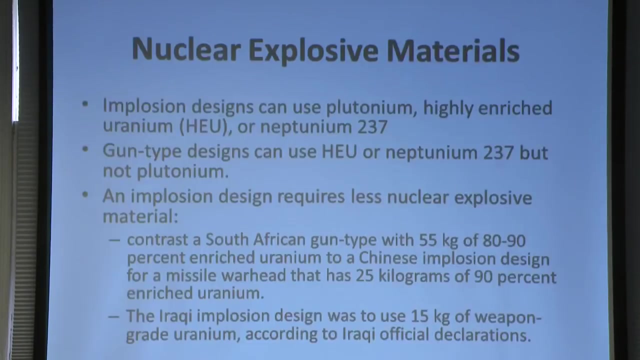 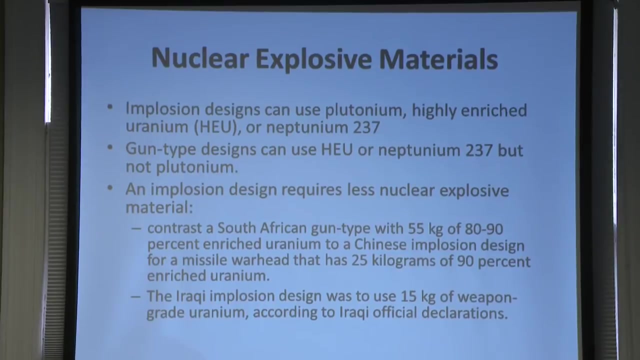 fixed and then shoot the other end down at it and when they combined you'll have enough for a nuclear explosion. And that was Hiroshima essentially. And let me just summarize what I've been talking about on the nuclear explosive material. 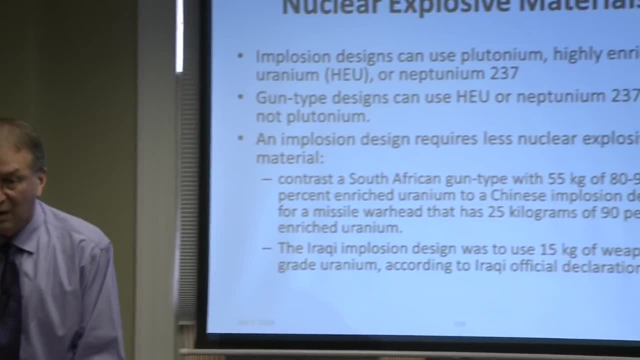 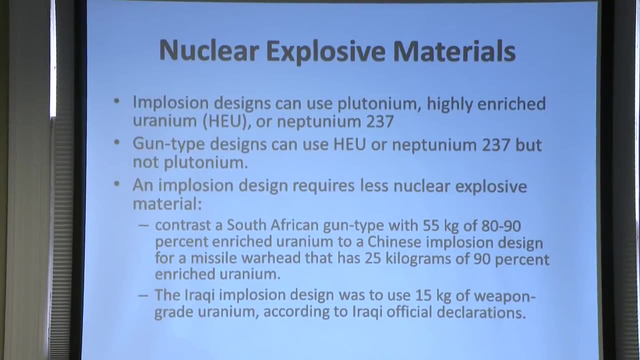 Again, I'll come back to that, But the and actually I'll add something else. If you're working on an implosion system, you can use anything highly enriched geranium plutonium. There's a material called, as you'll see in your notes, plutonium. 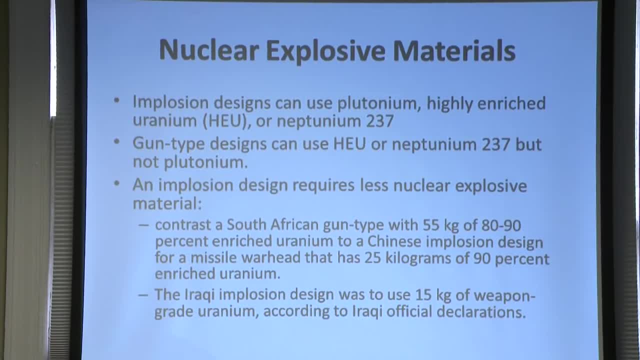 It's called plutonium. It's called plutonium In your readings, neptunium, it's neptunium-237, and that'll work in implosion. But if you go to gun type, not everything will work. 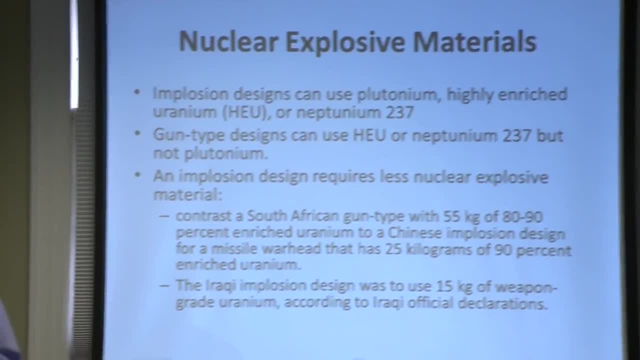 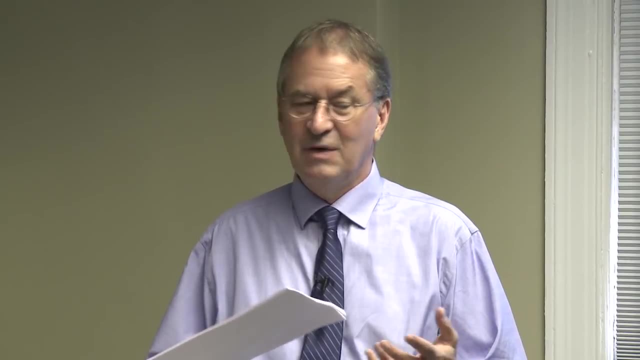 Plutonium won't work. You can't make a gun type device out of plutonium And so. but you can with highly enriched geranium and neptunium, and a lot of it is, if you look at the half-life which, again, you know. but half-life is just the time where half the elements have gone through radioactive decay and changed. So if you had this amount of plutonium after its half-life, you'd have half as much. The longer the half-life, the better it is for a gun type. So neptunium has an extremely long half-life, and so does highly enriched geranium. 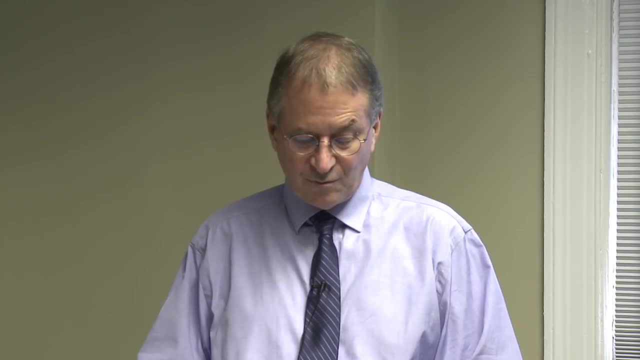 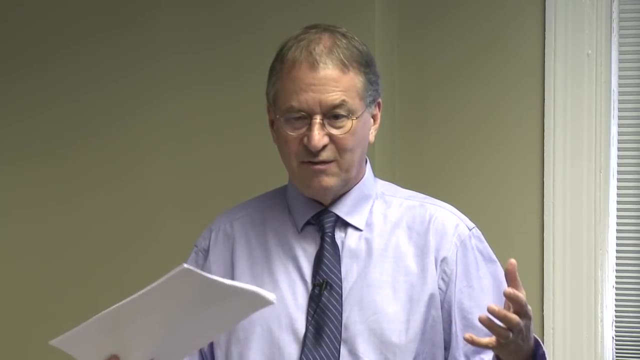 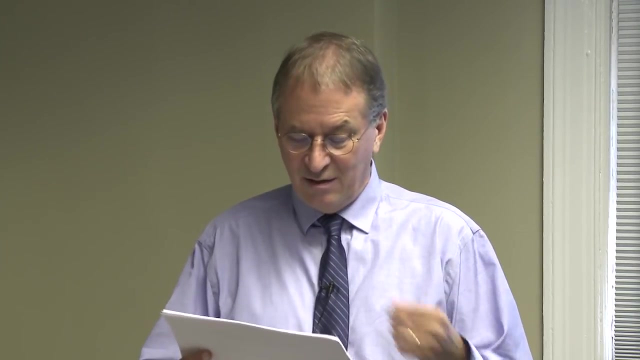 Plutonium isn't that long. Okay, I mentioned that gun types- you're going to have twice the amount needed for a critical mass. So gun types typically use a lot of material And so if you had a- we know this from the South African weapons people- you know their- design had about 55 kilograms of 80 or 90% enriched geranium and later you learn weapon-grade geranium is 90%. That contrasts to a Chinese implosion design. It was a weapon-grade geranium that needed 25 kilograms and it was also partially miniaturized. 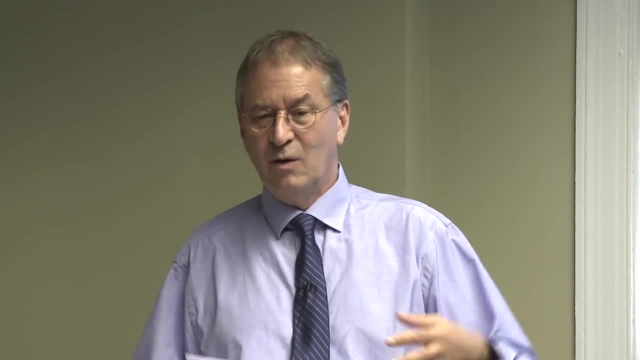 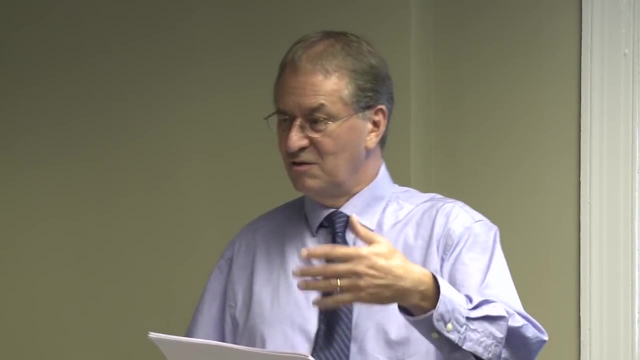 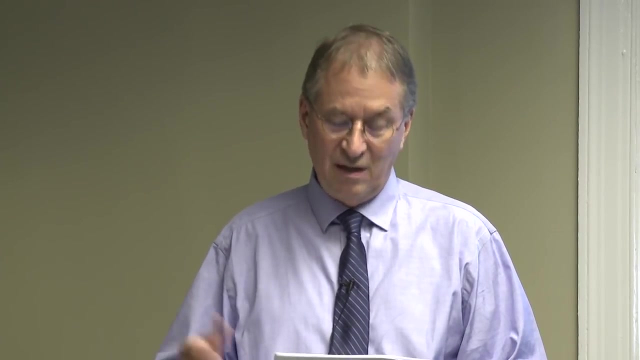 for deployment or delivery by a warhead, And we know this from it was the design given to Pakistan in the early 80s, which AQ Khan was then selling off later, And so the specifications of the design are known precisely in the public domain. 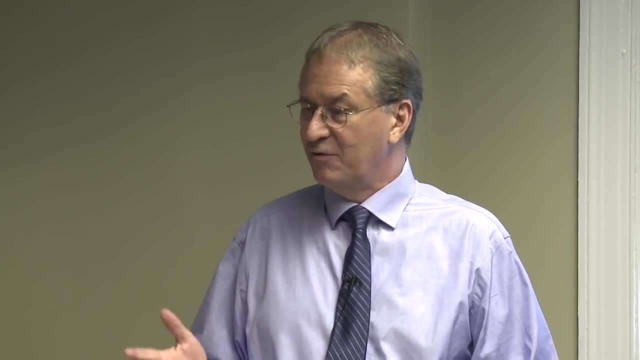 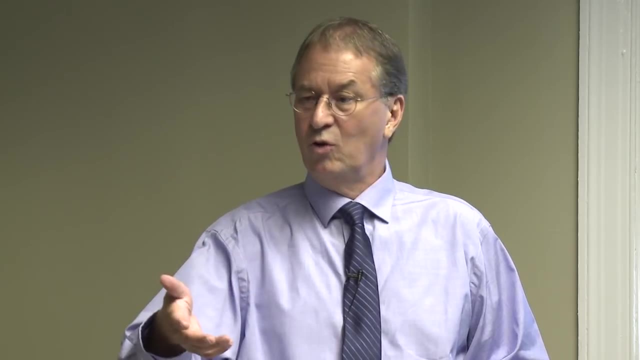 So a rule of thumb is that the implosion system can get by with half of the gun. Okay, So if you're a country struggling to make the nuclear explosive material, then you want implosion, And that explains why the data says Iran, even though it's using, could use weapon-grade. 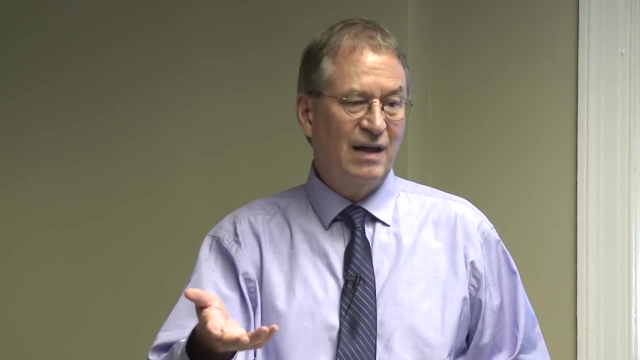 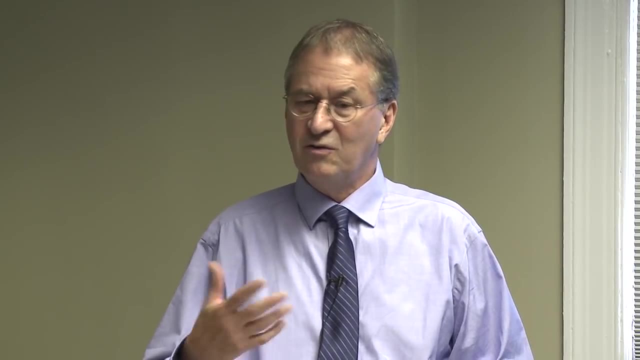 geranium. in their theoretical work they wanted implosion because they felt it would just take so much longer to get enough for a gun type, And so I don't think there's any evidence they've worked on gun type in the past. But there's evidence they worked on implosion. 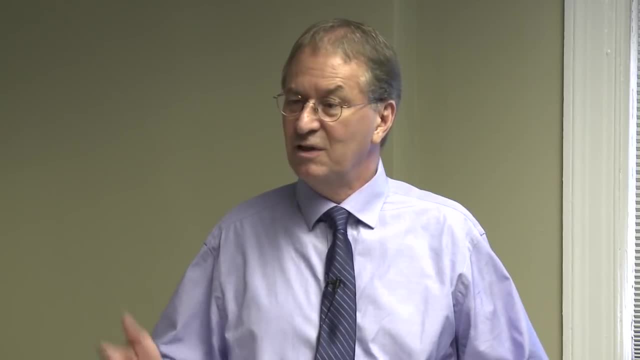 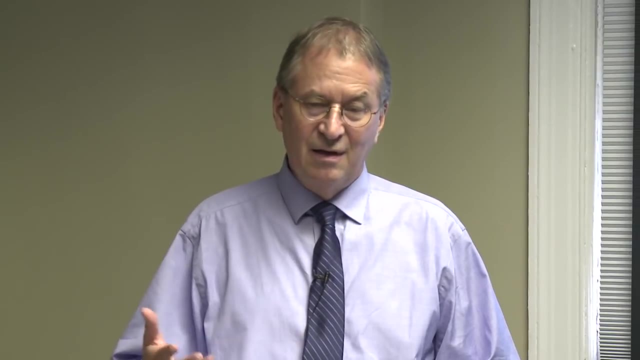 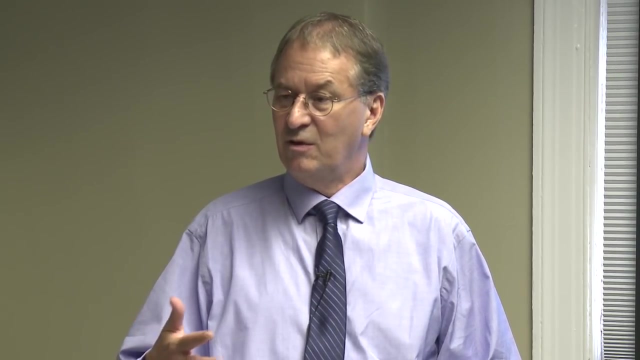 South Africa felt it had a lot, felt it could make what it needed and it stuck with gun type, even though it investigated implosion And the Iraqis in their thinking they were seeking to, they were really worried about enough highly enriched geranium. 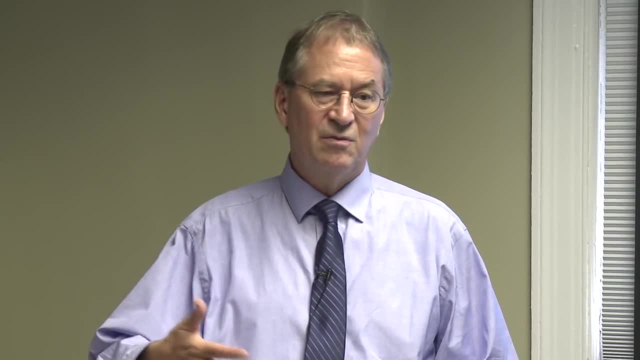 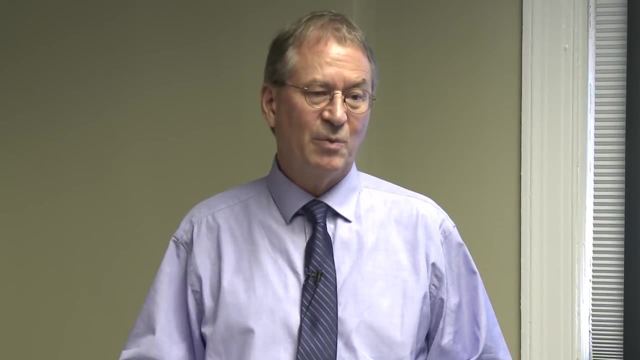 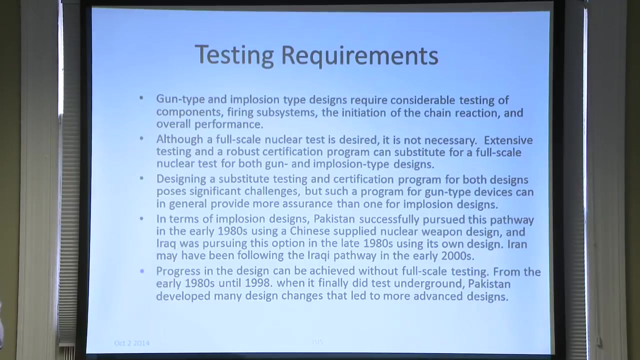 They had initially kind of an old-fashioned enrichment method based on what are called calutrons, and they were trying to design a weapon, at least on paper- that would only have 15 kilograms of weapon-grade geranium. Okay, Let's talk a little bit about kind of give a flavor, why it's hard to build a nuclear. 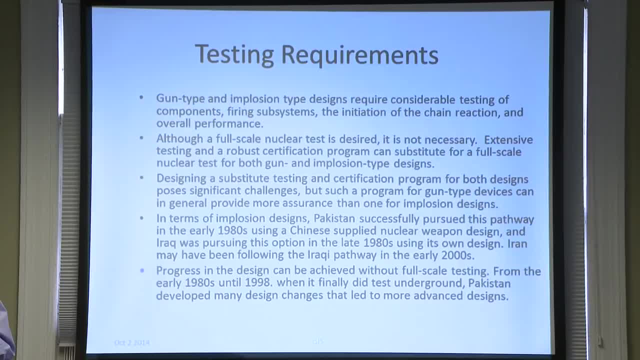 weapon And if you're going to build it, you're going to have to test it, And I don't mean a full-scale underground test like what they used to do in Nevada or out in the Pacific. I mean you need to test the components, the subsystems. 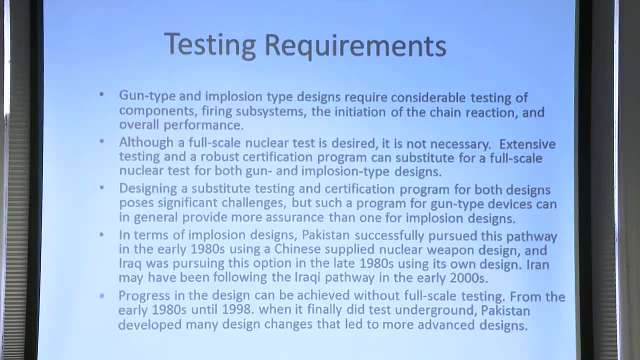 I talked about the high explosives. You have to do all kinds of experiments to design The high explosive components, the shape charge. you're going to be doing an immense number of experiments To understand the pressures and temperatures that are experienced when you compress this. 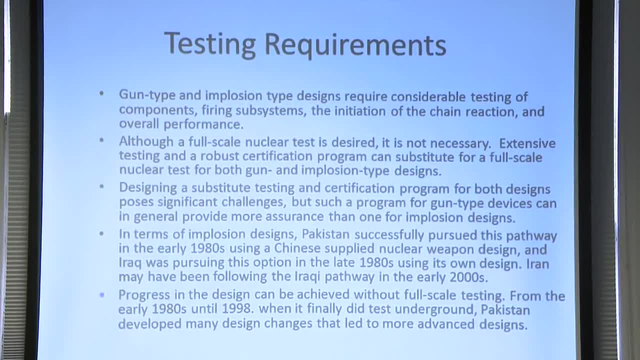 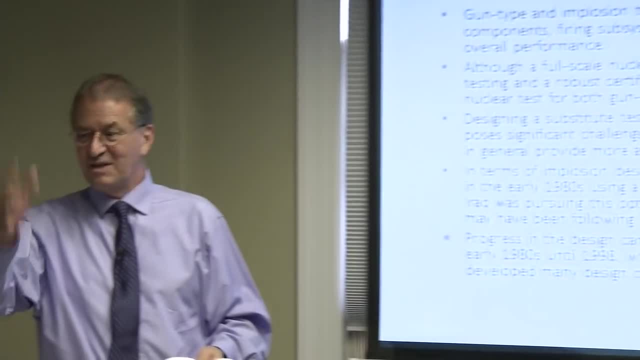 core. there's all kinds of experiments that are done, And then you also have to learn how to fire this system to get it to actually work and not just one side fires, the other doesn't and the little core just dribbles out the 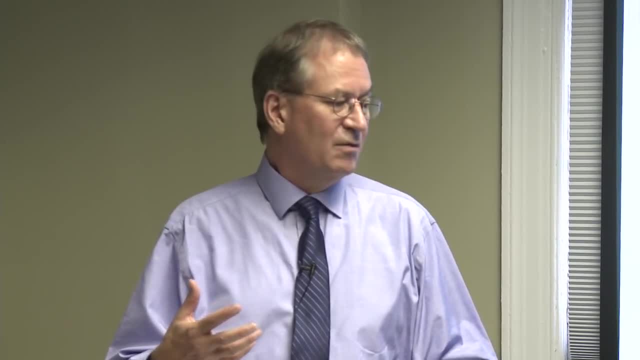 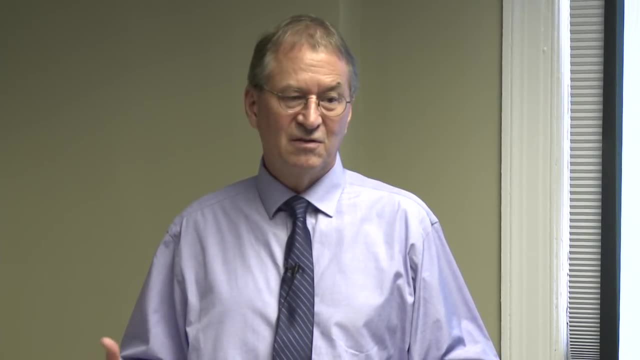 side. Okay Now, in that what people have learned is that you don't need to conduct a full-scale nuclear test to develop a nuclear weapon. That it's simply not true. that if you wanted an implosion system or a gun type, you would. 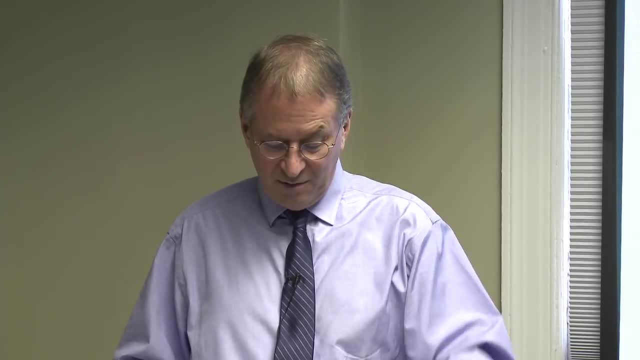 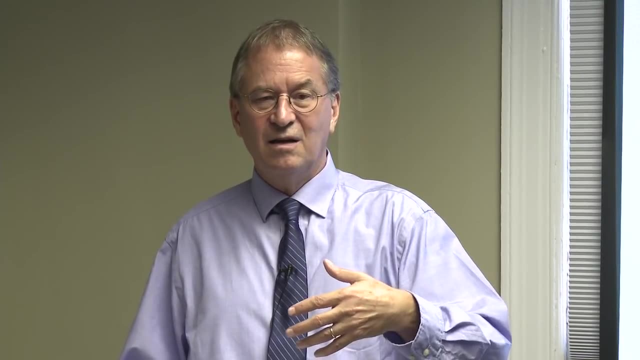 have to have a full-scale underground test. In fact, I remember I interviewed the father of the Iraqi nuclear weapons program, a guy named Jafar Jafar, back in the 90s, and his attitude was that it sure wasn't the first. 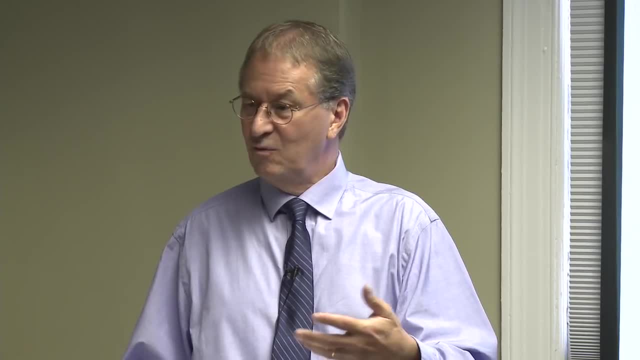 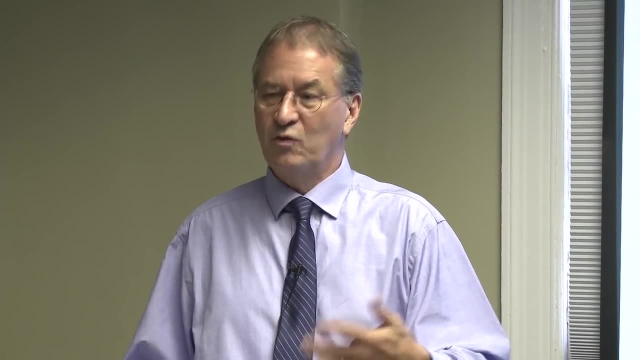 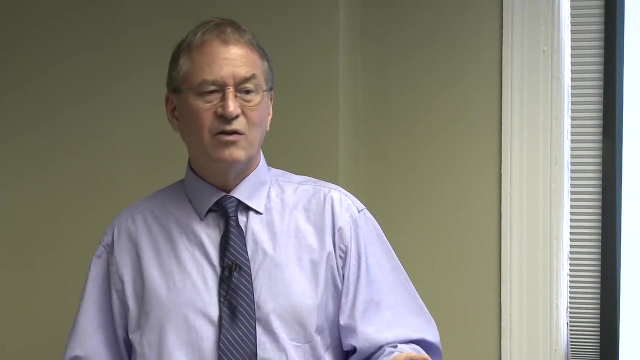 devices we would ever use. It was the first kind of devices you test with. if they were able to build them, The idea would be they would test to demonstrate and then to improve their capabilities. That's what we think North Korea's doing. It didn't actually. it could have gotten by without a test. it had a design, but the test 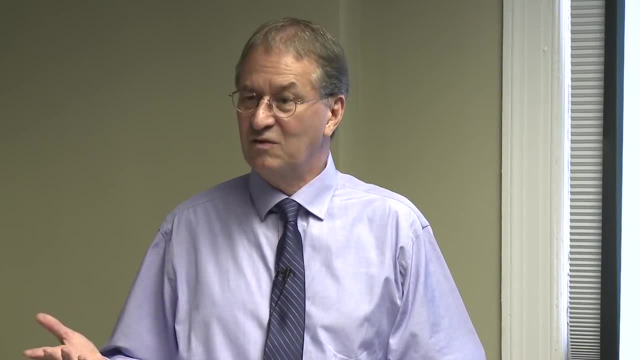 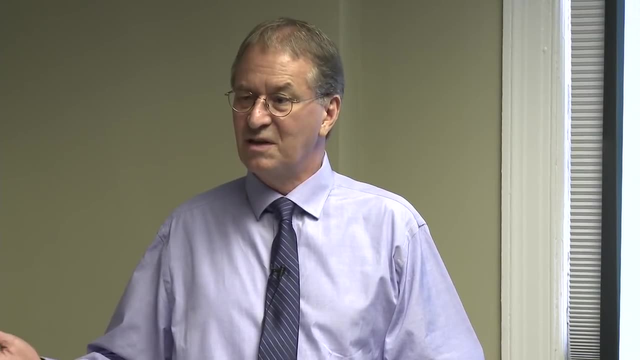 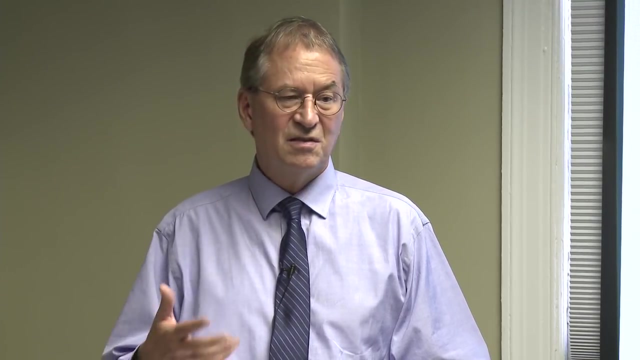 improves its design and makes a point, A point that's hard to miss. In the case of Pakistan, they went through- We call it a certification. I mentioned they had a nuclear weapons design from China and they went through a certification test to prove to the leadership that it would work. But it's not easy to do. It takes some real work and there's a lot of difficulties that have to be overcome. You can also improve designs. We saw that in the case of Pakistan. They talked about it When they tested in 1998, they went through 6 advancements in weapons design. Nothing like what the US had done, even 3 years of testing after 1945.. Testing will allow you to expand your capabilities dramatically, but they were able to advance their design. They worked hard, They took their time. seen in the information seized during the Khan investigations, there were some advanced. 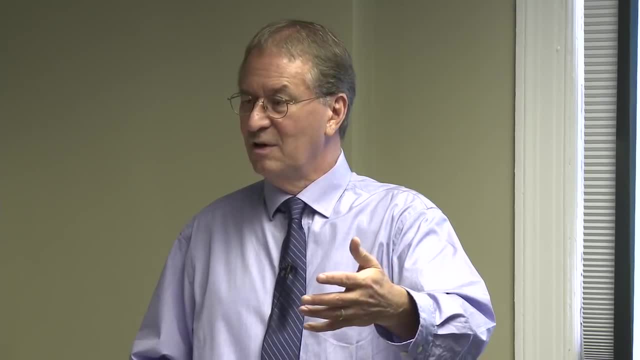 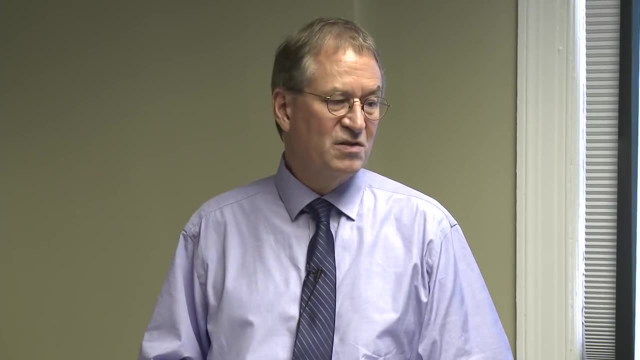 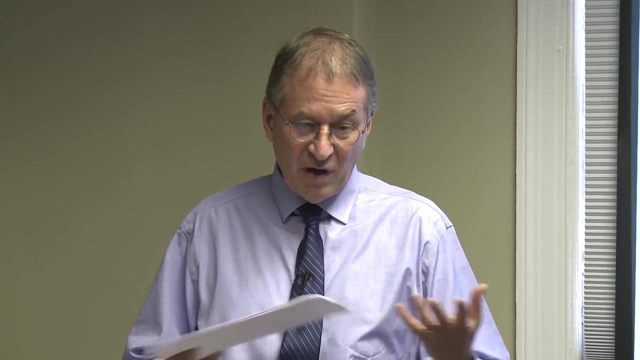 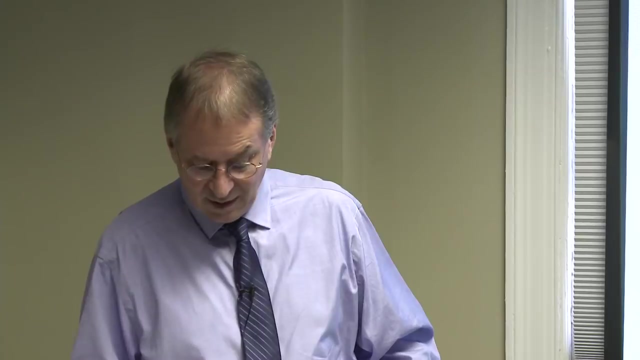 nuclear weapons component designs that Khan had transferred out of Pakistan and were found on computers in Switzerland in one of their cohorts that were involved in their scheme proliferation schemes. But if you don't do full-scale tests you're going to have uncertainties. One of the biggest is: what is the yield? It's very hard to predict the yield you'll get without a test. So in the case of South Africa it wasn't quite as big as this- five or 20 kilotons- but it could easily be by a factor of two. 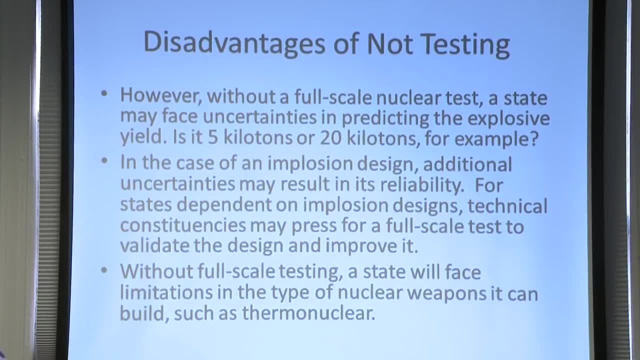 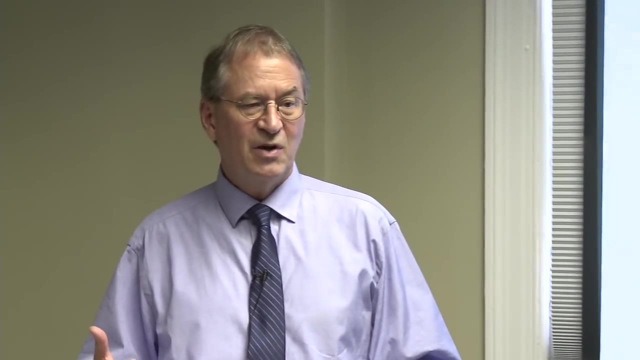 They would have very sophisticated theoretical calculations but they still without data. they would have some uncertainty. Okay, Now with implosion design, you're also going to have uncertainties on the reliability. It is a very complicated system compared to gun type and until you test it you don't. 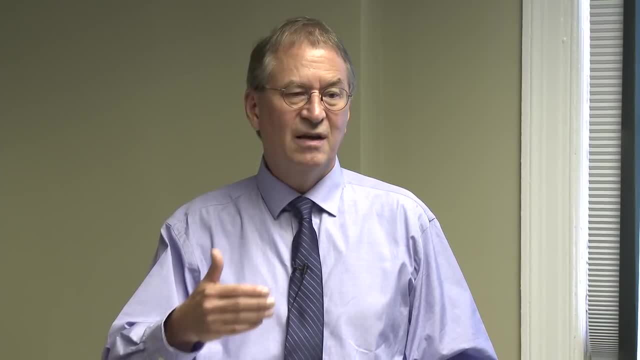 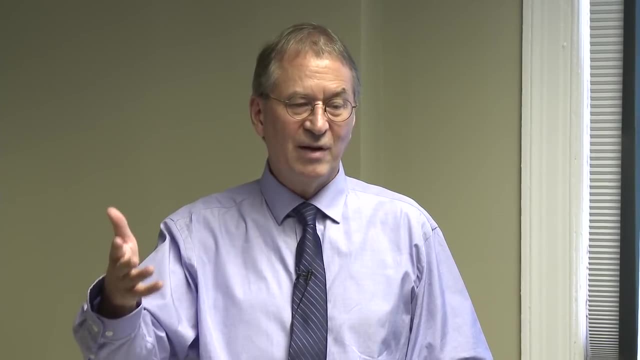 know how well it's going to work. Just as a basic issue of you turn a switch on with a light bulb, you know it's going to work every time until the light bulb burns out. But on a system like this, some of the times it's just going to fail. And so how often is that? Is it? one out of two times? And North Korea got a shock when it did test in 2006 that its yield was a lot less than it expected. It looked like it had misfired, maybe pre-initiated. Also, without testing, you're not going to go too far down the line of nuclear weapons types. I mentioned the word boosting. Even before that, you go from a solid sphere to a shell. Again, you're trying to build momentum at the critical moment. 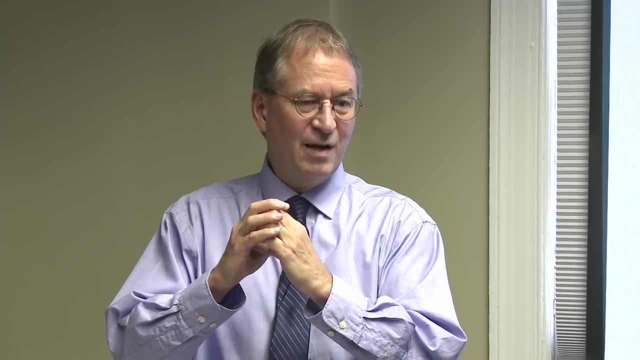 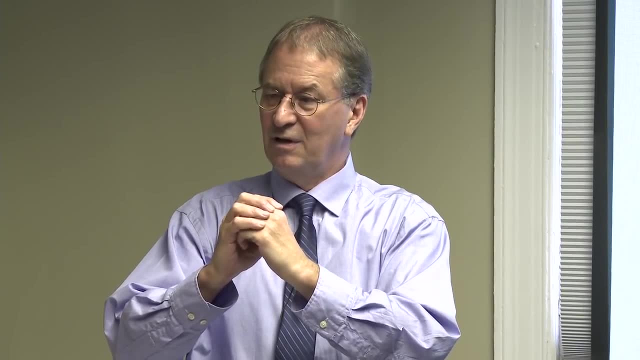 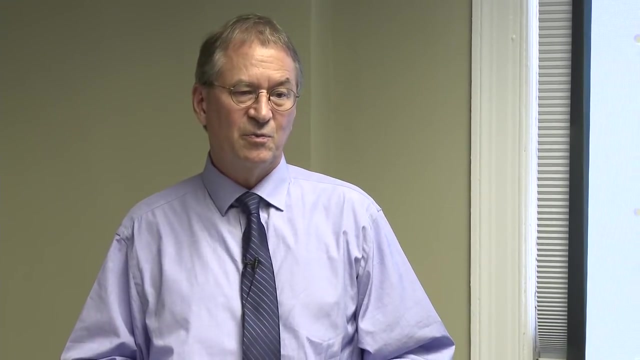 So a solid sphere, compressed in diameter. it's a lot harder to do that than taking a shell that then is pushed and then comes together in a spherical shape, But that's a tricky thing to do and you need a test to do that, to test your methods. 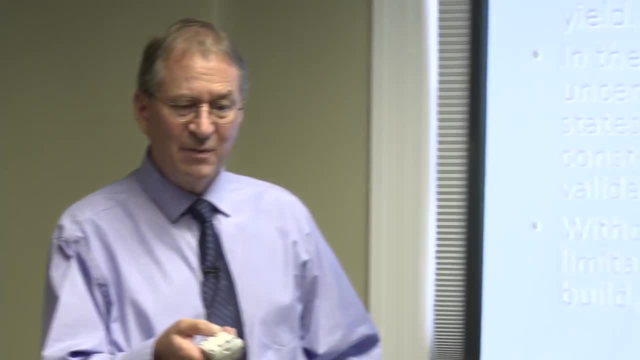 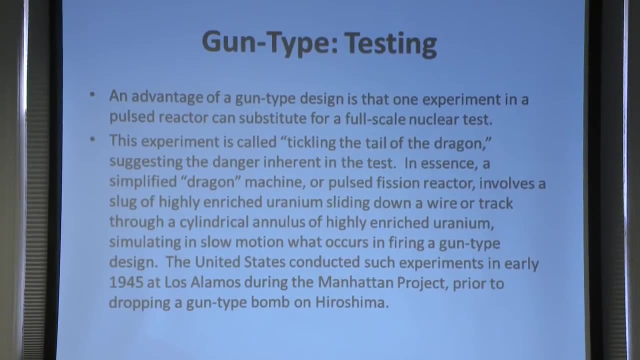 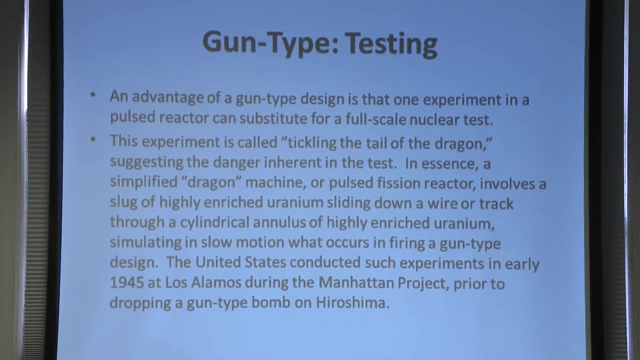 has some advantages: that there's an experiment you can do that tells you a lot about how well it's going to work, and it can substitute for a full scale nuclear test. again, an example would be Hiroshima. Hiroshima was never tested underground before it was dropped. Trinity, they did test. 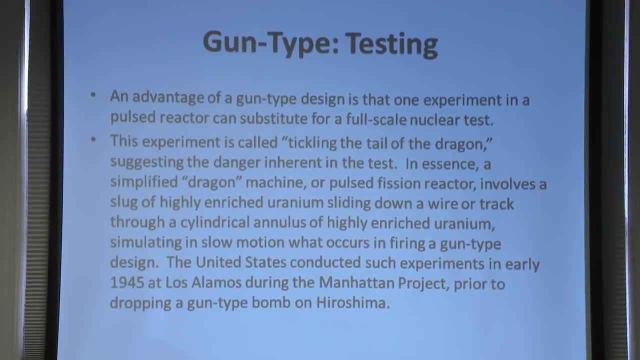 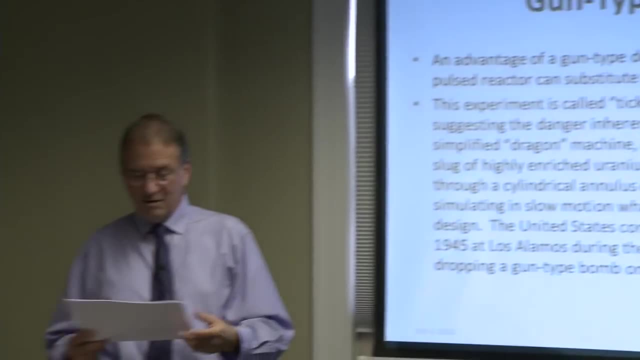 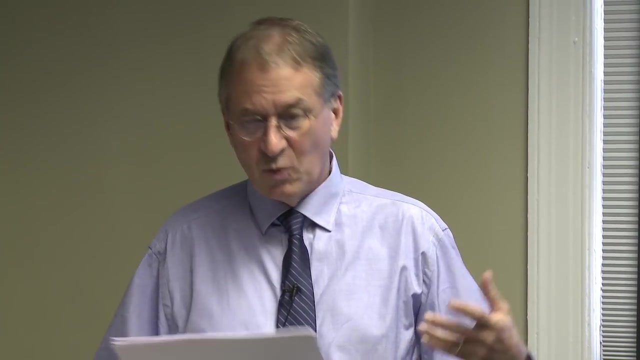 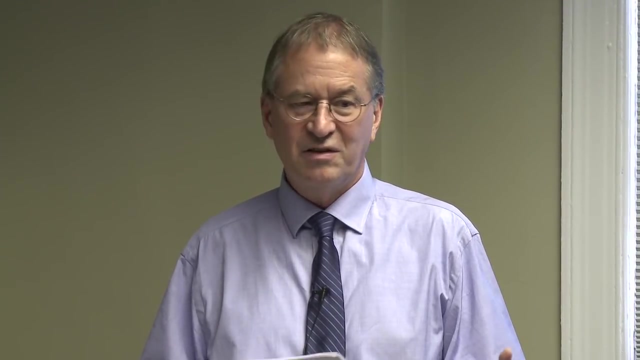 I shouldn't say underground. they never, I'm sorry, but they. it was an above ground test in Trinity but there was no need to test the gun type device and the terms in the Manhattan Project they called it. the experiment was called tickling the tail of the dragon. 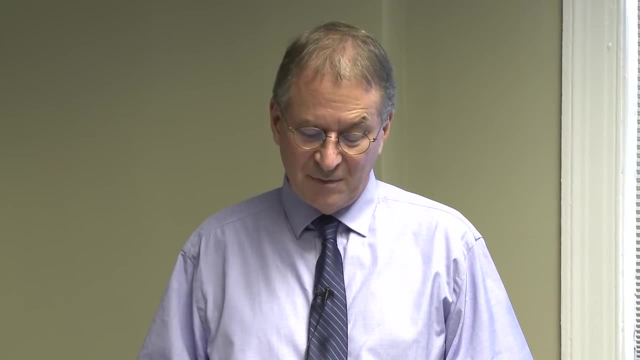 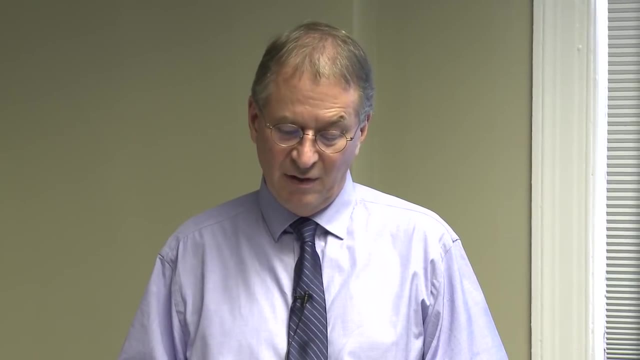 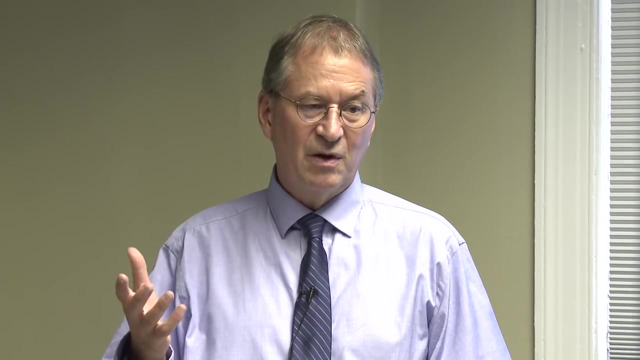 and what it is is. it's it's a machine and it's extremely dangerous to do. it's technically it's called a pulsed fission reactor, but what you're really doing is taking, in the simplified version, you're taking a, a slug or a piece of highly enriched uranium or weapon grade uranium. 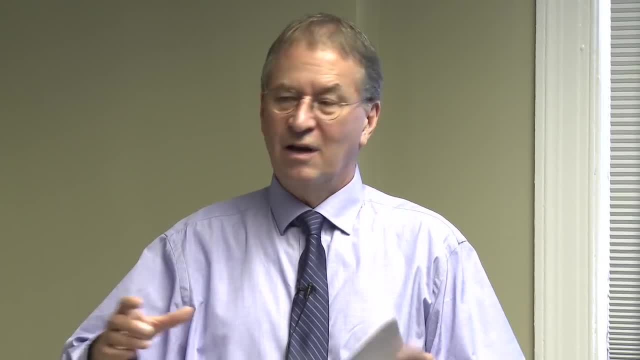 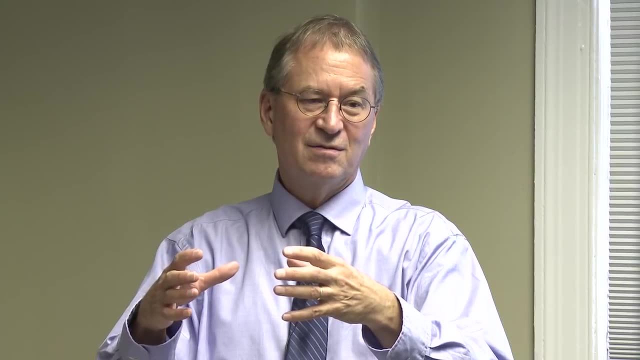 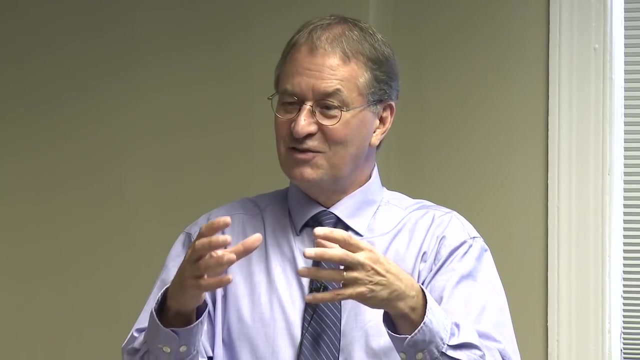 and sliding it down a wire or a track, through an annulus of weapon grade uranium, and so when it, when it goes through, it's critical for- and you've hope it continues- that it doesn't get stuck and that's actually the danger- is, if something happens where it gets stuck and it's critical, then you have this critical. 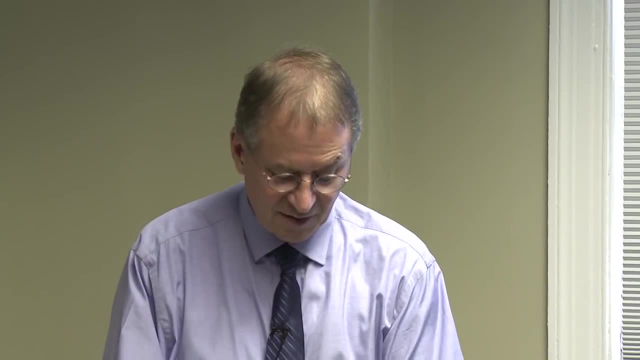 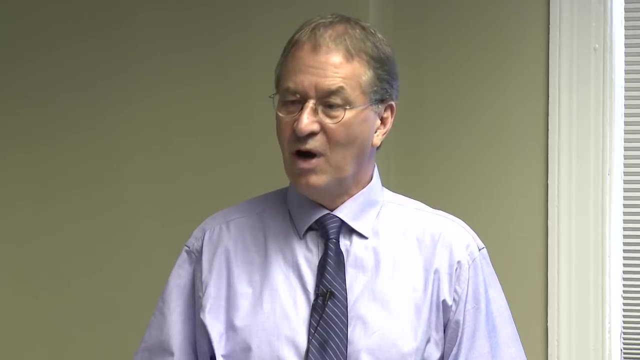 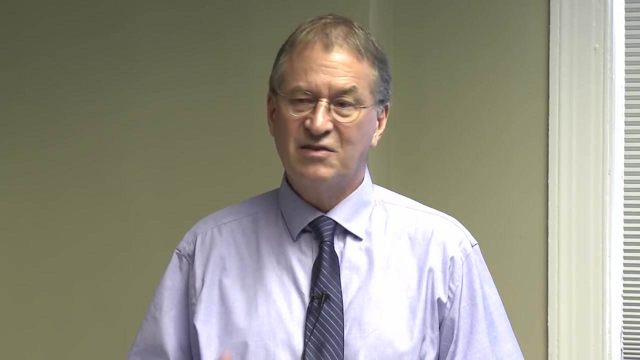 essentially a reactor, unshielded reactor that is operational, but if you measure what's going on when it goes critical, you learn a lot about how your, how your bomb will ultimately work. and the US conducted those experiments and the documents have been declassified on the US. 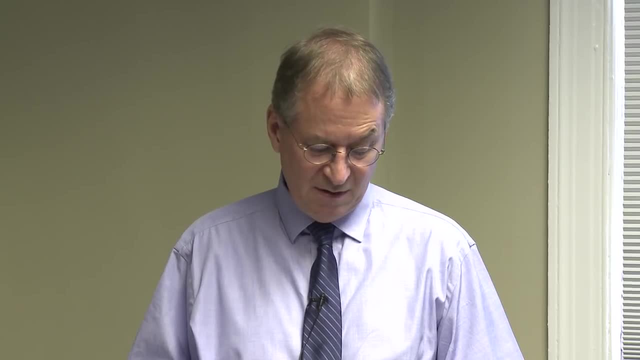 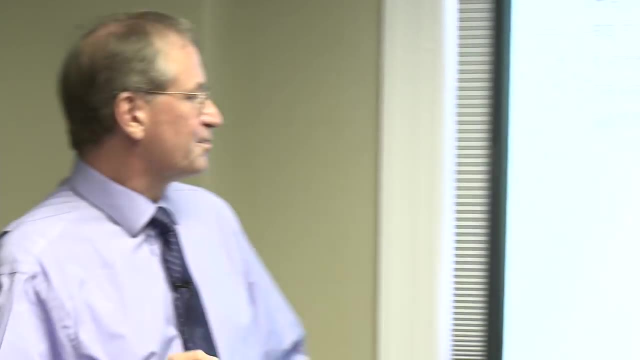 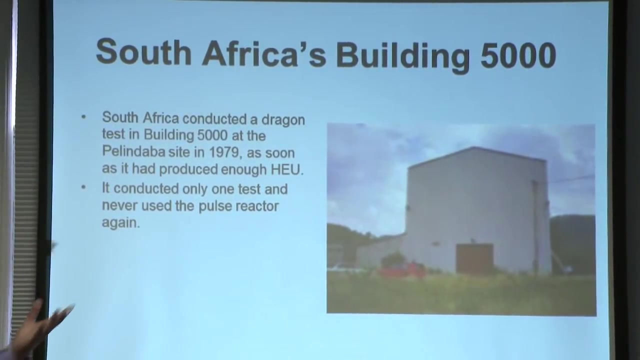 US experiments on tickling the, the dragon's tail, and in South Africa. just to give some examples. this is the building where they did it in South Africa. it's called building five thousand and they did it in nineteen, seventy eight, in fact, as soon as they got. 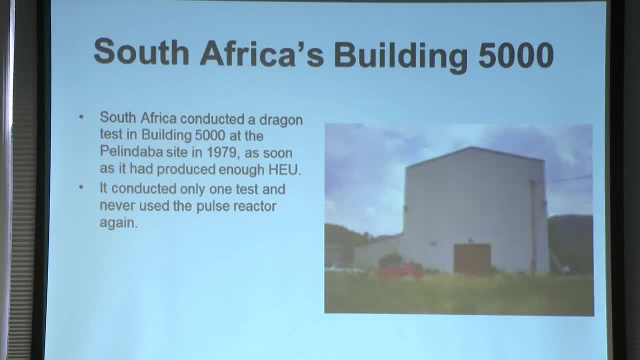 this was eighty percent enriched uranium. they couldn't, they didn't, they couldn't make ninety percent at that time, the enrichment process wasn't working well enough, but as soon as they get enough, eighty percent um. and what they did is they had a design that required fifty five kilograms. 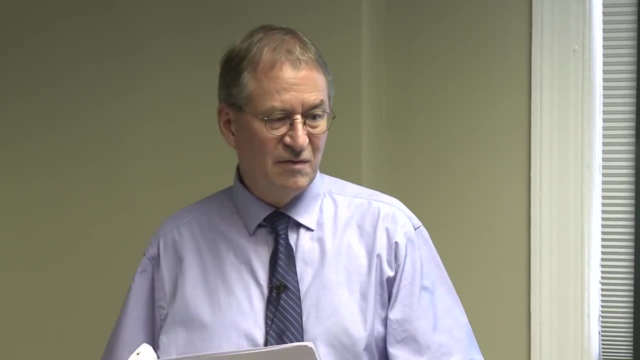 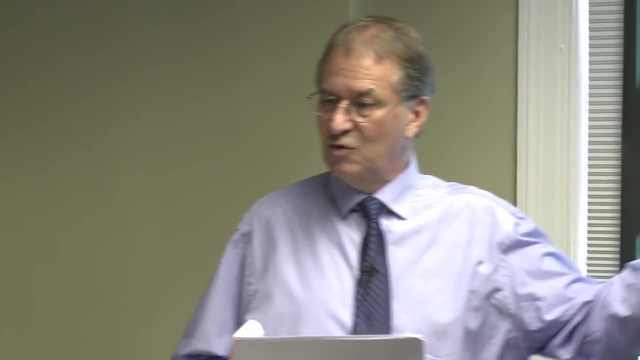 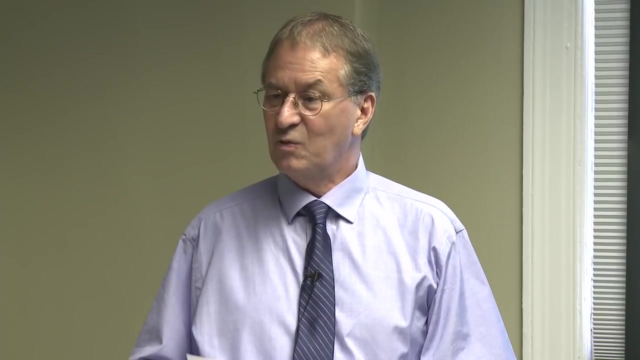 that's how much they got, but with eighty percent they would get less of an explosive yield than ninety percent. but this, it was exactly the same design, and so they they then took, took it to there and did this, this experiment, and then that's, that's the one test they did in this reactor. they never operated it after that. 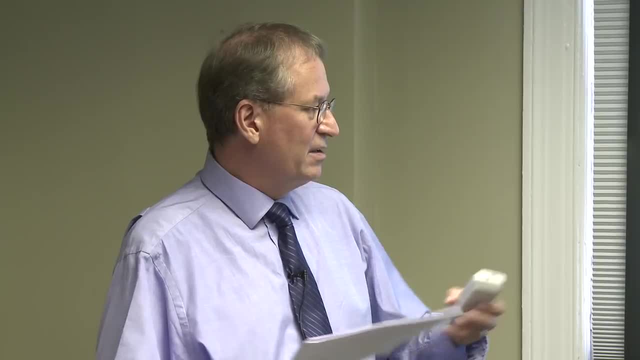 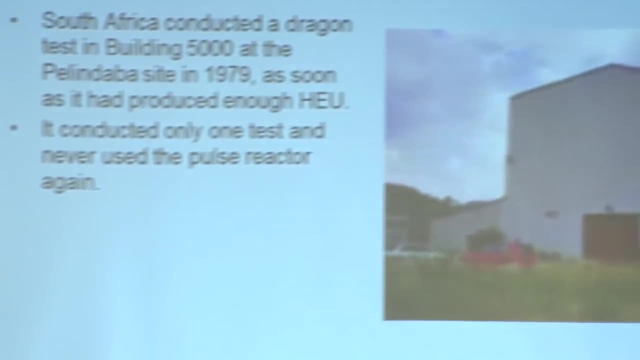 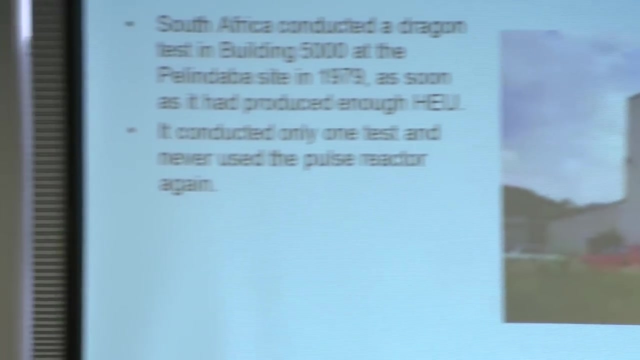 and I, and again, just to bring in the satellite imagery, it's a very nondescript building. I mean I I met a. just by coincidence, our daughters went to the same nursery school or school. I met one of the main participants, one of the major participants in this program. 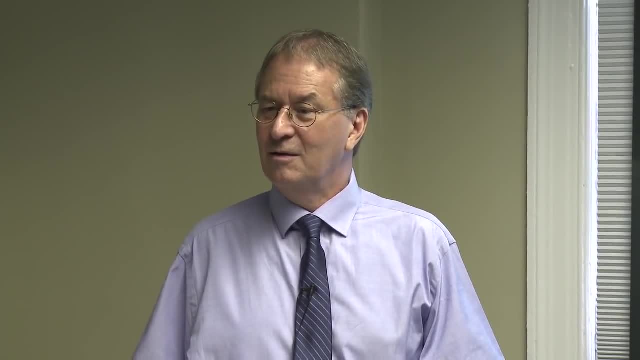 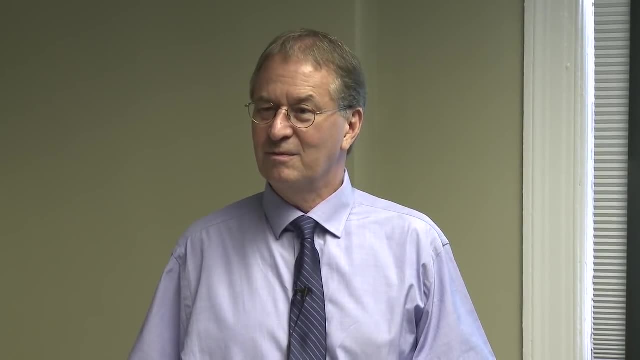 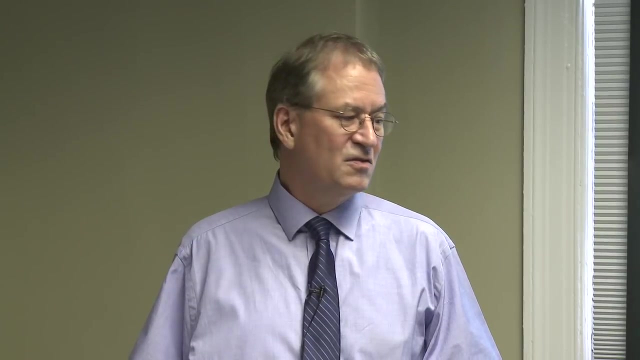 and he had not intended to be a spy in the in the seventies and early eighties but he didn't want to work in the nuclear weapons program and and he had been at one of our ivy league schools as a phd or postdoc and and he just wasn't comfortable in the weapons program he had. 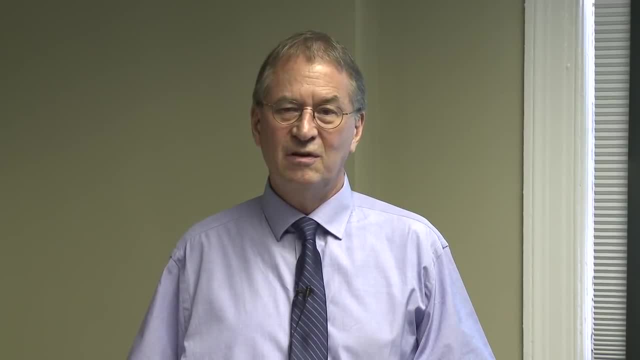 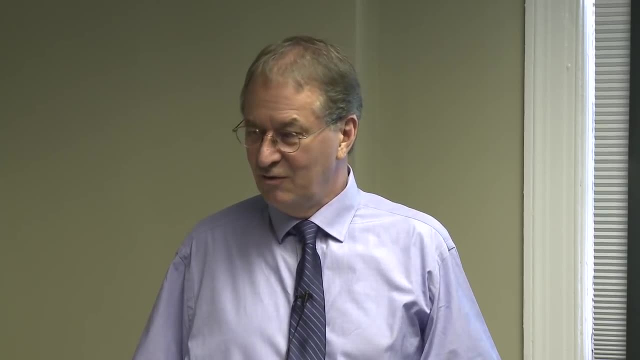 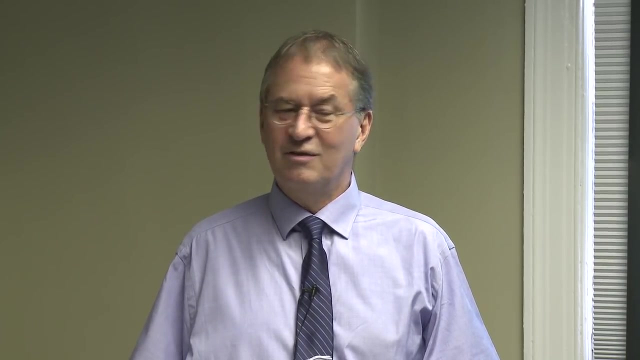 other responsibilities at the nuclear site that didn't involve weapons. and he just left one day, just left south africa, which turns out to be illegal under the south african classification system. so they put out a to uh interpol, a red notice and accused him of being a drug dealer. 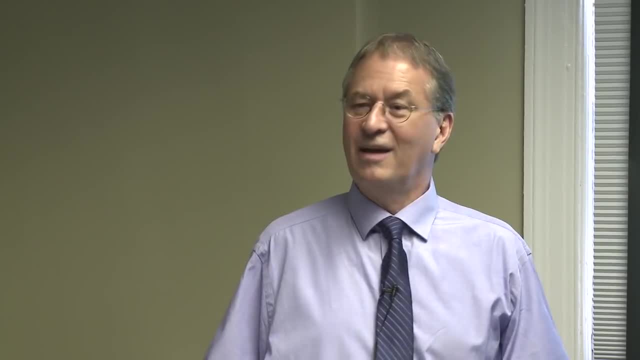 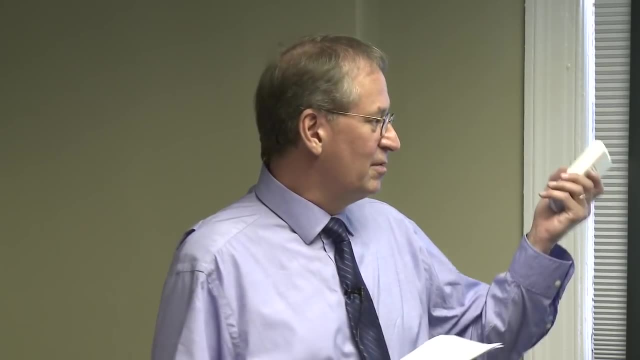 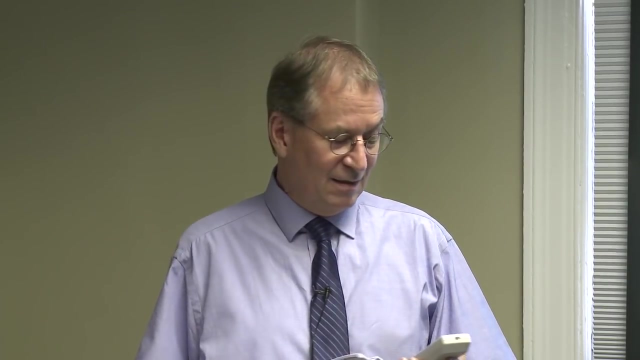 and he was in the united states by that time and he decided that he didn't feel like being arrested as a drug dealer. so he approached our government and and revealed a lot about this program in the seventies that it wasn't that well known and the uh. 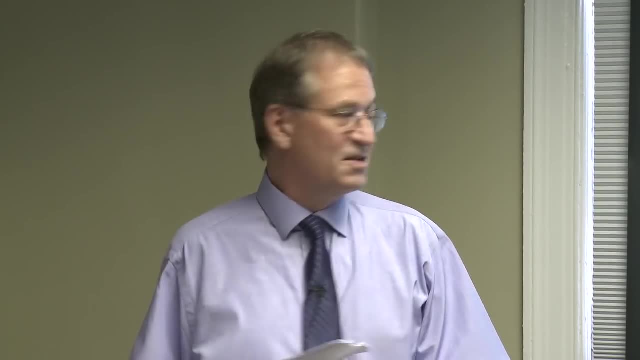 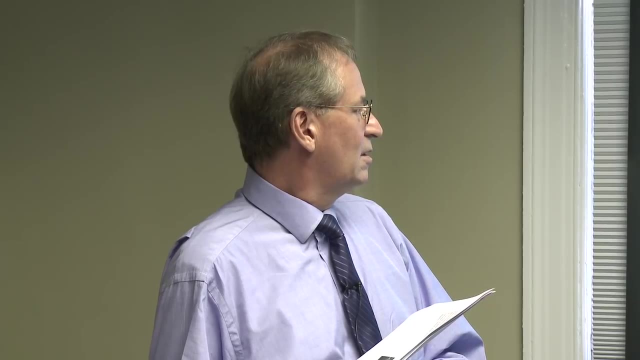 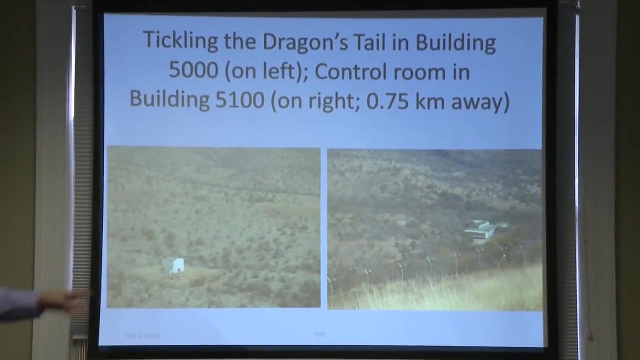 one of would have been this and this. this facility was actually, if it was working, was there was no one there, and that and that. this. this is the building. five thousand. the control building would was about three quarters of a mile away in in what was is called. 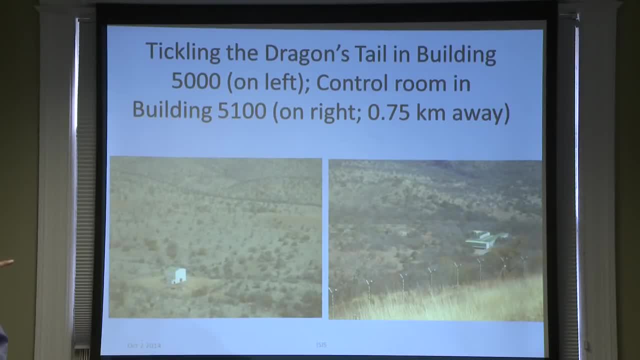 building fifty one hundred and it has of the. it had a lot of other functions, but in it was the control room for that reactor and that this, uh, you can see it here this time. natural, this helps, but what this is is a just a google or standing on the table. 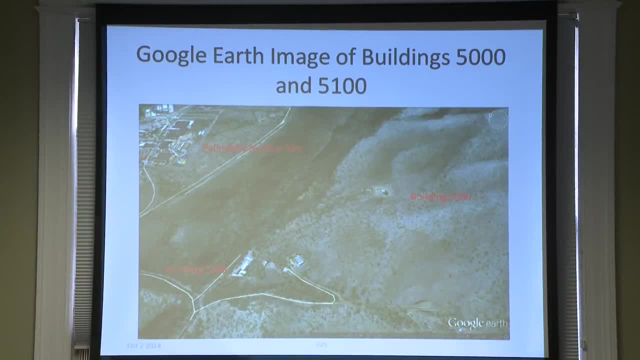 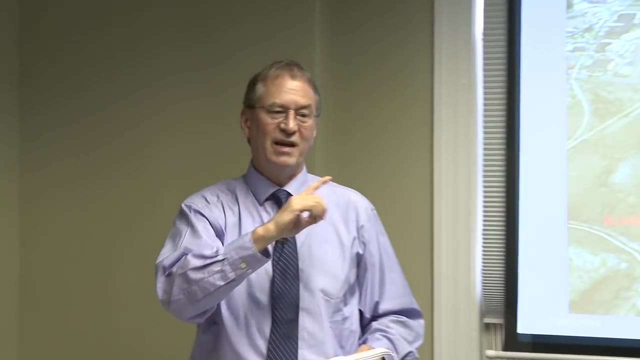 and uh, the structure of this has to do with the nuclear of the Building 5000 and Building 5100.. Building 5000 is in a valley, so that if you're at Building 5000, you look around, all you see is the hills. The natural way to protect was. 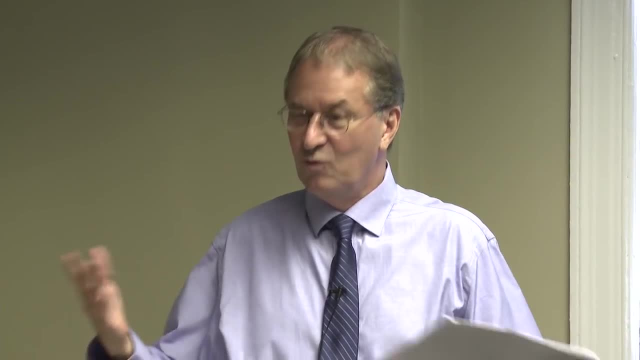 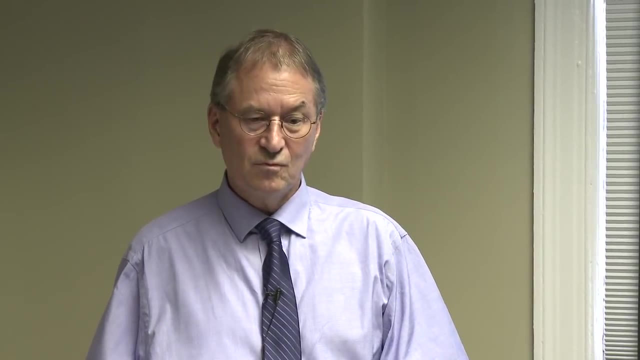 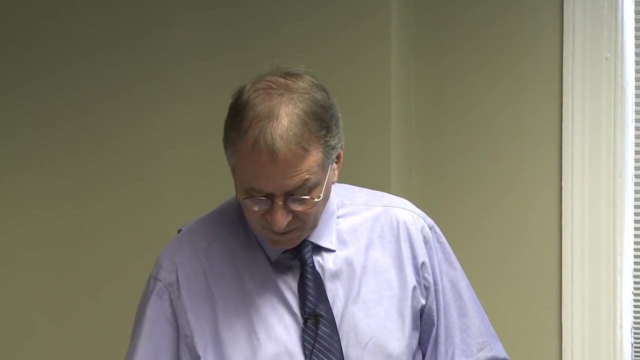 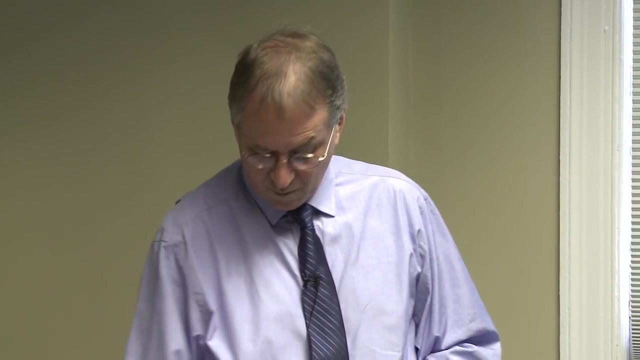 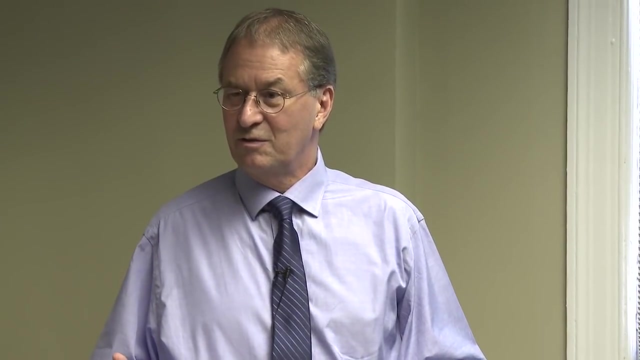 to use the hillside. If this thing went bad, then they would have the geology or geography to protect them, But once they did the test, they had much greater confidence. This is an example where we'll start to hide their capabilities. This was a first attempt. 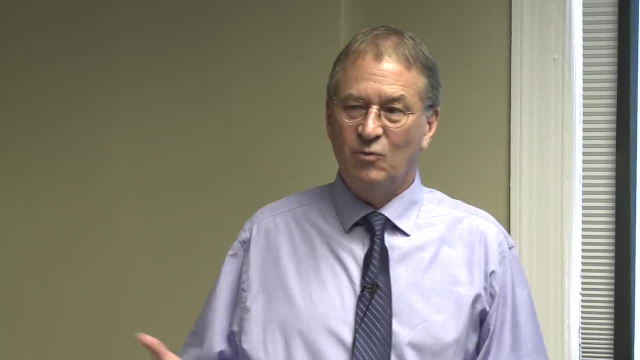 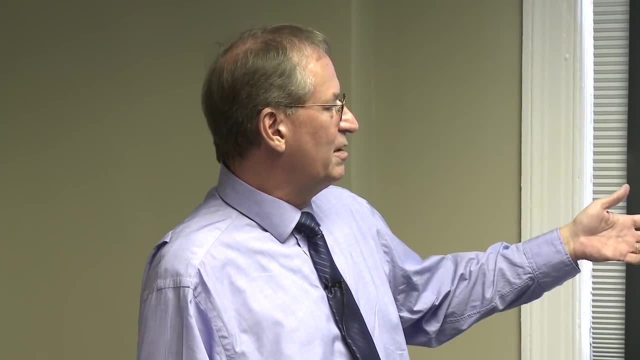 In this case, in a sense a defector- It wasn't really, but a defector- reveals the program in great detail. It's a program that gets revealed too because it's so close to this Pelindaba nuclear site. This is the 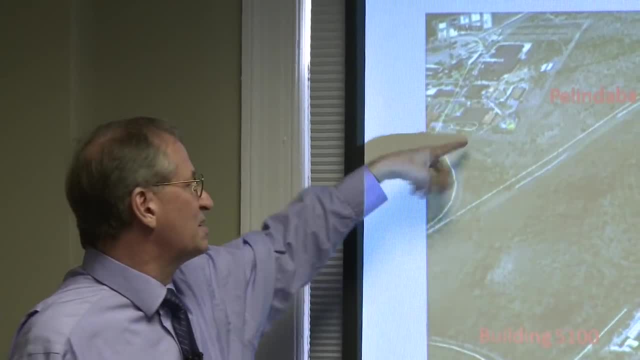 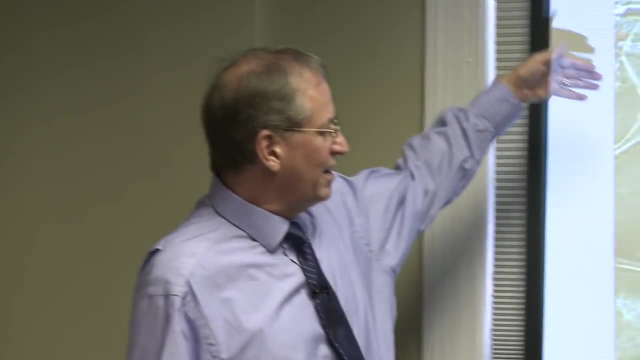 South African's main nuclear site where they have civil activities. There's a US-supplied reactor right there. US people go there, Others go there, Then down the hillside, down in a valley. there's a river down here, the Crocodile River. Then they put these secret. 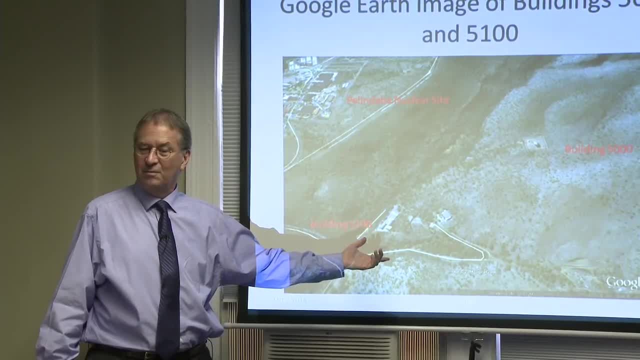 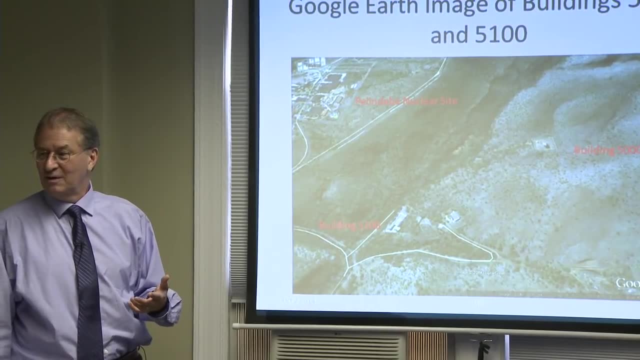 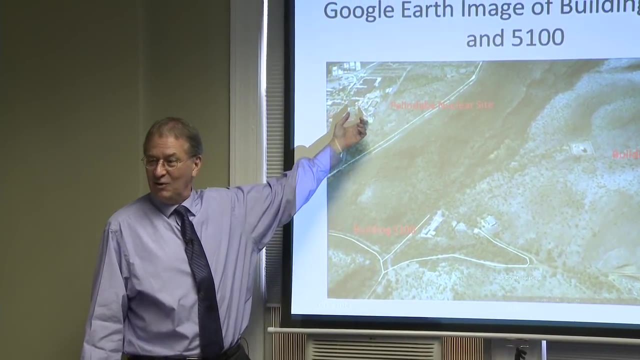 nuclear weapons there. I remember talking to them. They weren't that convinced it would work, because they were also developing implosion weapons, at least studying implosion weapons. Well, what do you do? You blow off high explosives. If you're up here visiting and you hear explosions, 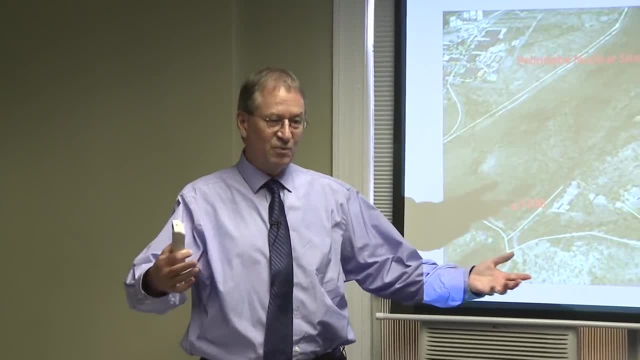 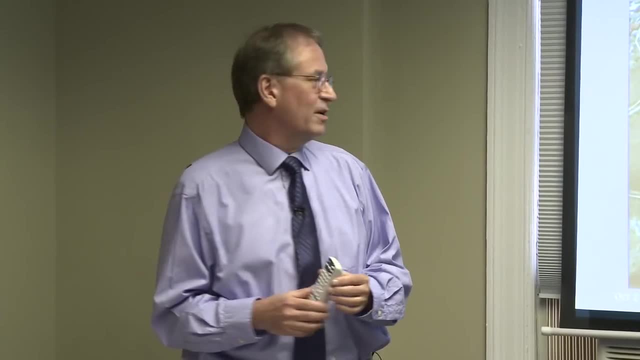 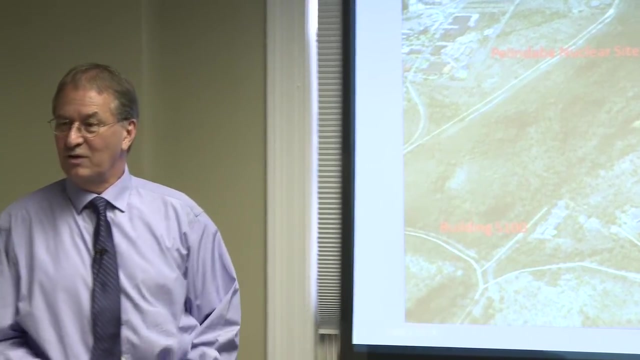 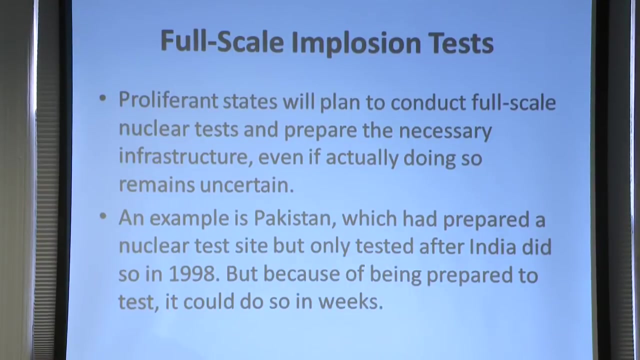 down in the valley. you would probably tell your government if you're paying attention to these issues to take a closer look. So this idea of putting things adjacent to a declared nuclear site isn't the most effective way to do it. I mentioned how it's difficult to build an implosion system, Typically a country that's 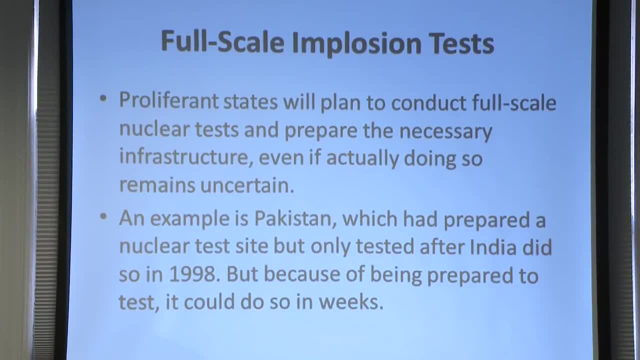 going to do. it is going to be thinking about a full-scale test. Probably the best example is Pakistan. Even though they had a Chinese design, they developed a certification program to say it would work without full-scale testing. They still don't have a full-scale test. They're 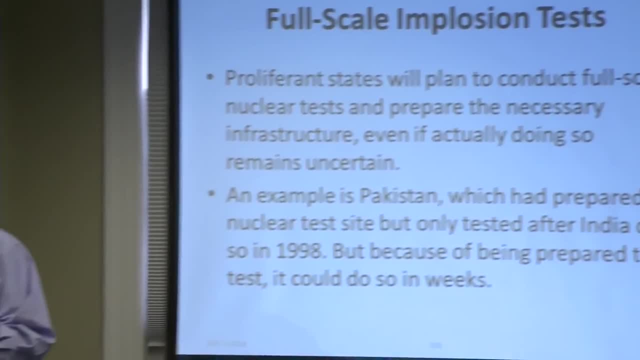 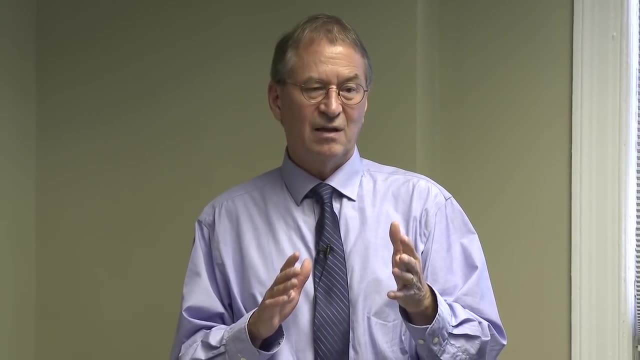 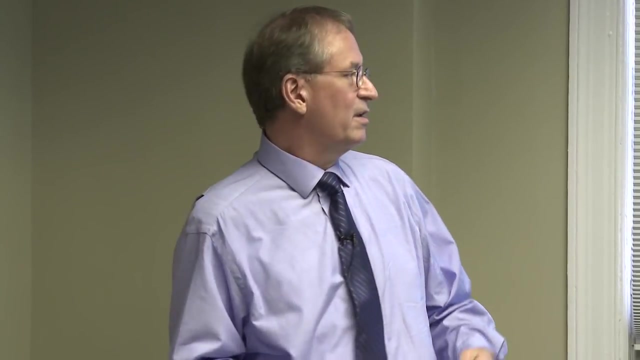 just going to do it on their own. They started building a nuclear test site in case they wanted to test. In 1998, after India tested, Pakistan was able to test within a few weeks and conduct five tests simultaneously- I think it was five. Then, a day or two later, they detonated another one at another site. 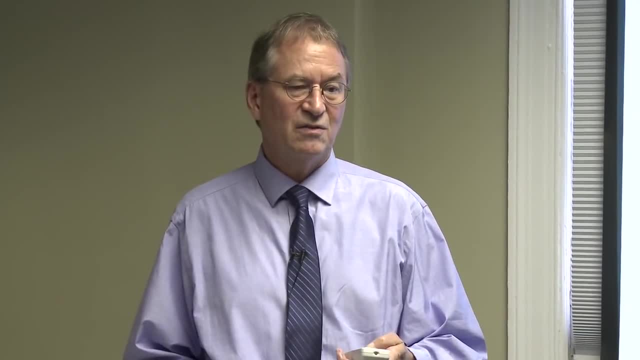 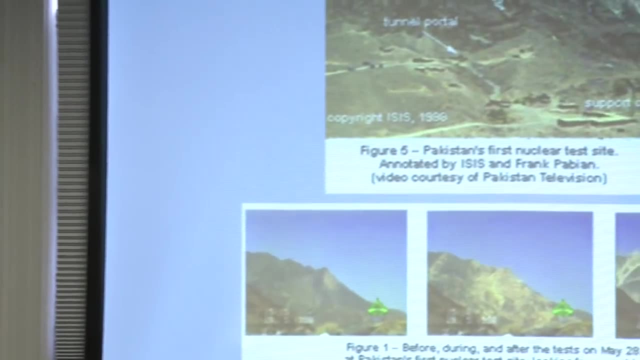 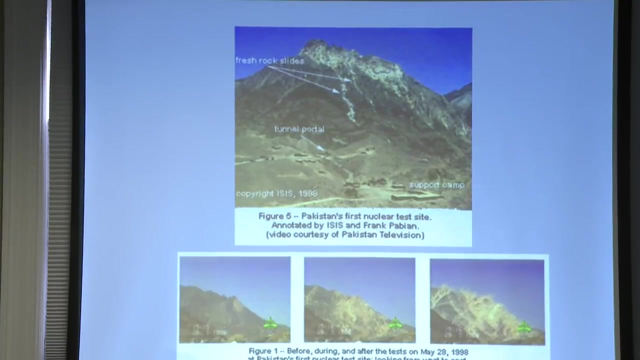 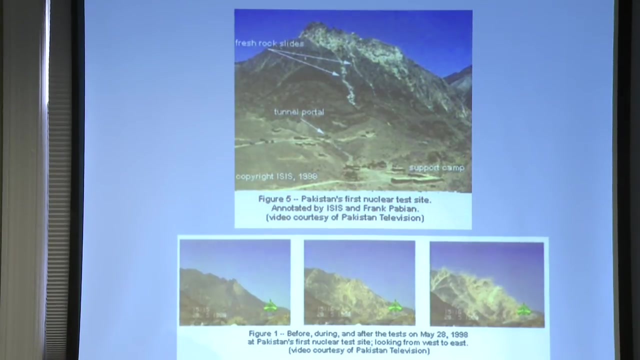 You look for these test sites. if you think the country is following the implosion route, Here's the mountain. No Pakistanis detonated their device. There's a video. Did we ever put the video on our website? Yes, I think so. 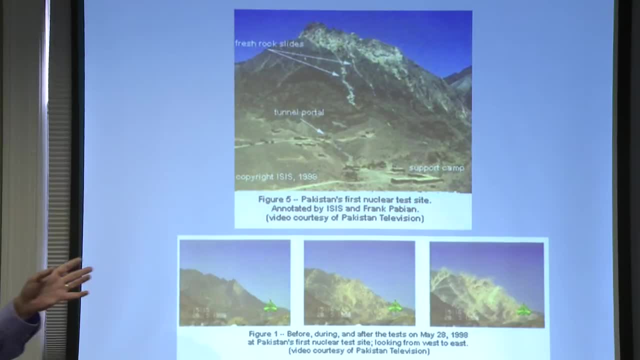 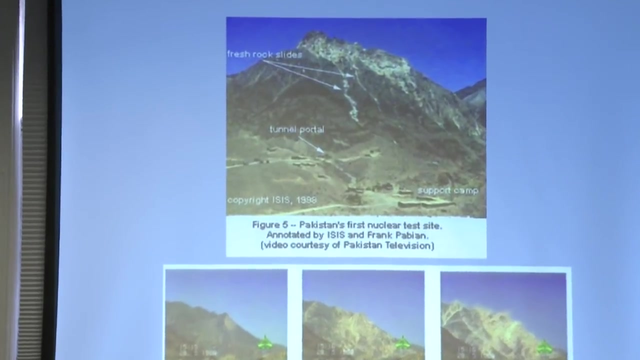 This wasn't publicly known even until after the test. I'm forgetting some of the chronology. it wasn't known after the test, but we did a study to find this location. One of the things we did was we wanted to get the video and we called the Pakistani TV station and 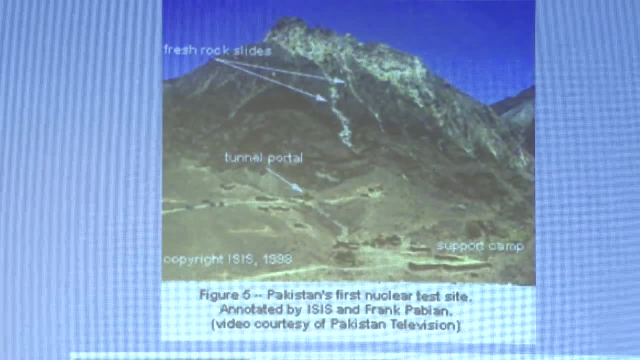 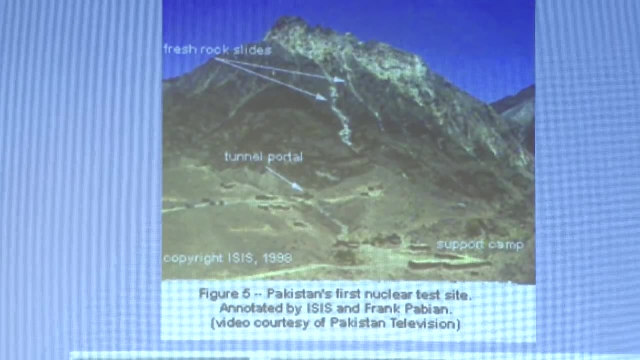 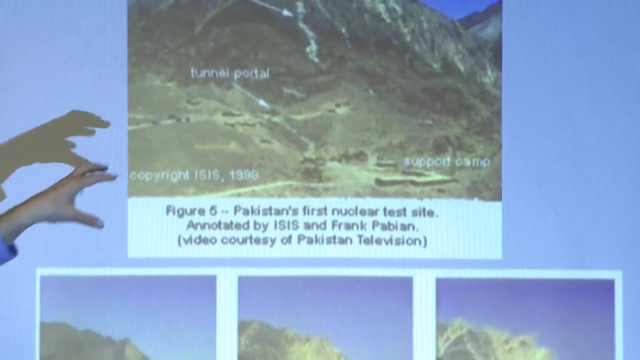 asked for it. They sent us this incredibly great- it was called beta quality video and it arrived in a burlap bag one day from Pakistan. It was just remarkable imagery to see. You could actually look at it and zero in on the facilities there and how they'd actually. 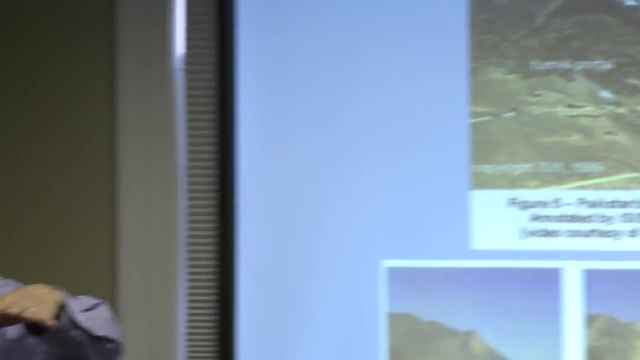 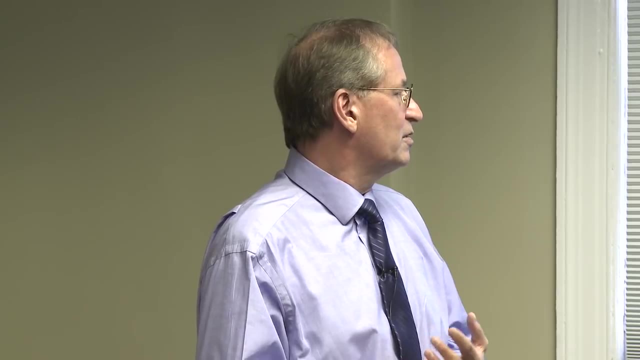 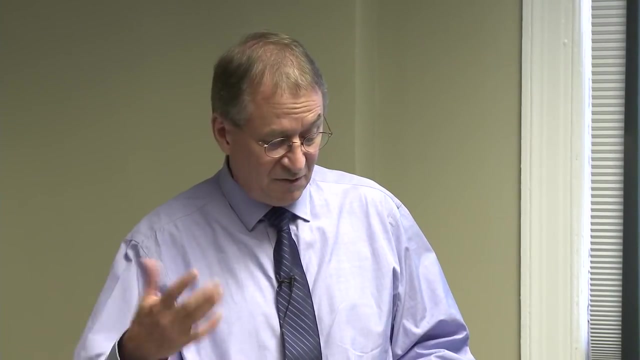 camouflaged. From above this looked like a village, but it was actually bunkers and instrumentation locations that were critical to doing the test. I think this stuff is on our website. I apologize, I forget these things. It's been quite a long time and I'm getting. 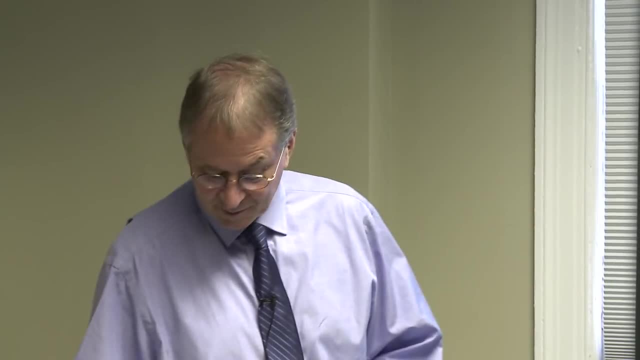 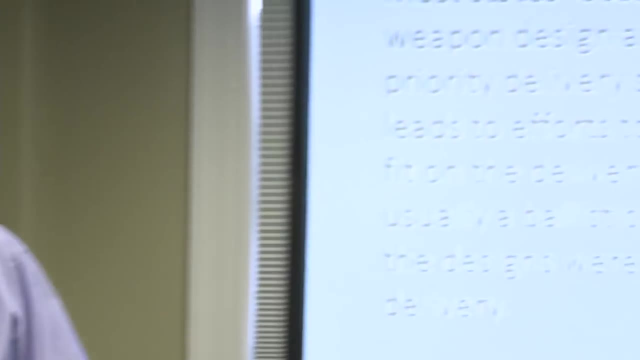 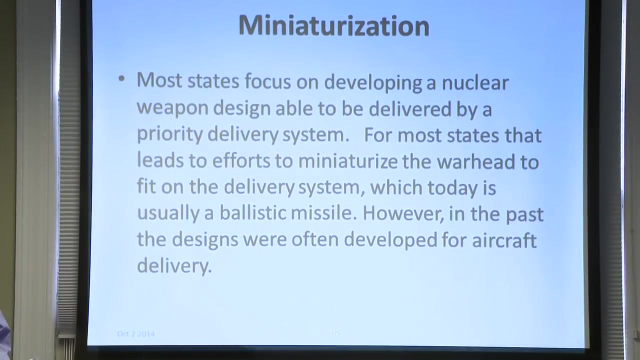 old and forgetful. The next section I wanted to cover was on miniaturization. It comes up in the debates all the time. If you follow North Korea, a lot of the debate is: can they put a warhead on a missile or not? There's a complication to the debate: can the missile reach America? or when will it reach America? That's a more profound debate on how capable they are with ballistic missiles 0 over. can they miniaturize and actually put it on a shorter range missile which would be called the nodon? It really follows that most states, when they think about building nuclear weapon, are going 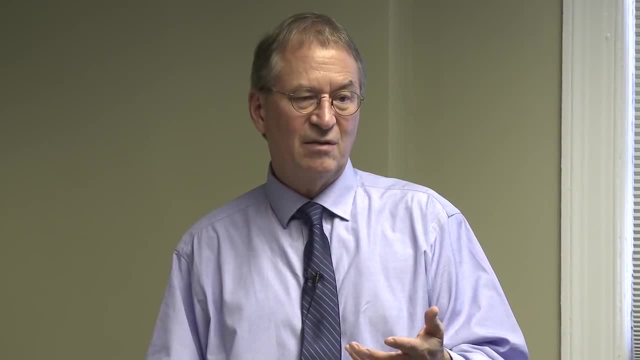 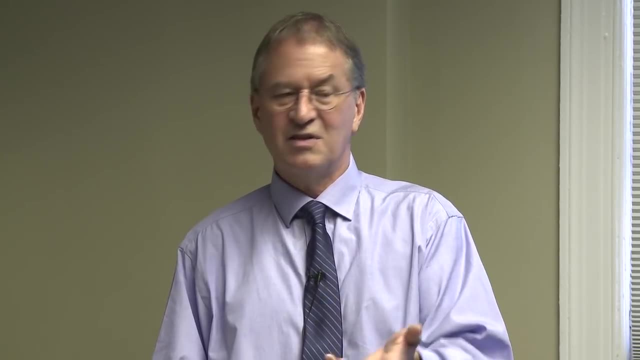 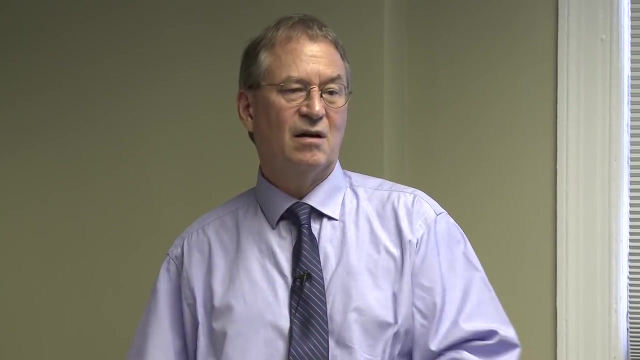 to have typical delivery systems that they feel they can control. It can change with time. In Pakistan their delivery system of choice was the F-16, and then they bought a missile system from North Korea, the Gowri. By the late 90s they switched to ballistic missile delivery. Again, it's a logical progression. A lot of this is all just a logical reasoning that you want to be able to get through to your enemy. Your enemy is developing better defenses. attack aircraft such as the F-16 can work, but they can be shot down. 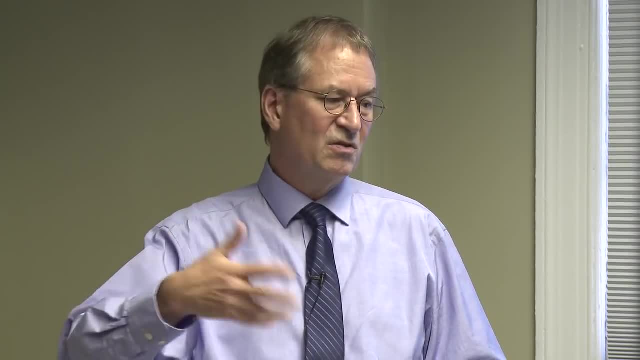 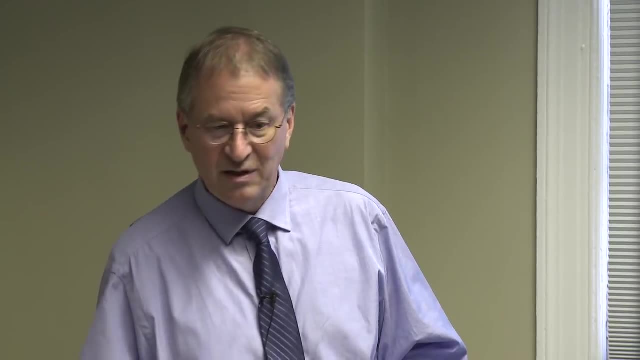 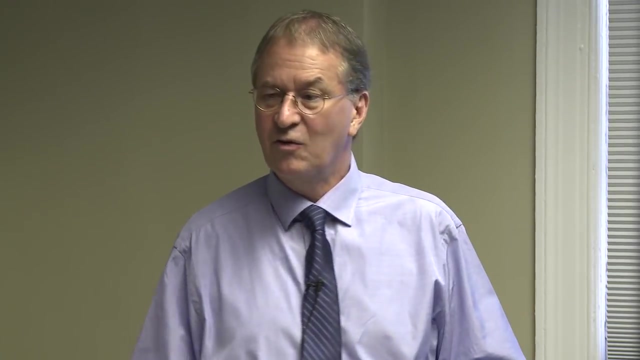 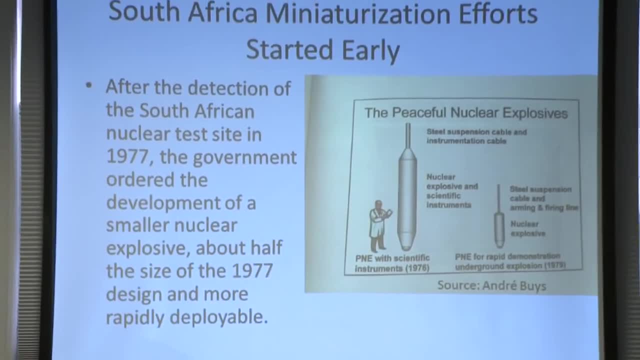 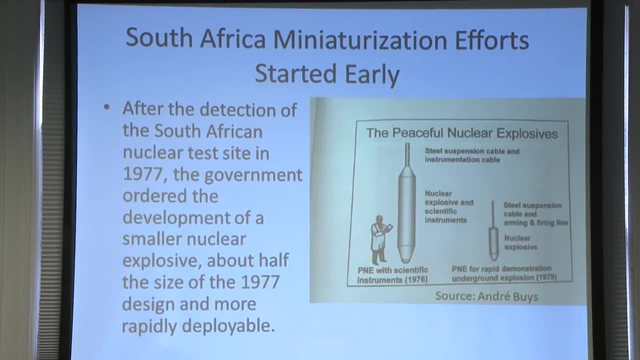 In 1977, the Russians discovered a secret South African nuclear test site and I mentioned they had a gun type In 1977, they didn't have enough weapon or highly enriched training for a bomb. That was in 1978 when they did Tickling the Tail of the Dragon. 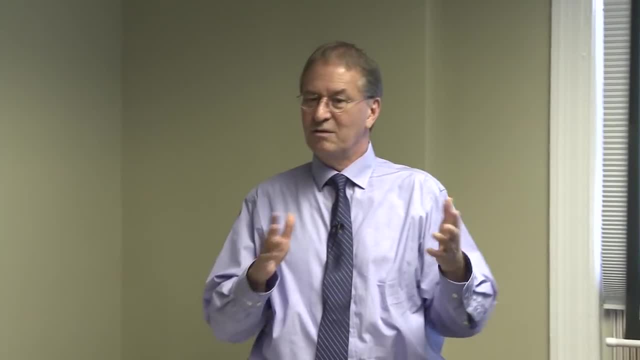 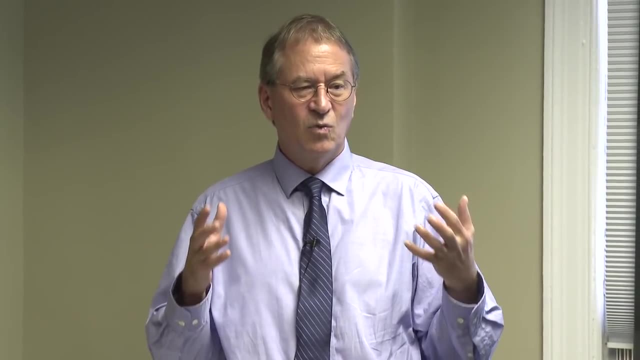 They didn't even need a nuclear test site, but nonetheless they built it because of this idea of building a lot of things in parallel. In 1977, they decided: why don't we just have a full-up mock-up of a nuclear explosion? 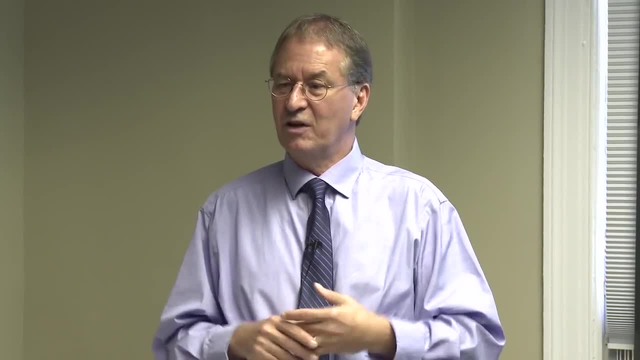 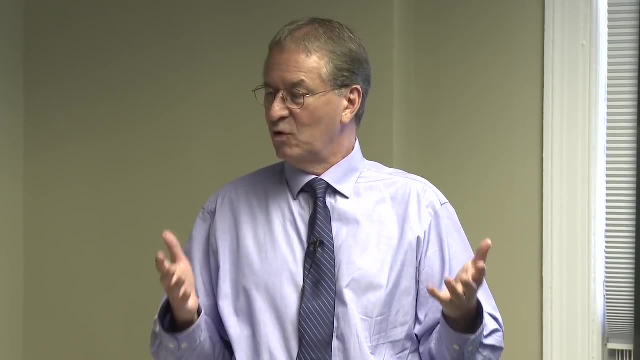 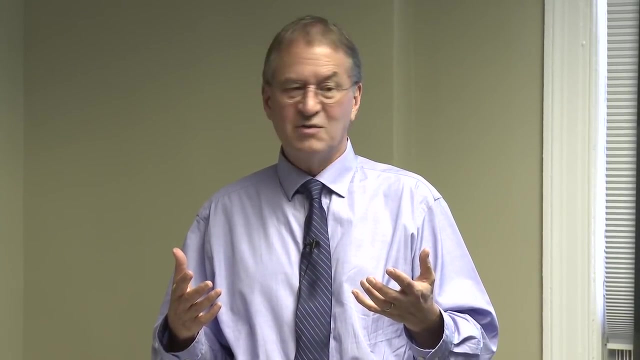 They designed a mock-up. They started putting everything out there and the Russians detected it and then told the Americans- and just an alarm went off worldwide- that South Africa was getting ready to test a nuclear weapon. It led to UN Security Council sanctions on South Africa. 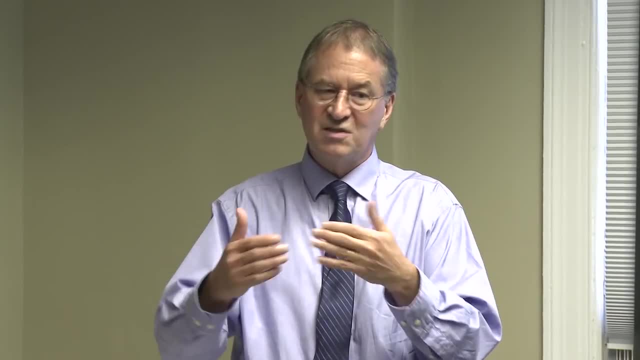 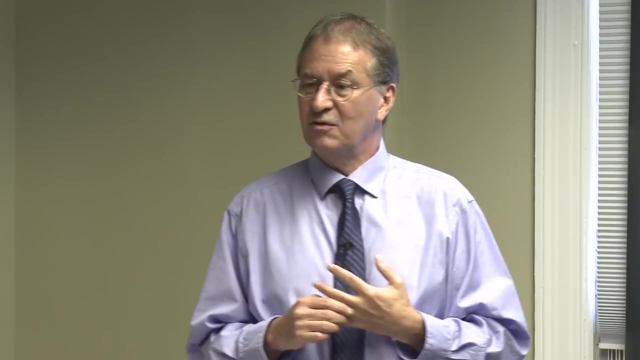 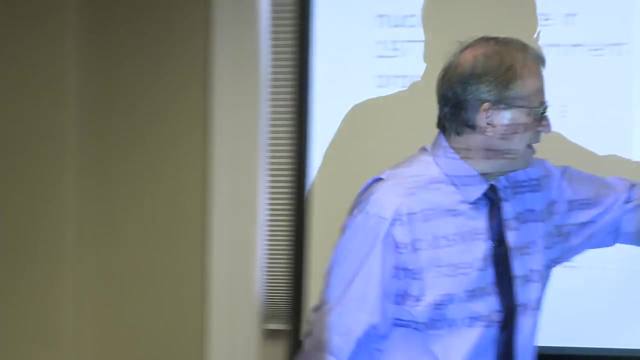 They had been in the works for a while, but the nuclear aspect tipped them into passing and a military embargo was placed on South Africa in the fall of 1977. This is a schematic. This was done by – he was in the South African program- a guy named Andre Baez. 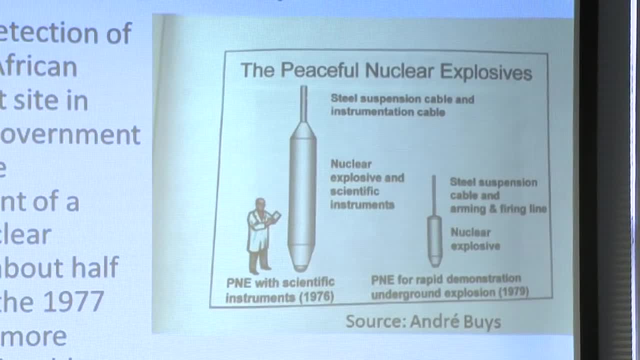 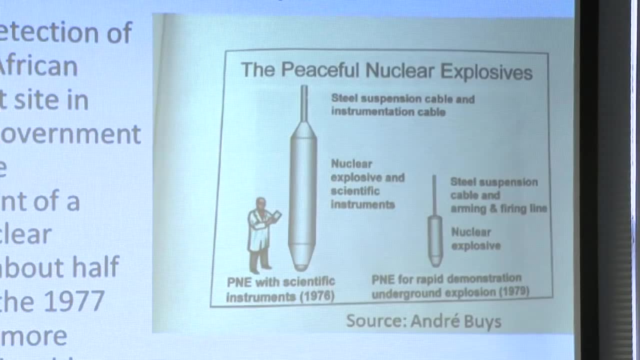 Andre Baez was in the South African program. He started in the early 1970s working on the development of a gun type device and he's been one of the more over-represented Open people once they've banned in their program and the big, long, cylindrical thing. 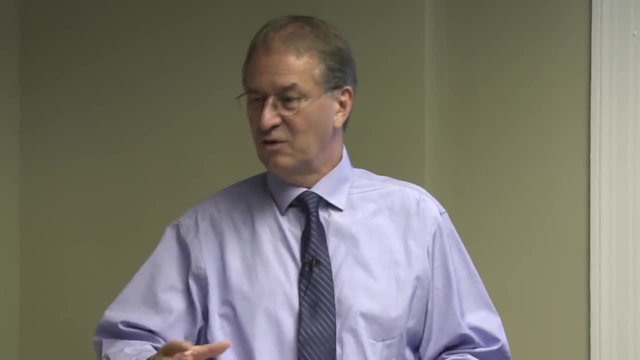 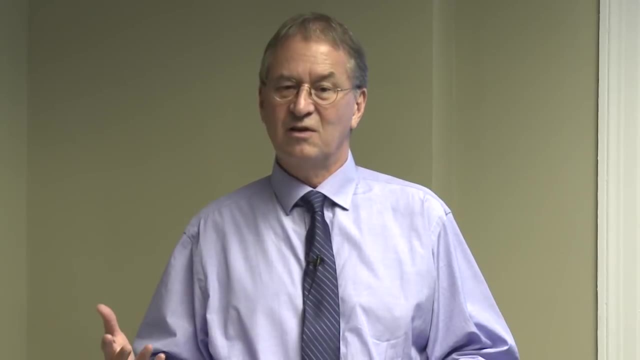 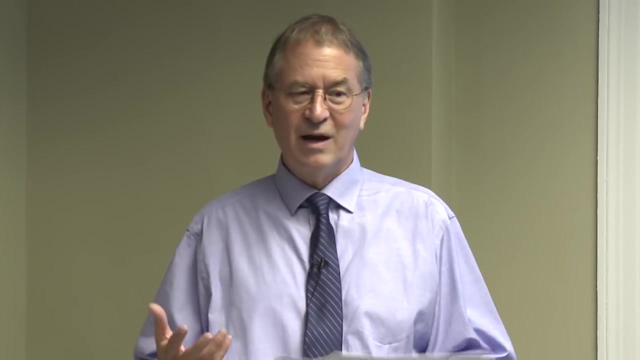 on the left is the package. they were going to put down this hole. It would have the bomb itself and then instrumentation because there was going to be scientific experiments. For a lot of the people in the program it was a peaceful nuclear explosive. They were going to learn all about nuclear explosions. 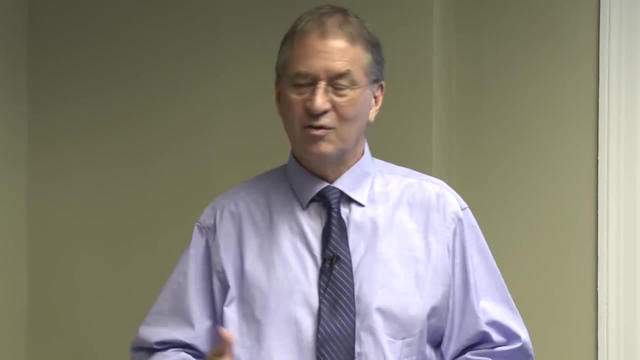 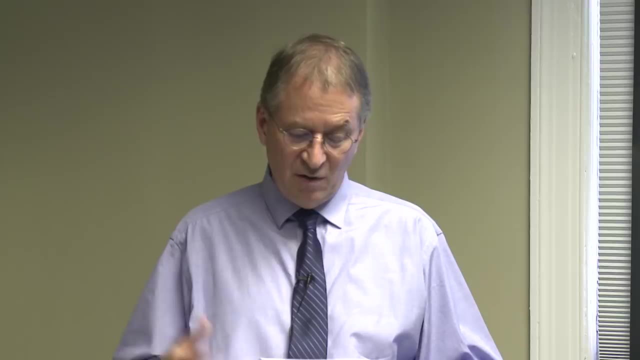 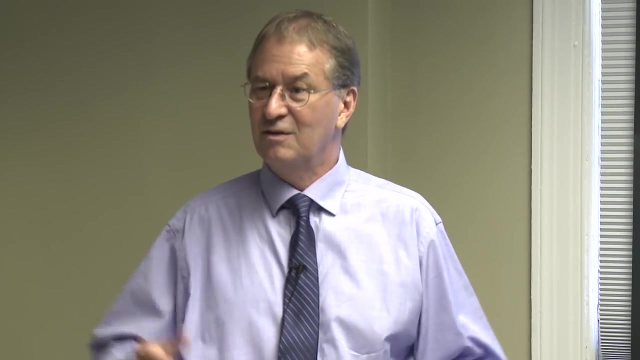 How Could you apply them to build a harbor or do mines In the back of the mine. it could be a weapon too, but as this colleague of mine represents, they weren't all looking to build nuclear weapons to deliver against the front-line. 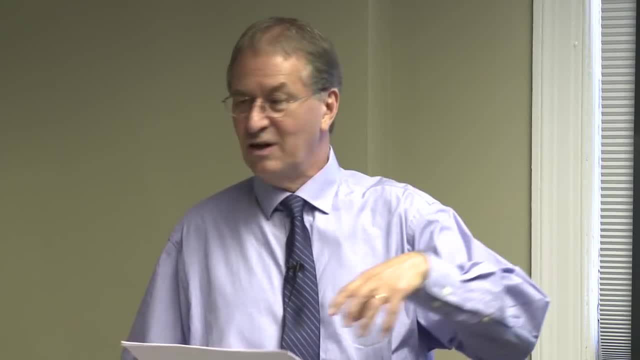 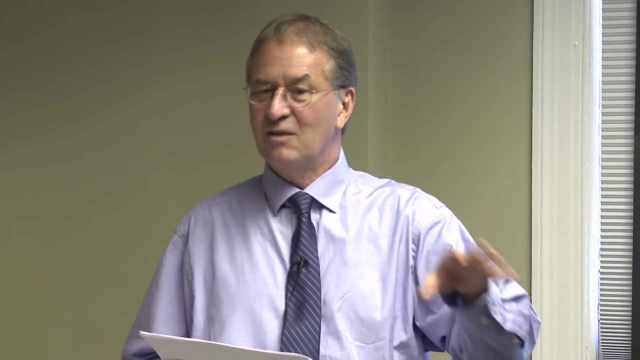 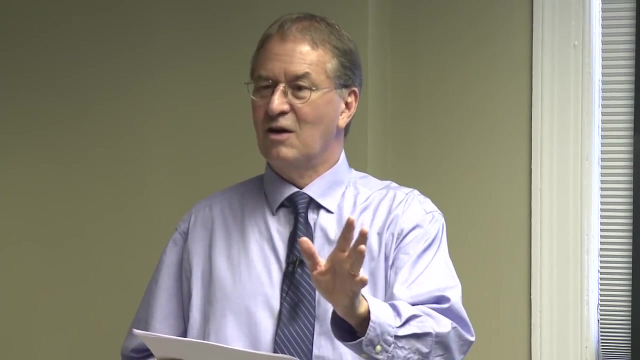 states, as they were called. It was a very hectic situation down there, with – again, you may not remember, There were 50,000 Cuban troops in Angola by this time. There was an active war going on. You had, in a sense, Russia surrogates on one side and you had South Africa on the other. 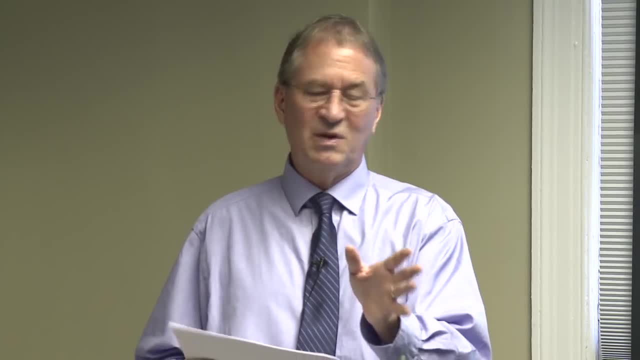 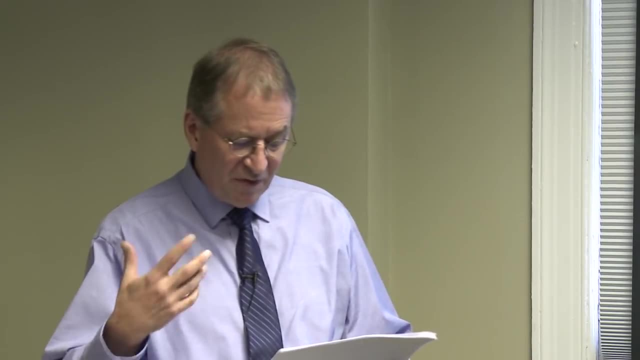 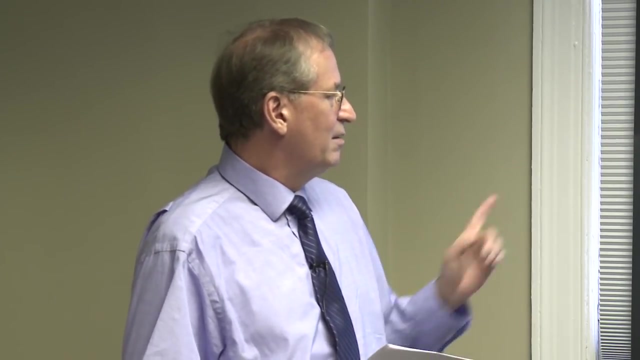 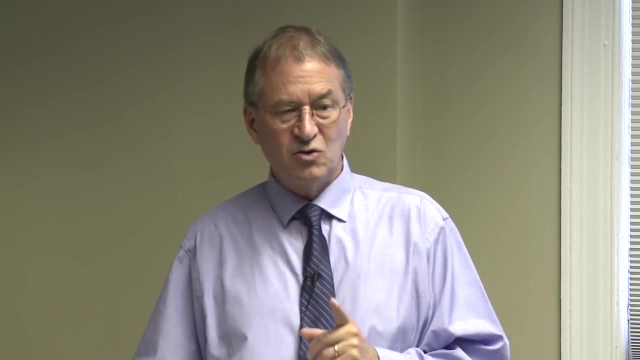 where the US was behind it but was losing interest because of apartheid policies. Even with that, a lot of these people in the program were not that enthusiastic about it. When they were confronted with the public condemnation and the Security Council were not in favor of the resolution, they made a decision. 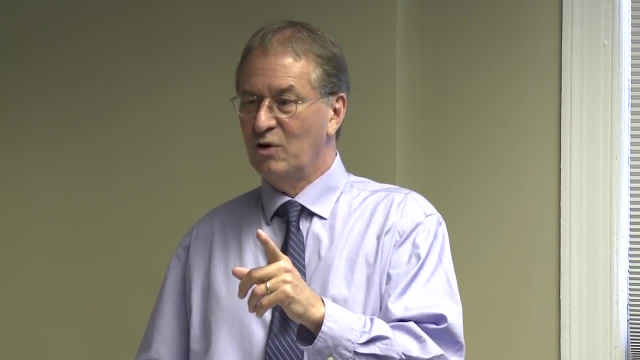 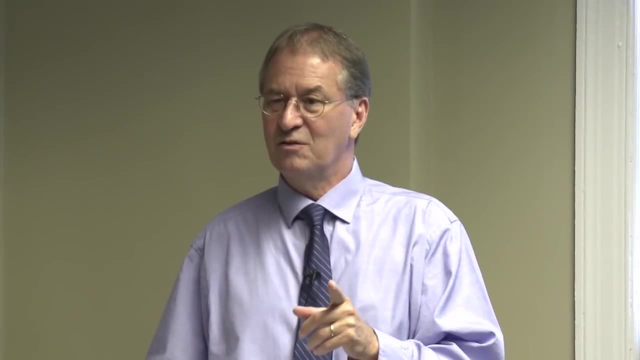 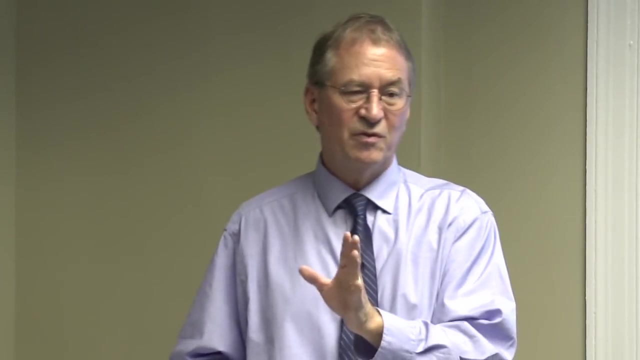 They said: look, we're going to go down the route of nuclear weapons because we've been put in a corner. They are putting sanctions on us and those will stay until apartheid is gone. They've started making a demand that South Africa sign the nonproliferation treaty. But if they even signed it, the sanctions wouldn't disappear because of apartheid. This is an apartheid regime. It basically said: look, Why not build nuclear weapons? Because for us to agree to these conditions mean we'd have to end our regime as they envisioned. 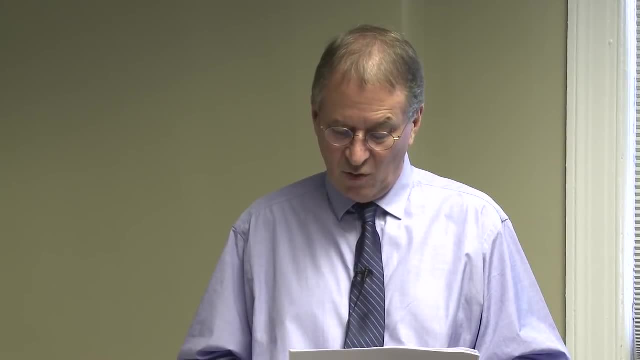 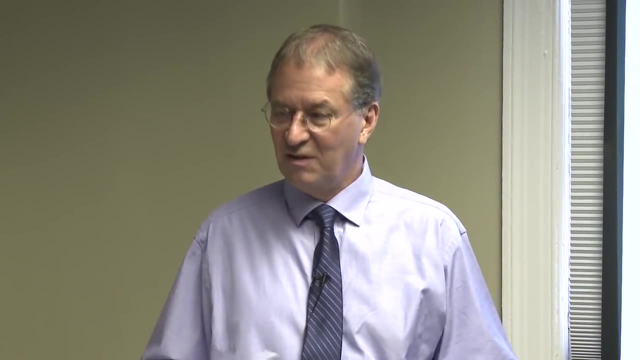 it In 1977, the apartheid regime was very strong and there wasn't a lot of dissent within it. They decided from one day to the next that they're going to miniaturize, which means they're thinking of it as a weapon. 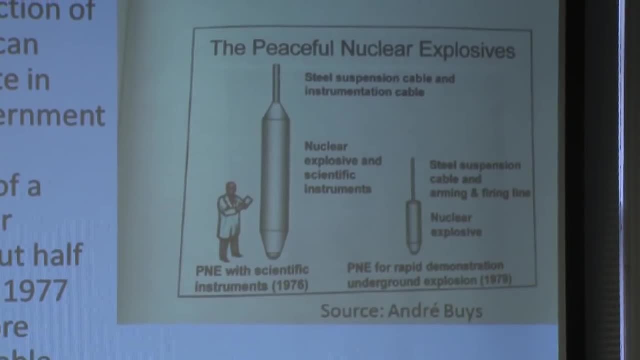 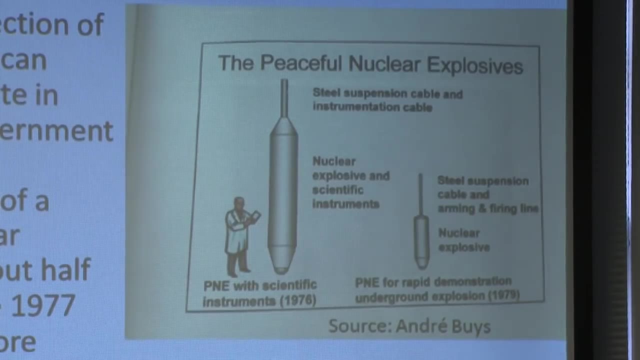 When they designed a P&E. in fact, their first device was a P&E. Well, they called it P&E. It was a nuclear explosive device designed to go down a shaft. It had been reduced in size from here to there. The design itself was about half as big. 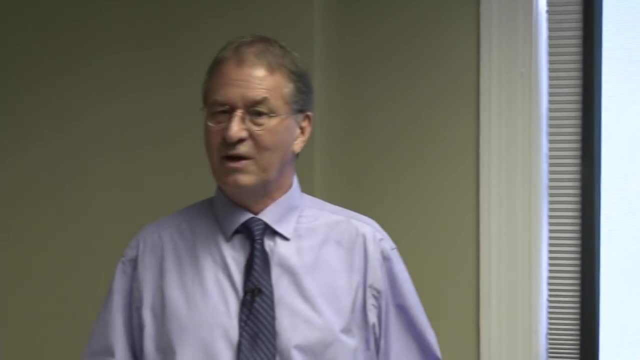 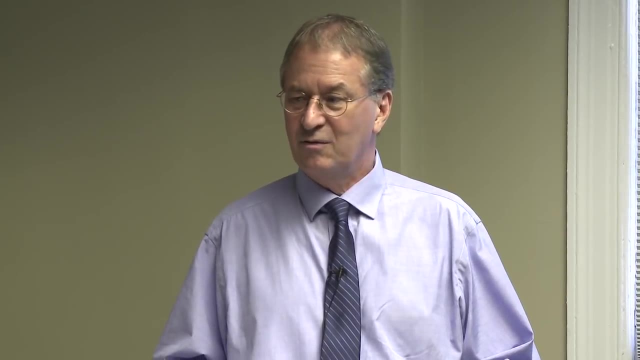 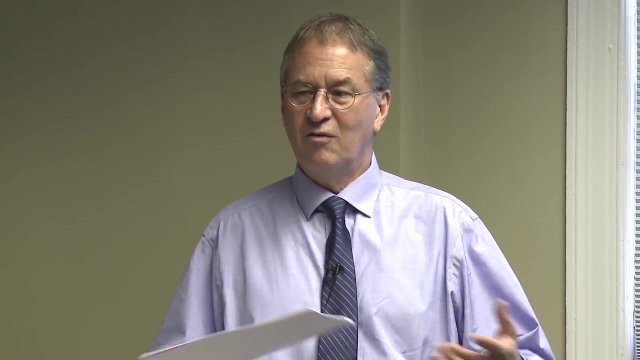 The warhead itself or the nuclear explosive itself was about half as big. It could be deployed quickly, which means if they were going to test it, it was to send a political signal. They evolved a very elaborate kind of convoluted nuclear strategy. They knew they couldn't take on the Soviet Union. They viewed that the Soviet Union had nuclear weapons on ships offshore. They were worried that with 50,000 Cuban troops, Russian support, that they could lose the war. Then they would use this nuclear weapon. 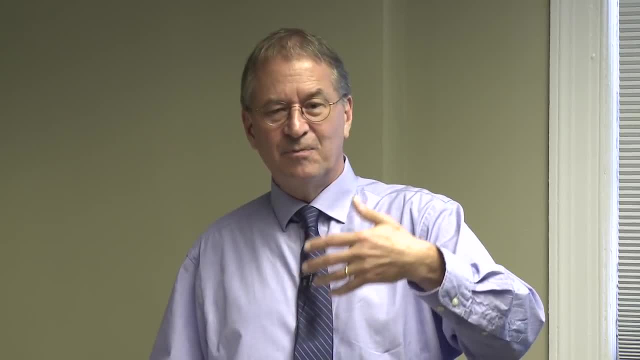 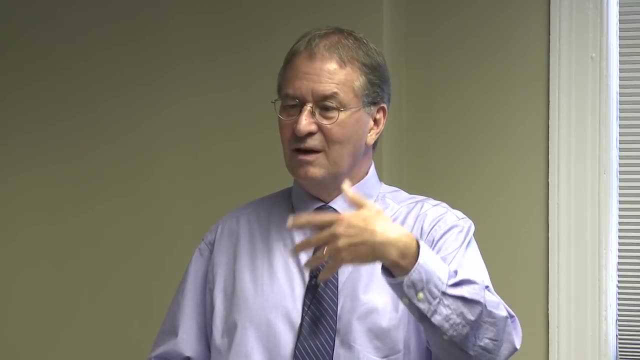 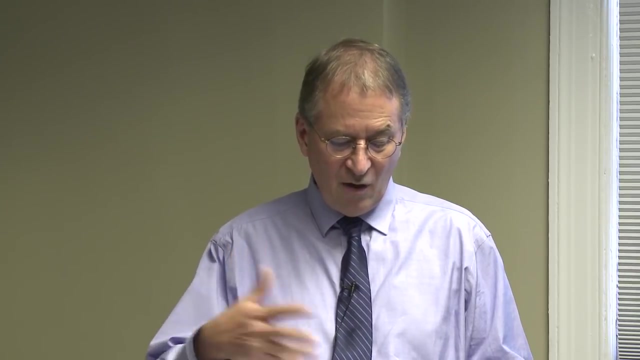 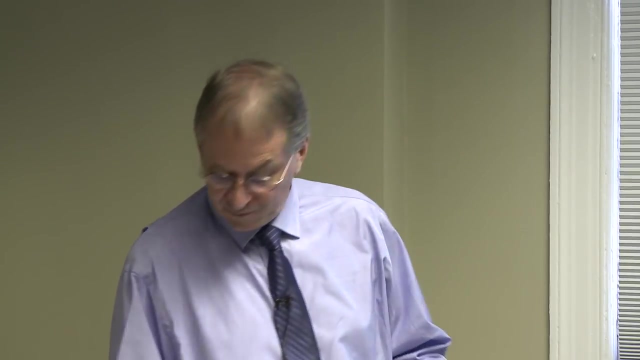 They called it back-to-the-wall strategy, that they could use it to not deter the attack but force the United States to help them. Yeah, They would step in and confront the Soviet-inspired advance Throughout their program. that was the basic motivation. 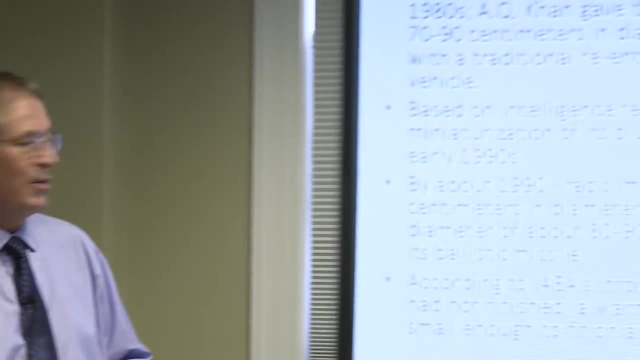 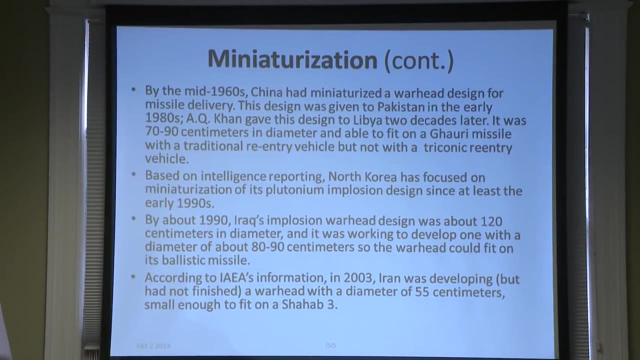 Stepping back a little bit. talk about miniaturization in general, and then I'll come back to South Africa. The states have gone about the miniaturization differently. China after their first test in 1964, two years later they were able to miniaturize. 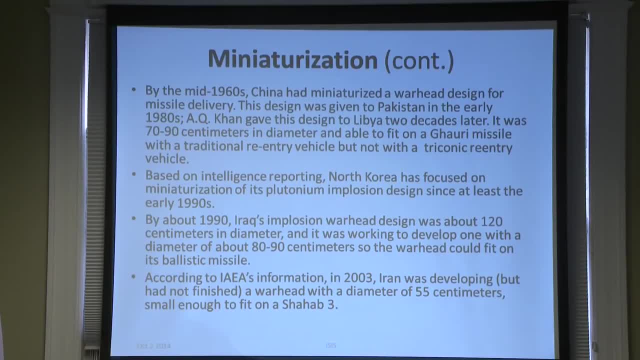 for a missile. In fact shot the missile across China, detonated it above the Lop Nur test site, which also shows you the safety considerations given to these things back then. But again, in two years they were able to miniaturize for a warhead. 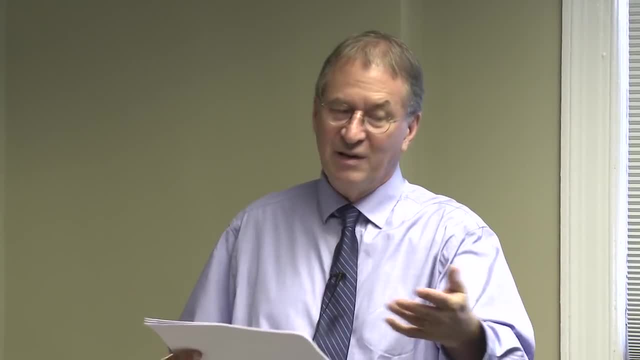 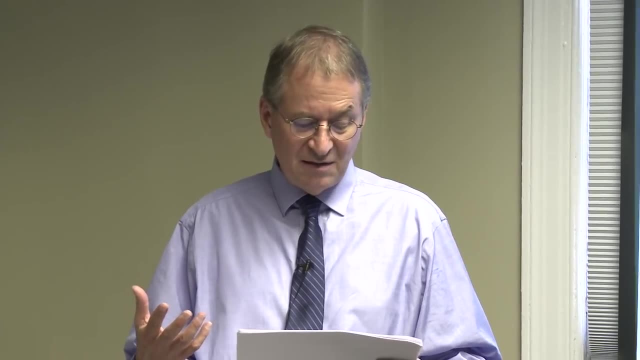 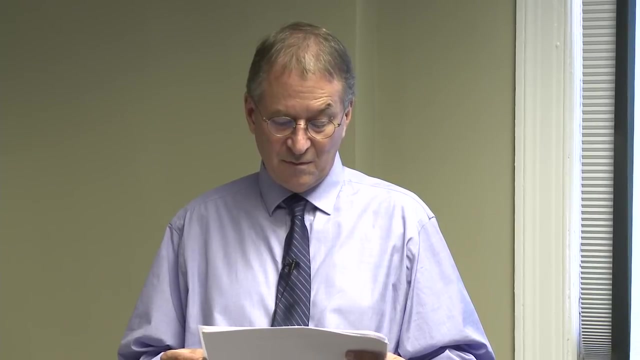 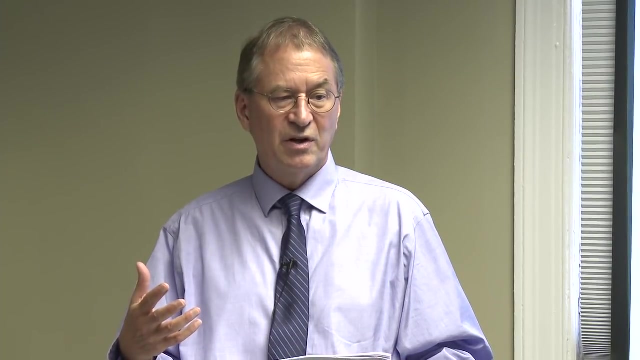 That was the design given to Pakistan. We think it probably ended up in North Korea too at some point. Just to give you some sense of these dimensions, that design is about 70 to 90 centimeters in diameter. In comparison, this Iraqi design that they were working on with 15 kilograms is about 120 centimeters across. When they launched a crash program in 1990 after their invasion of Kuwait, they were trying to get it down to about 70, so 80 to 90 centimeters, And it failed by the time the war started in early 1991.. 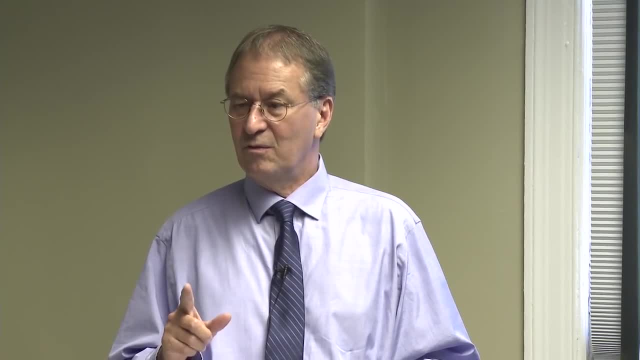 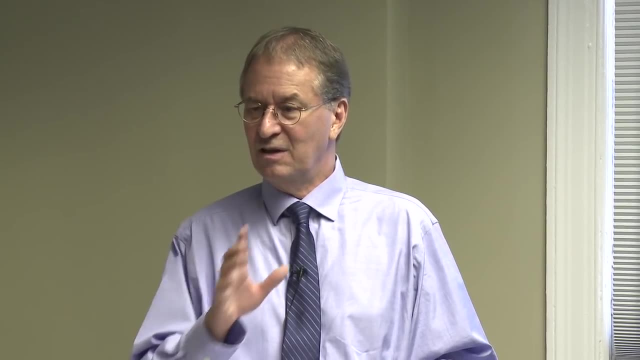 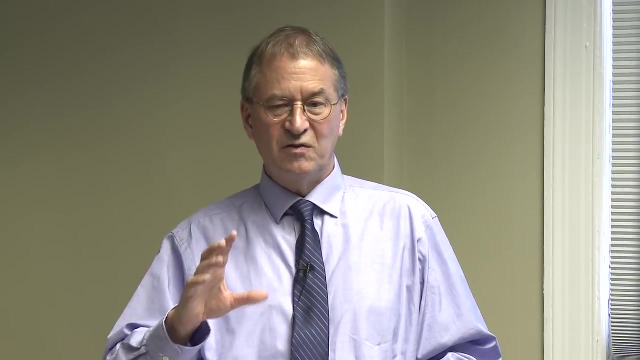 In the case of Iran, they're using a derivative of a North Korean missile, but the warhead is—the reentry vehicle has changed because, again, the Gowri is North Korean, The Shahid III is ultimately a North Korean design, But the reentry vehicle has changed and they need a smaller warhead and the warhead, the. 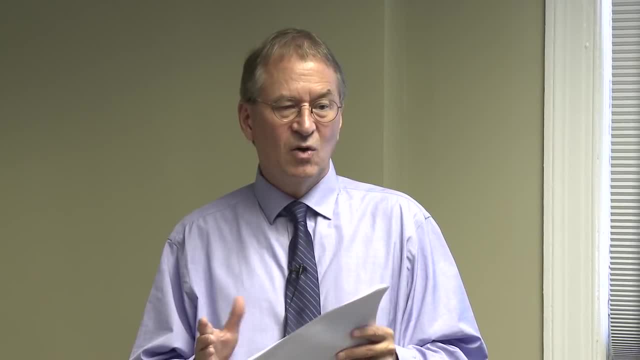 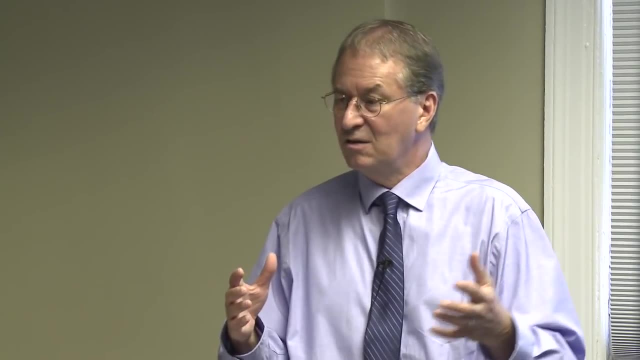 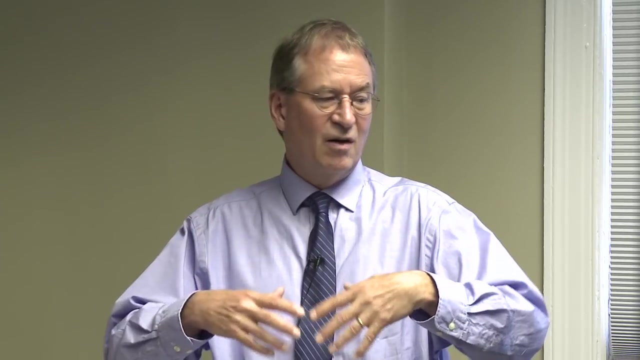 IA thinks Iran was working on In 2003,. it was about 55 centimeters in diameter. The IA isn't claiming they succeeded by any means, but it was a very small design that Iran was working on. That's what a lot of these allegations are: attempts to get Iran to explain away this. 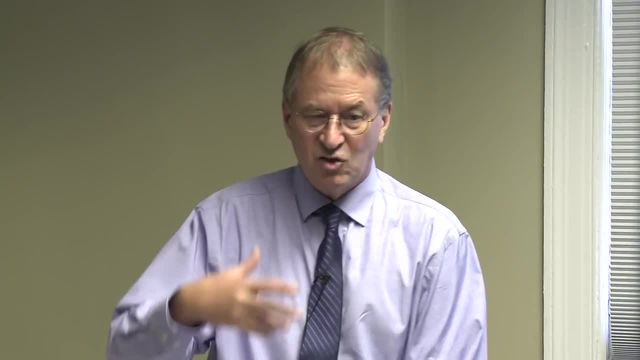 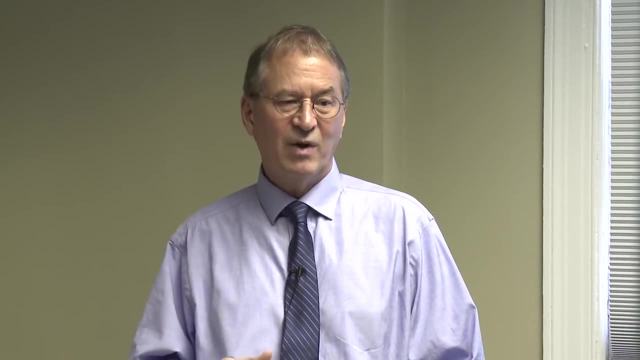 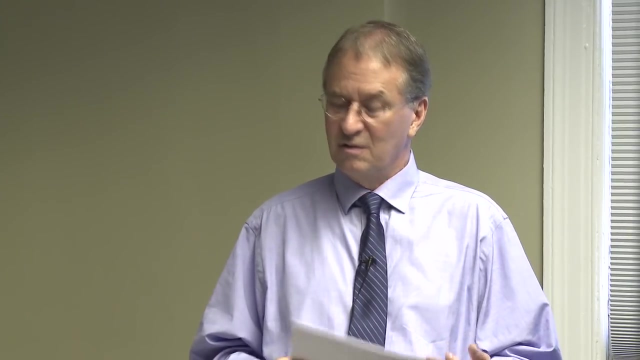 pretty solid intelligence information. It shows that, if it's true, It's true that long before Iran could have thought of producing weapon-grade uranium, it was designing a warhead to fit on its principal delivery system, the Shahid III, and taking the steps necessary to do that. 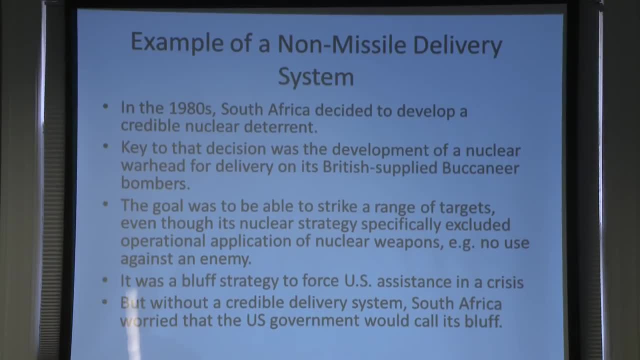 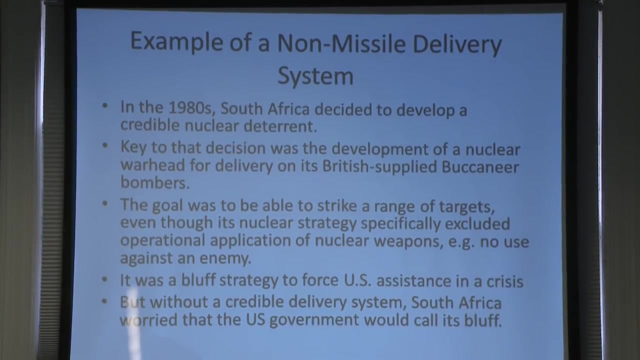 South Africa didn't have the greatest military aircraft. They're under a military embargo. They're largely depending on aircraft they bought early. They had something from the British. The British called it a buccaneer bomber and that became their nuclear delivery aircraft. 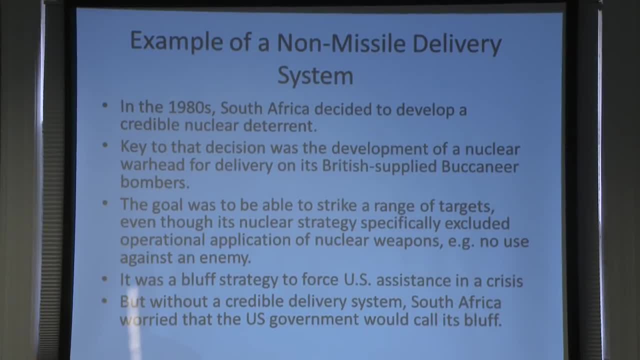 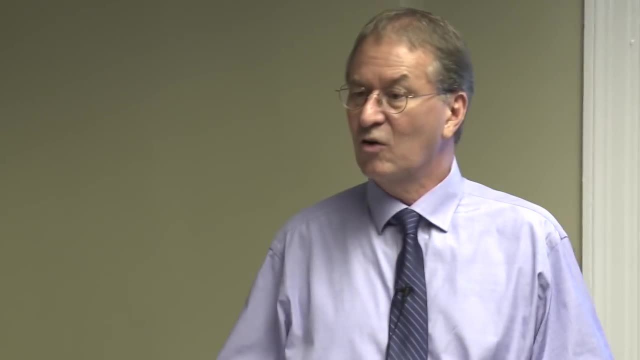 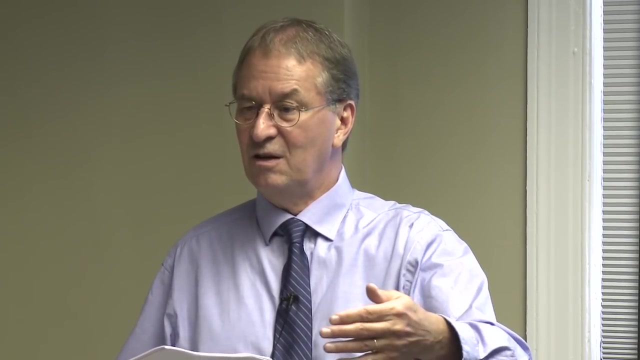 It had been so for the British. They had to think through how do you develop a system for this, a fairly old aircraft that's not going to penetrate Soviet air defenses that were in place or were being put in place in the front-line states like Angola. 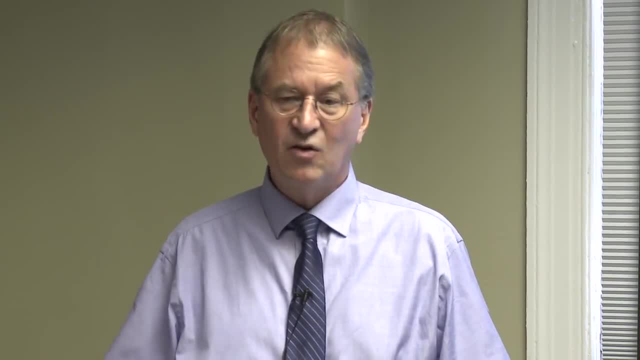 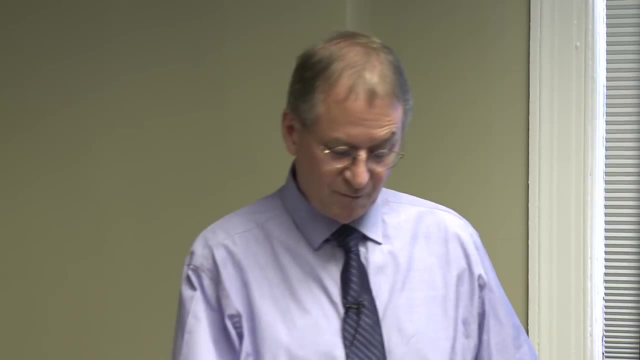 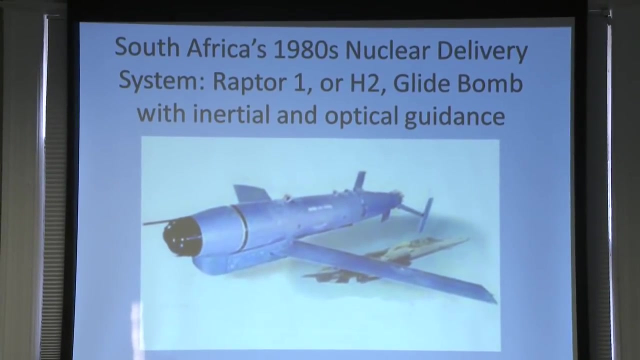 What do you do? What they did? They decided to develop a standoff weapon and put a nuclear weapon on that. Here's a picture of it. It's called the Raptor Wanderer H2 Glide Bomb. It was developed for conventional use. 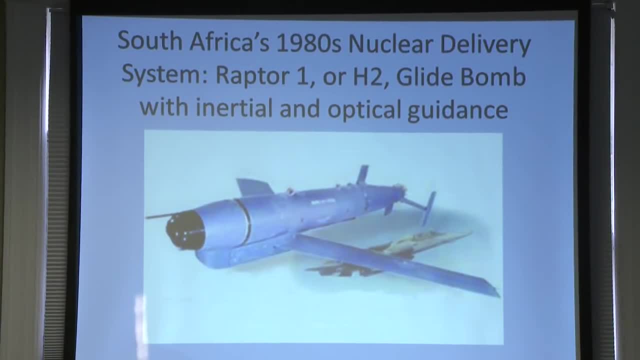 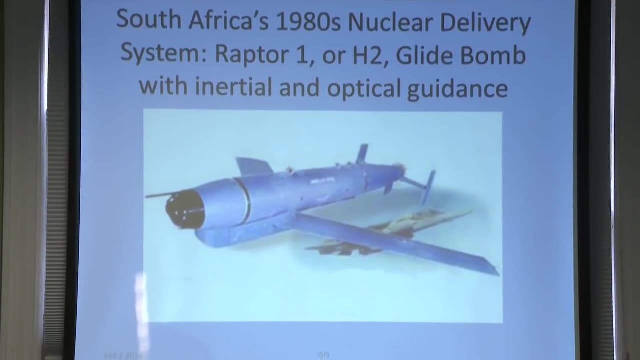 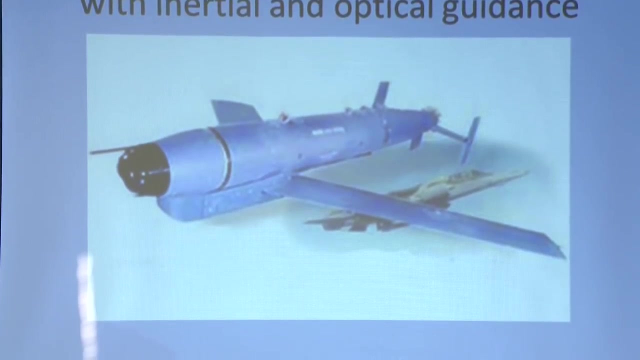 It actually has video guidance so it can relay back pictures to the commanding aircraft that's fired it. Then it can be directed at a target. They demonstrated it in a battle and destroyed a bridge with it in Angola. Underneath that, it was their primary delivery vehicle for nuclear weapons. 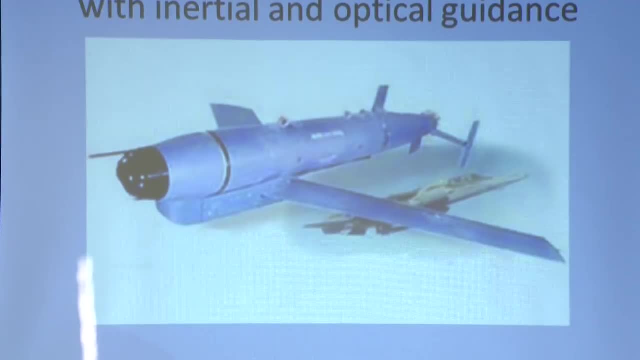 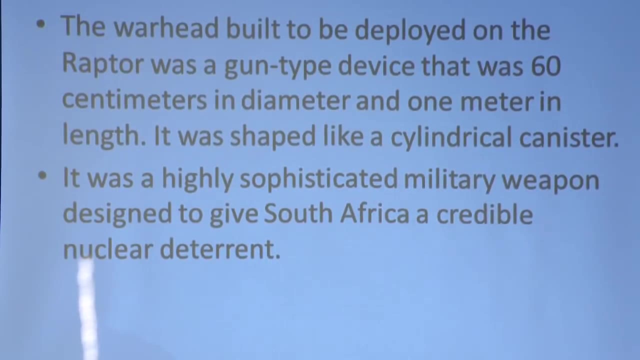 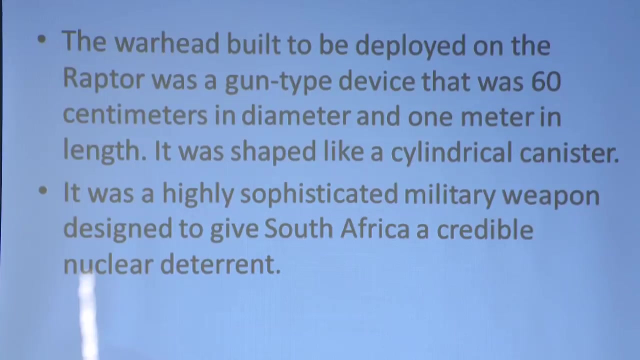 The way it looks when you put it on. a—well, the design of this weapon. it was about 60 centimeters in diameter and one meter in length. It looked like a canister that would then fit into this glide bomb. Again, it was very sophisticated. 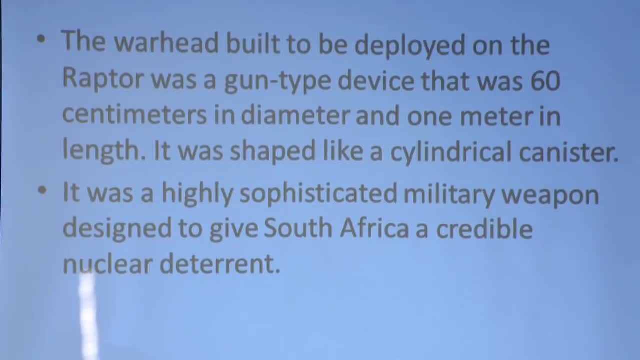 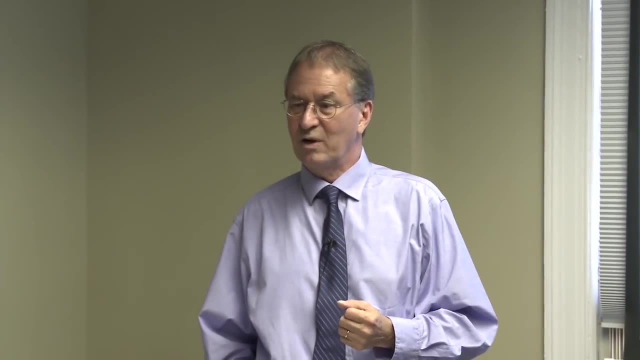 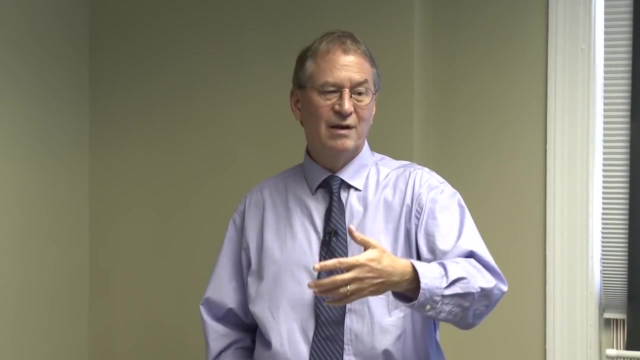 It went through a tremendous amount of testing. It was like a Cadillac model of a gun-type device. That's the way people have described it, for example, people in the IA who investigated the program in great detail. Again, no advancements in the—we call it- the physics package, the core. 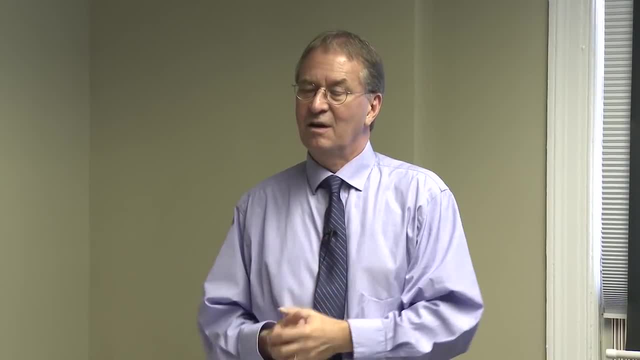 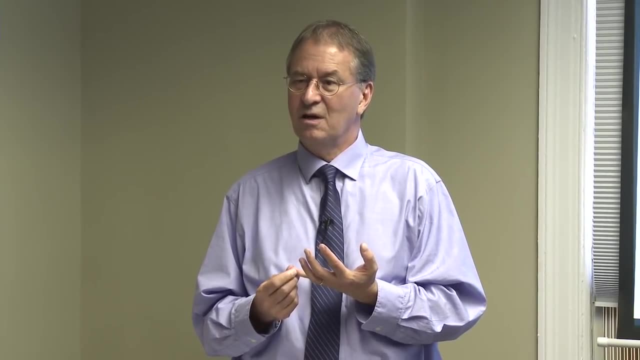 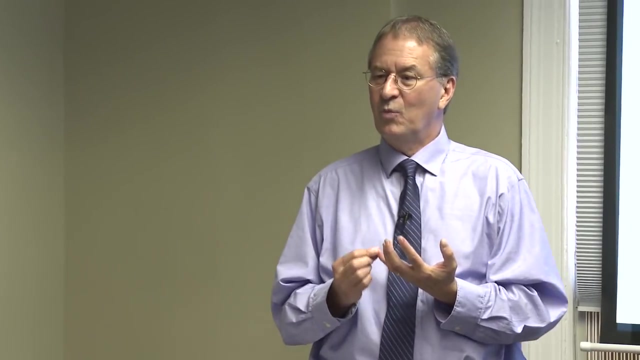 They didn't use more sophisticated techniques to assemble the highly enriched geranium. The only thing they did that was unexpected was they didn't have—they didn't have- a neutron initiator. I don't know all the reasons why, but if you don't have a neutron initiator on a gun-type, 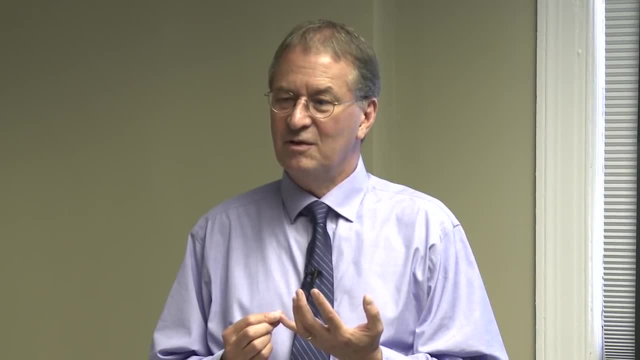 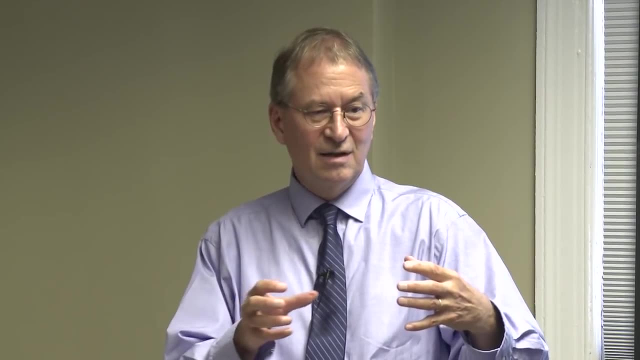 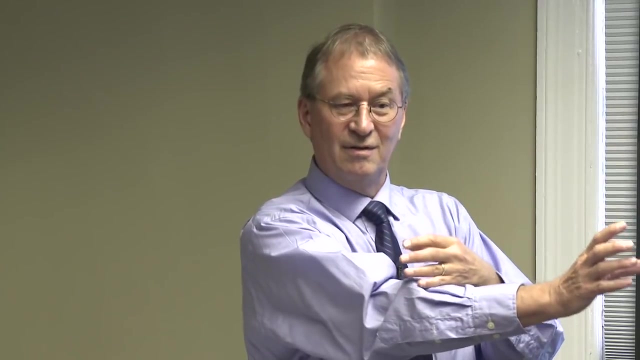 device. you risk that this plug is coming down the barrel like a naval gun and it hits the fissile material, the highly enriched geranium, at the end and it just keeps going. The only reason I say this is because there are other students who have done it, but we 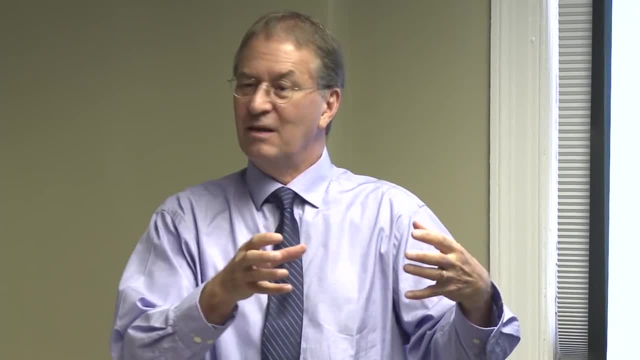 were a 0a-ẻ business before, it was fine. I admit that they're all good. okay, All right, Thank you. Thank you, Bill. Thank you, I am going to go to the next question that I'm going to um rather quickly and I яa. 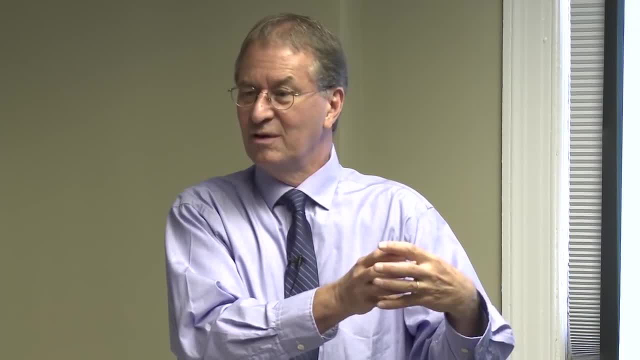 passe et al. Sure, sir, Sure. The question for no one, uh, John Caniley, is if the issuance of the Muscat pharmaceutical producer, if you are just going to, just went through that with the Jenkins method and instead of adding at all the treatment that the prescription or the 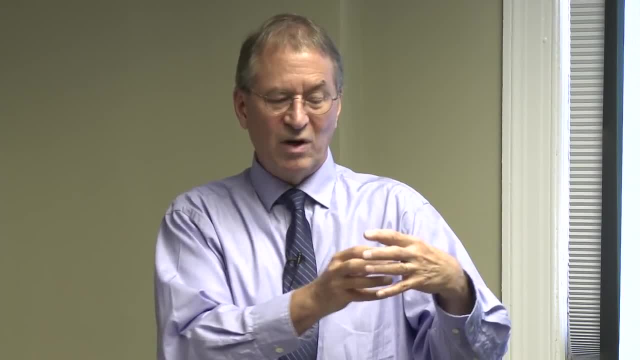 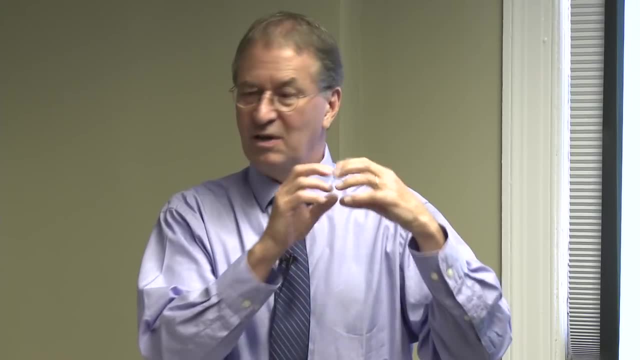 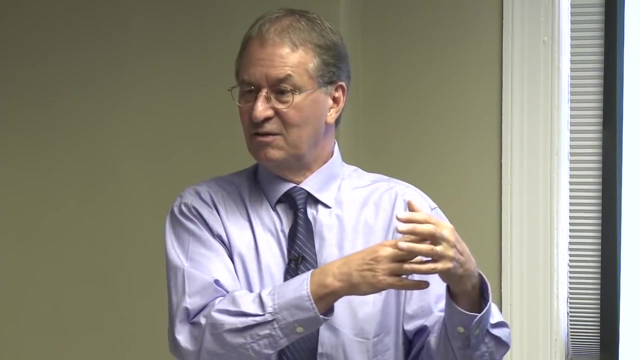 prescription, else that was there on the outside, all the legislation that was there, non-existent. Yes, If it initiates the nuclear explosion will happen so quickly that explosion will happen before it can hit the back. In the South African case they didn't want a neutron initiator, so they had to design. 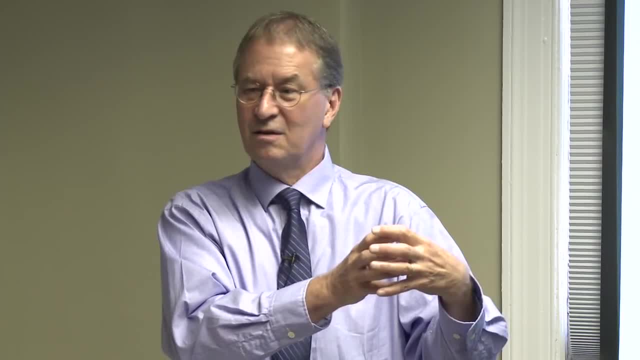 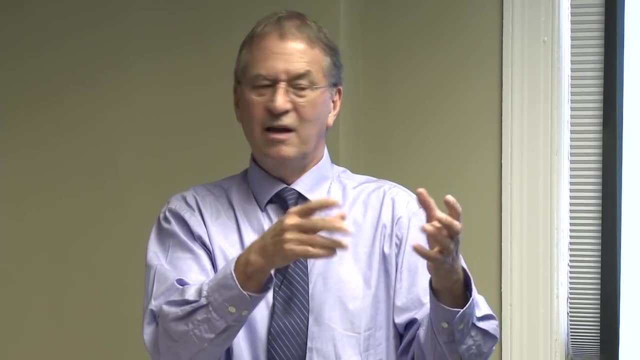 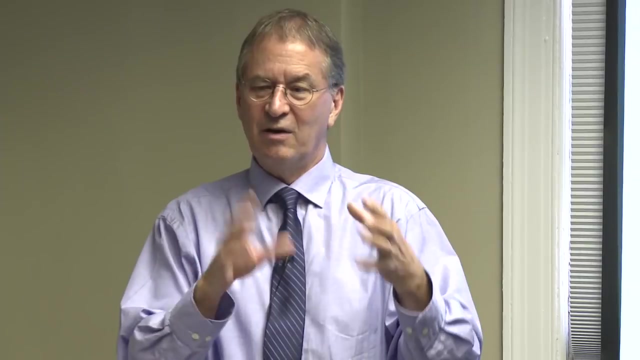 it so that the plug would actually be caught and not bounce back in the end and it would sit there. There's a mistake in what I gave you. in the South African study I think it talks about in microseconds, a neutron from outer space will set off the chain reaction. It's actually milliseconds, if that matters to you, but we should correct that mistake. They designed it so this plug, fired from in a sense like a naval gun, is caught at the end, Then a neutron produced in outer space will start the chain reaction. It avoided having to build this very complicated neutron initiator, which, at the time, typically required renewal every year. They wanted a design that didn't require that. The homework assignment is: how do you keep it from bouncing back, Because if it hits, it's not going to just stop. 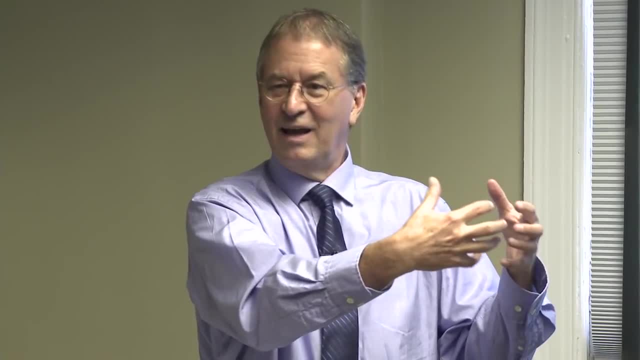 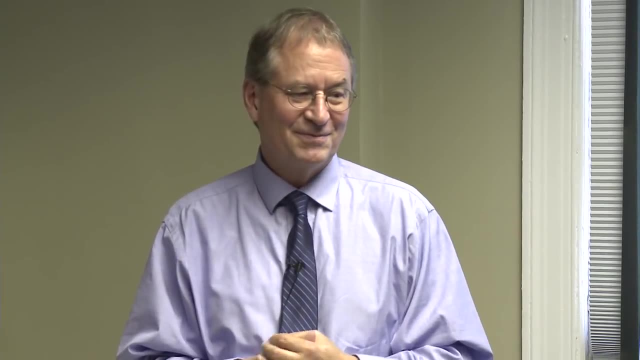 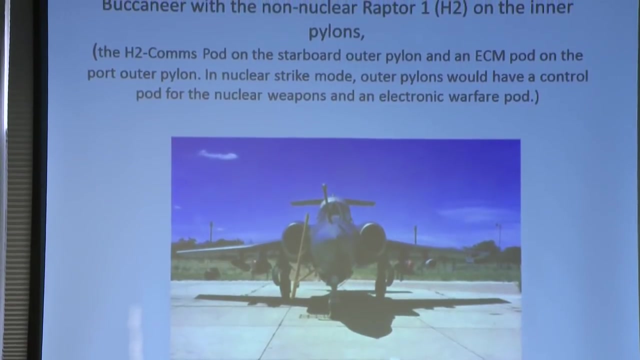 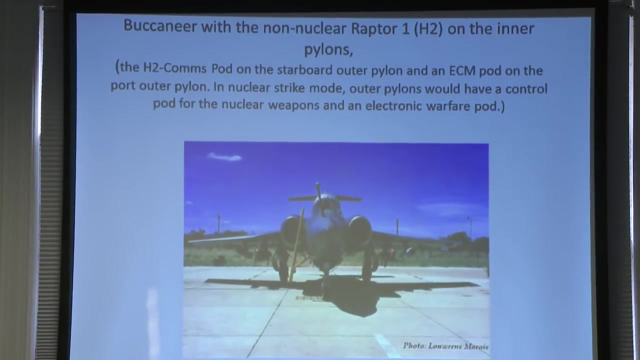 There's got to be a massive end, but how do you stop it from bouncing back? That's your homework assignment. Here's the buccaneer bomber. It's a little hard to see this, but the two red-tipped objects are the H2, so if the wings fold in and it's in a tube, they can bounce back. It's a little hard to see this, but the two red-tipped objects are the H2, so if the wings fold in and it's in a tube, they can bounce back. 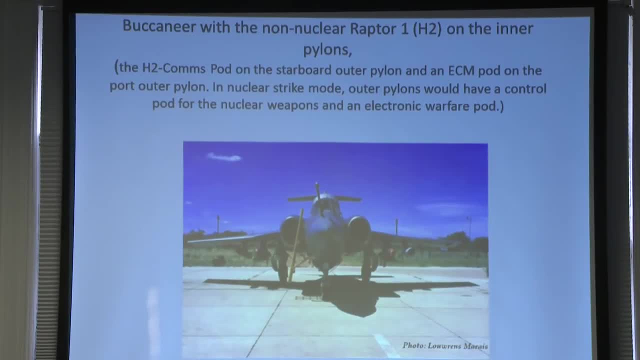 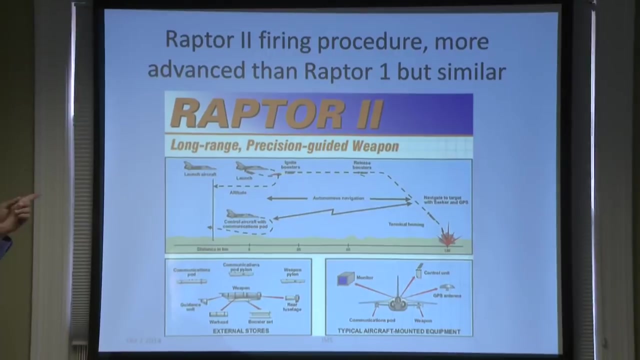 It's a little hard to see this, but the two red-tipped objects are the H2, so if the wings fold in and it's in a tube they can bounce back. Then in a nuclear strike mode the outer pylons would have a control pod for the nuclear weapons. 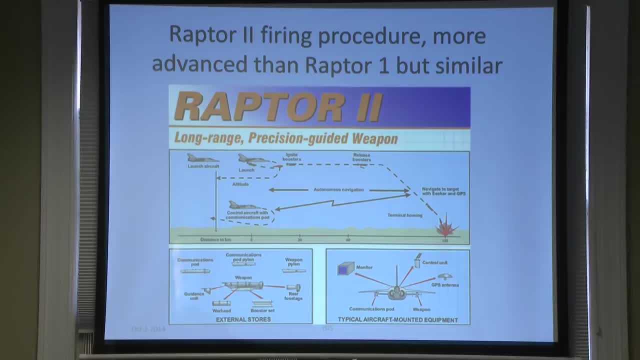 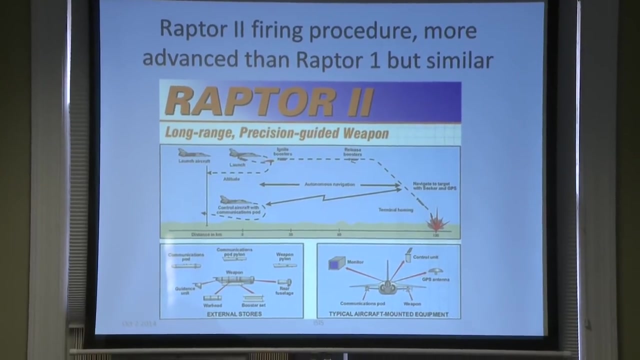 and an electronic-warfare pod. The idea of it was to ‑‑. this is for a later model, but you can fire in a stand-off and you can be controlling it as it goes along and getting information back from the glide bomb. But I'll leave this. 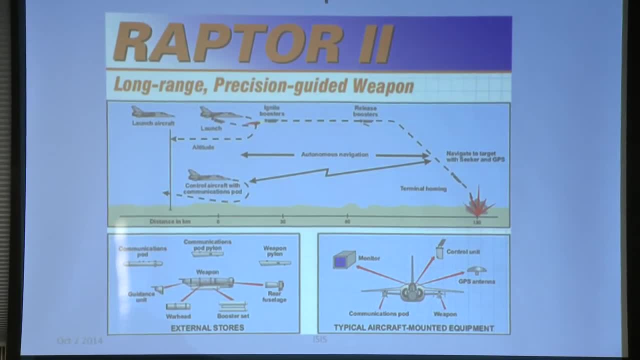 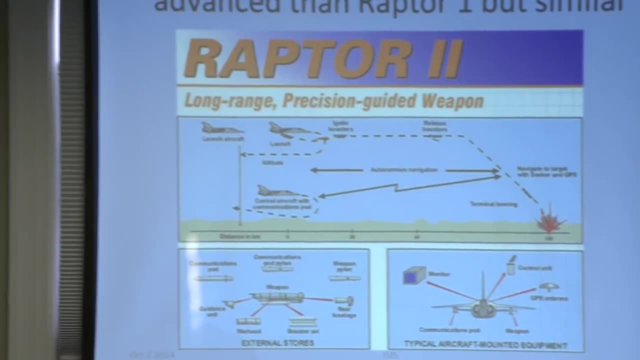 When you get the slides you can take a closer look at it if you're interested, But it worked for them. By the end of the program they had also worked out a deal with Israel where they were acquiring a ballistic missile from Israel. 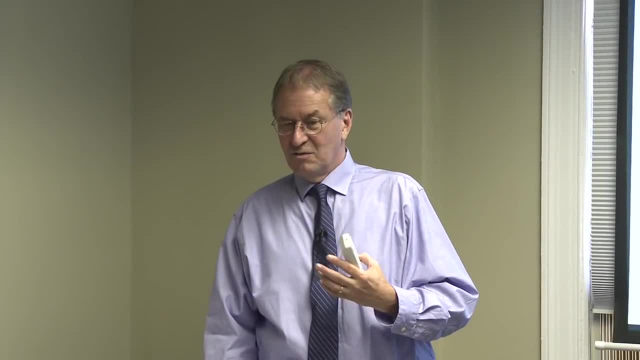 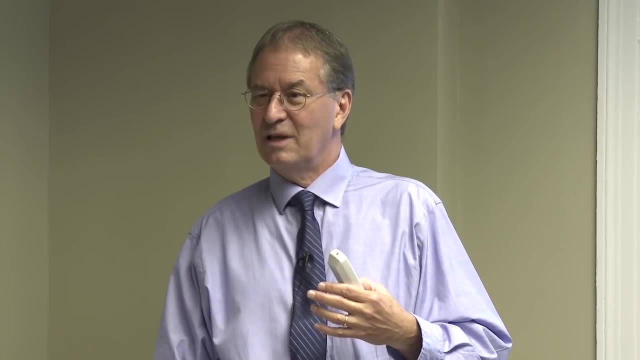 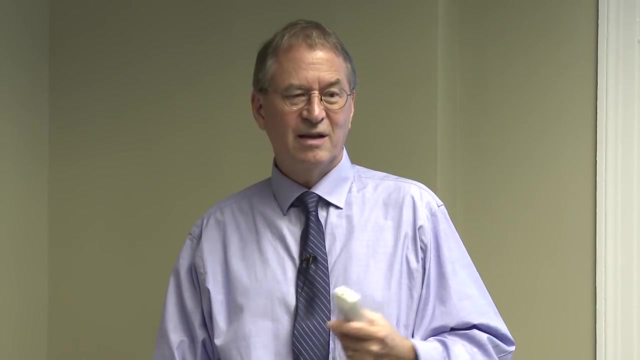 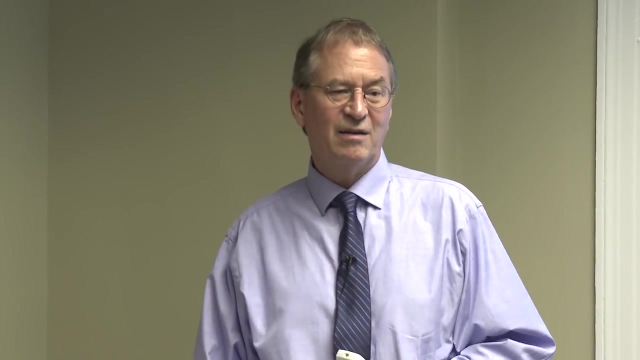 And just a little. I don't know if you follow what Congress does on sanctions with Iran In a very real way. Israel was like Iran to Congress in the 1980s And they took tremendous actions to try to block Israel from being able to provide the apartheid regime. 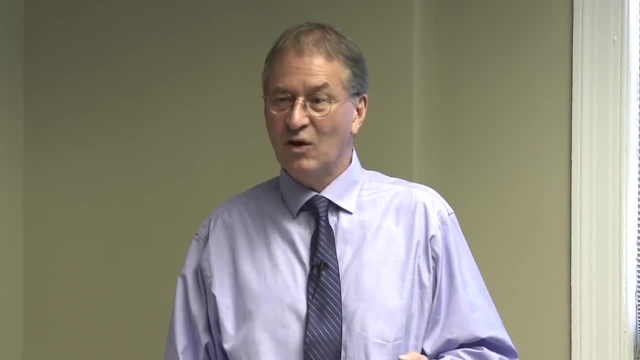 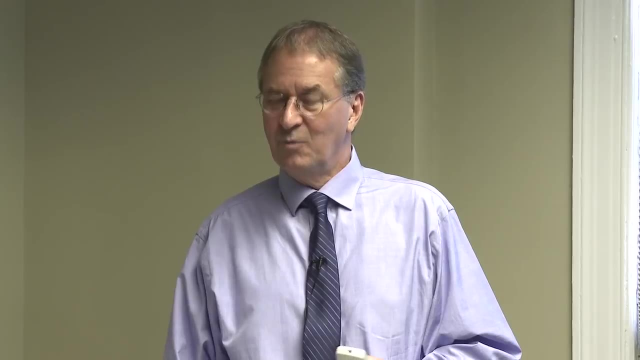 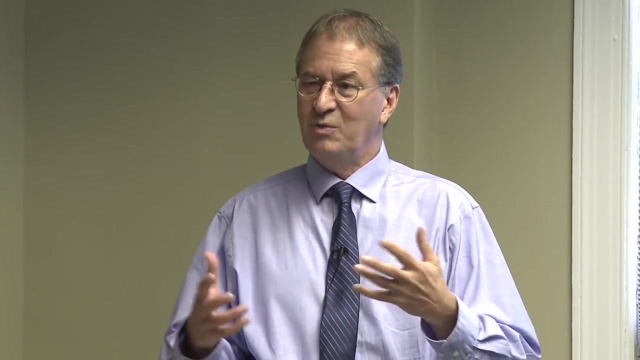 with armaments, in particular with ballistic missiles. They failed. Israel did provide the missiles And South Africa was building them, And by the late 80s they were building up a program to make the warhead for the ballistic missile, But they hadn't decided: would it be a gun type or an implosion type? 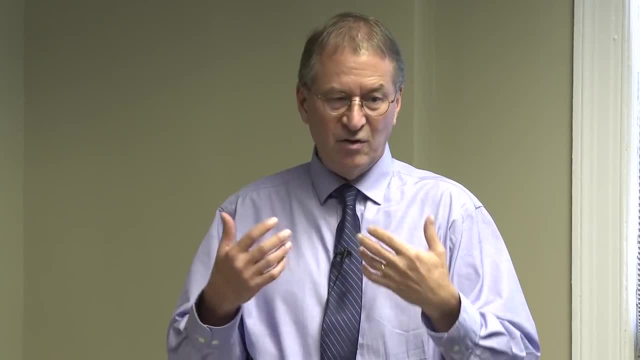 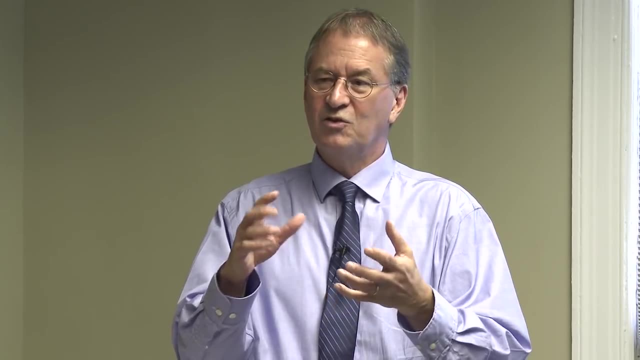 And they tended to, they told me. I've been down there and talked to many of them and they told me they favored a gun type, But they were facing an engineering problem, which is, I said, they want to make it, they want to make it safe, they want to make it secure against unauthorized use. 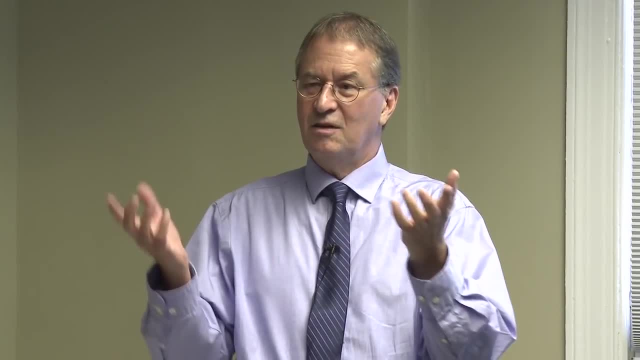 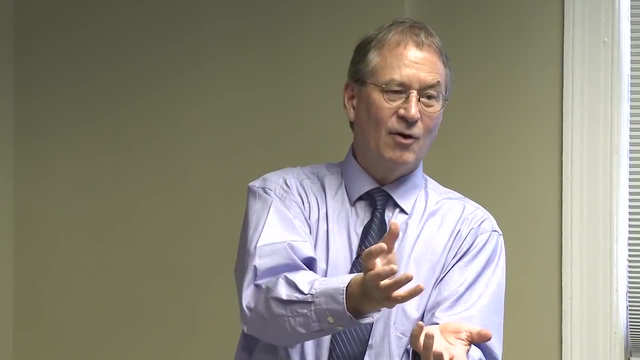 Well, one of the things you don't want to happen with a gun type device is it's a tube with highly enriched uranium in both ends. What if you tip it up and it just slides down? So again, it won't be a nuclear explosion, more than likely with that amount. 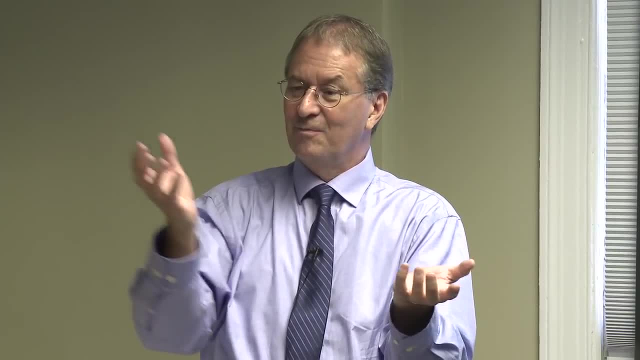 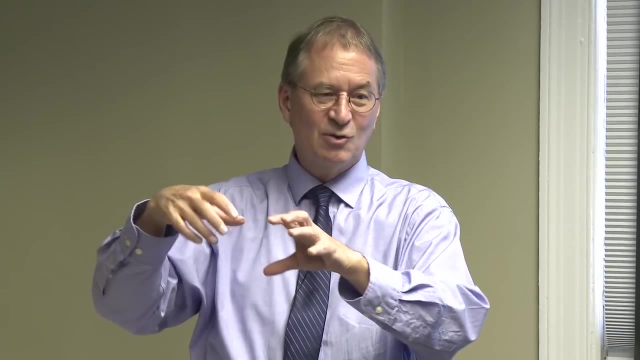 but it's going to be a critical reaction. So how do you keep the material from going all the way down? And again, I won't make this a homework assignment, but the solution for South Africa is: you have this tube and you have to make it safe. 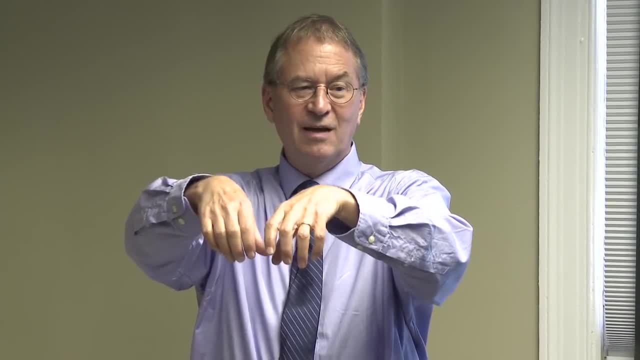 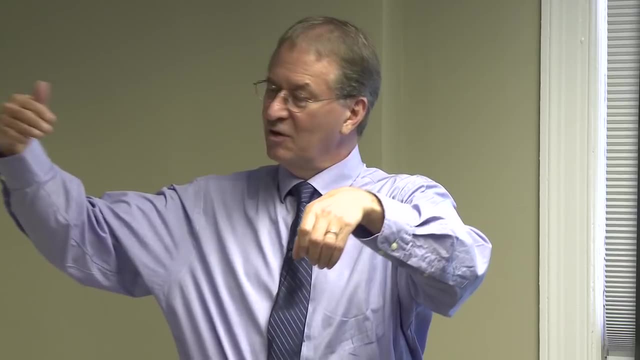 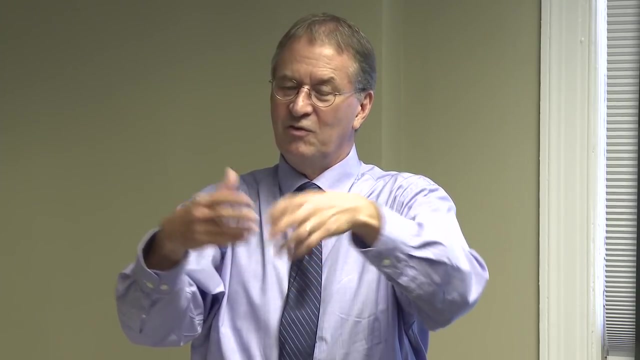 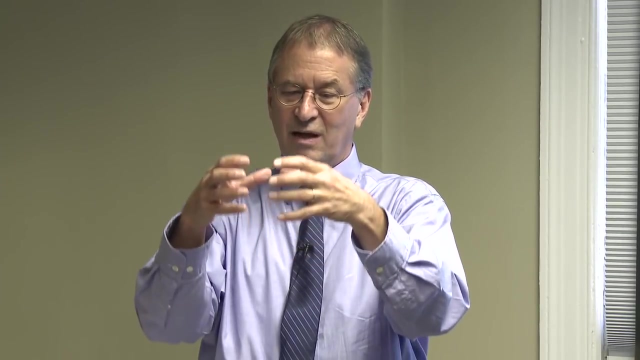 You cock it so that you split it in half and then you twist it so that you have overlapping edges, And so if it goes down it strikes the edge of the bottom tube and can't go any further. But if you're building a ballistic missile warhead, that's a problem, because you want to have everything symmetrical in a missile. because you don't want an off-center of the weight. It can cause the reentry vehicle to act funny. And so how do you build a safety device for the gun type? And they hadn't worked that out by the time of the end of the program. 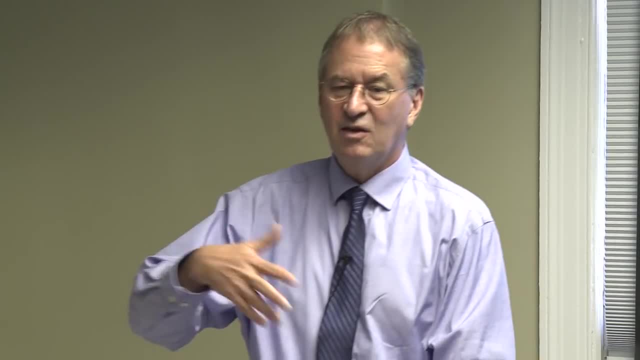 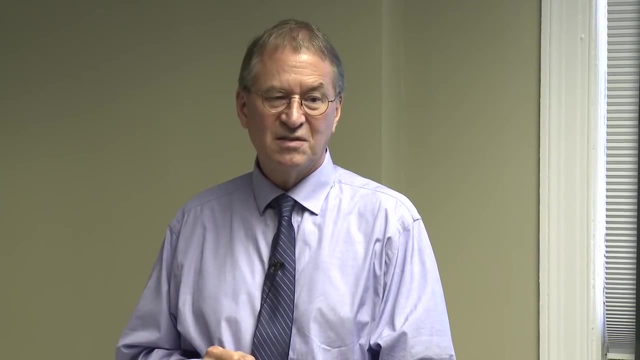 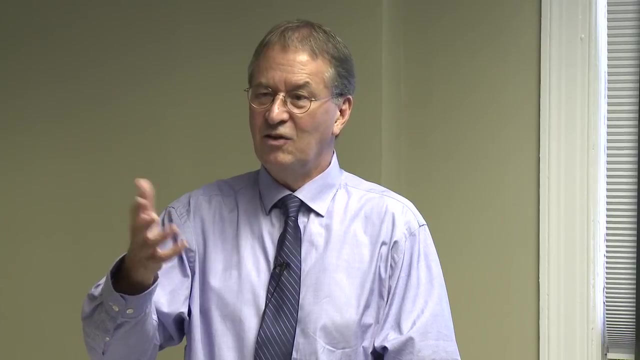 But they were also not sure, with their standards, that they could build an implosion-type weapon that would satisfy all the criteria of safety that were necessary to have an implosion system Because, again, it's high explosive, It can go off accidentally And then you could in some disaster.